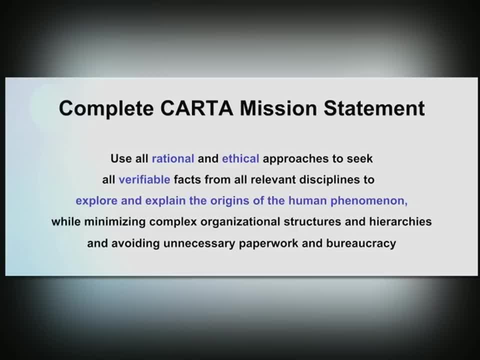 approaches to seek all verifiable facts from all relevant disciplines to explore and explain the origins of the human phenomenon. An important caveat here is, while we minimize the complex organizational structures and hierarchies that often infest these kinds of organizations and avoid any unnecessary paperwork and bureaucracy, the hope is to get to the science and get the discussions. 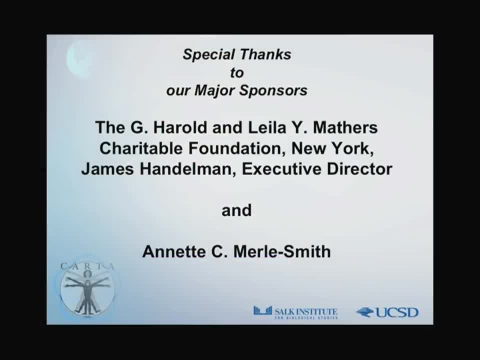 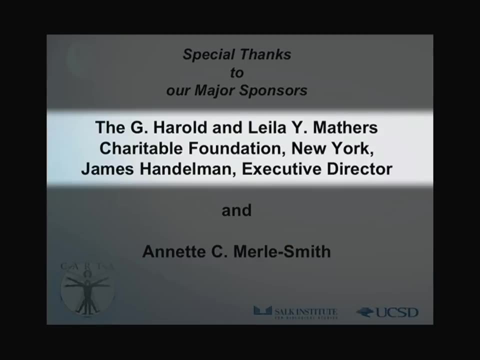 out front. This would not be possible without our major sponsors, who've, with great foresight, sponsored this organization, the graduate program that surrounds it, as well as these conferences, And the first one I'm going to talk about is the University of Michigan. 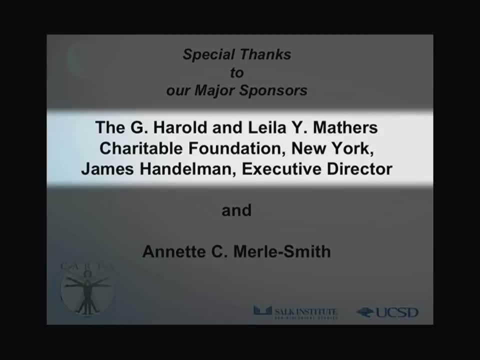 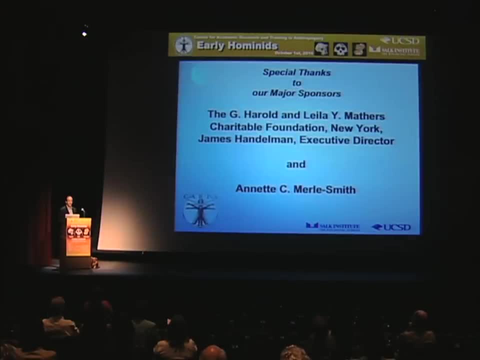 The second one is the G Harold and Leah Mathers Charitable Foundation, based in New York, And, secondarily but not least, Annette Merrill-Smith is very much appreciated for her continued support of this effort. These individuals are foresighted and extremely important for us. 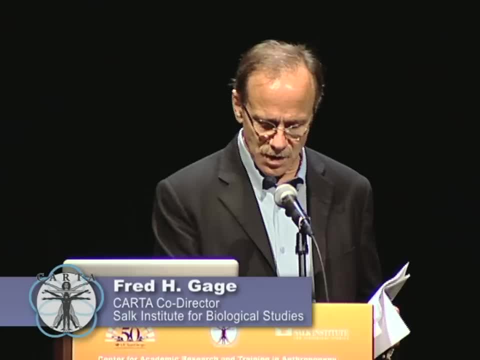 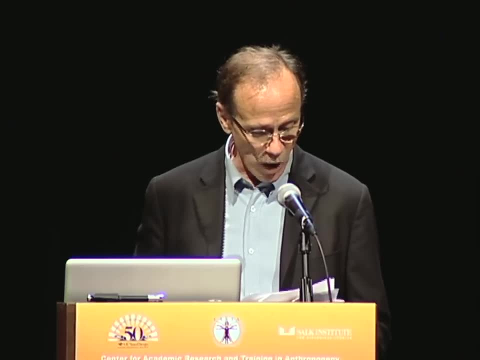 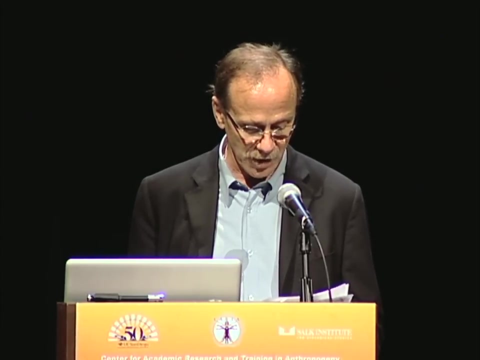 So with that, I'd like to introduce the chair of this symposium and the person that's really made the insight, And that's Tim White. He's currently the director of the Human Evolution Research Center and professor of Integrative Biology and the curator of the Biological Anthropology at the Hearst Museum of Anthropology. 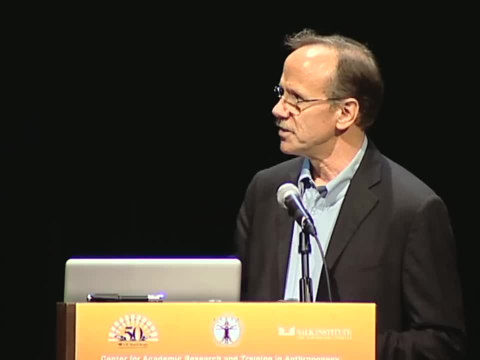 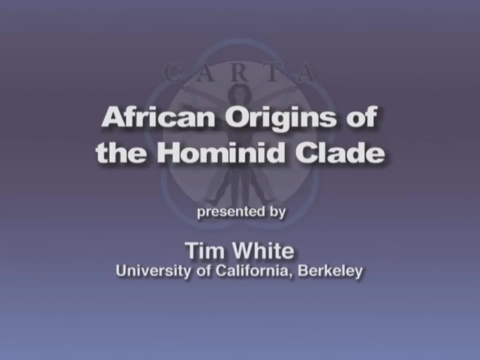 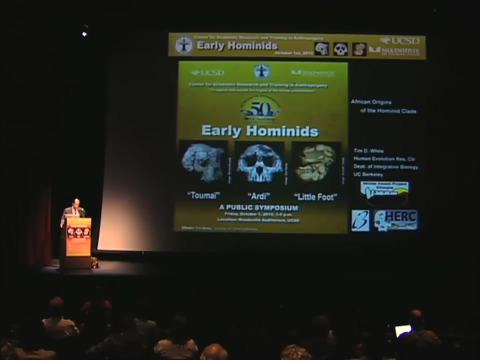 at the University of Berkeley, And I'll leave it at that and welcome Tim as the director of this symposium. I want to thank everybody for coming. Thank you This afternoon. I can guarantee you of one thing: There has never been a symposium like this. 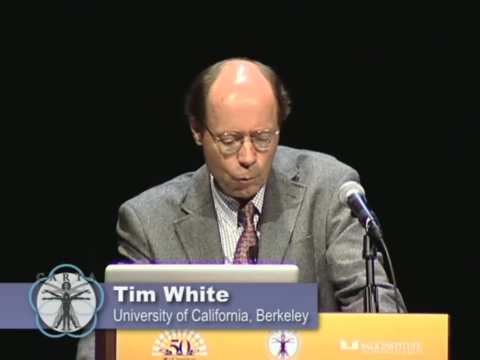 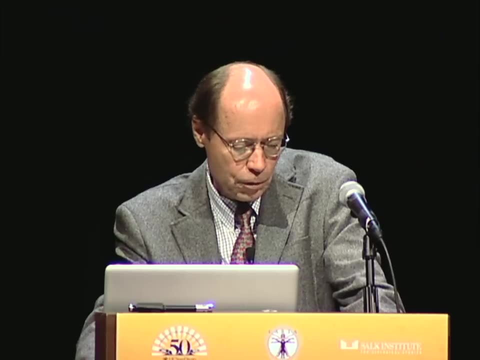 And it's exceedingly unlikely that there will ever be another one. So it's very unique And for this opportunity I would like to thank, on behalf of all the speakers today, the organizers. give you a little bit of history on this particular symposium. 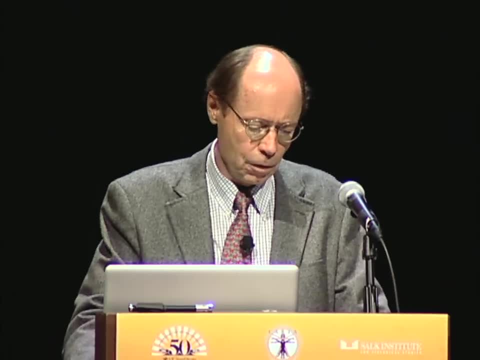 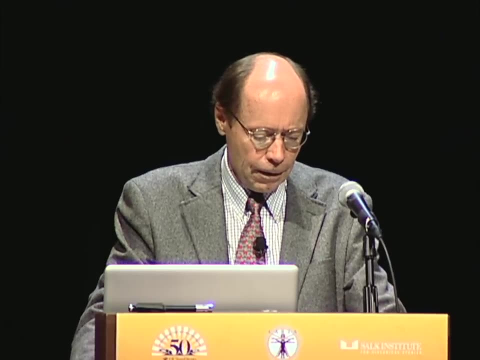 When CARTA was found in the early days, Dr Varkey called me And said: you know, we really ought to have a symposium on earliest hominids. And I remember at the time saying: you know, it's really not a good time for that. 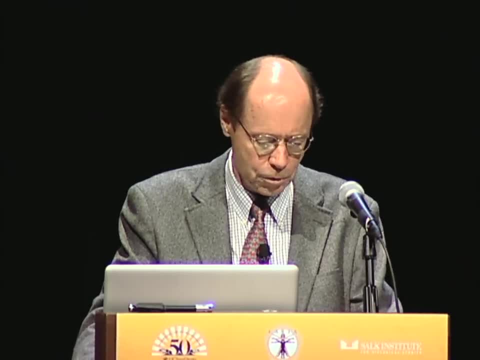 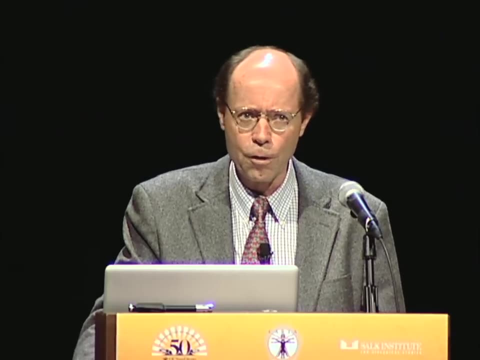 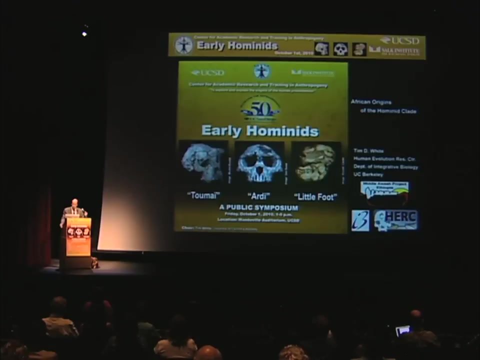 And for me it's often not a good time this time of year because we do fieldwork this time of year in Africa. But it was also not a good time because we didn't have enough early hominids when CARTA began And fortunately we now have enough. so when Ajit, who's very, very persistent called, 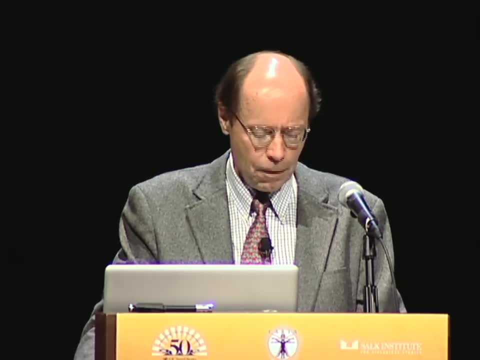 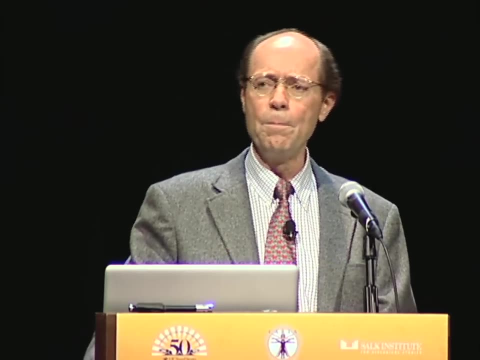 me last January. Thank you, January. he said: okay, now I have another idea. Why don't you chair a symposium that's all about all aspects of human bipedality? And I said, well, no, because I don't do that. 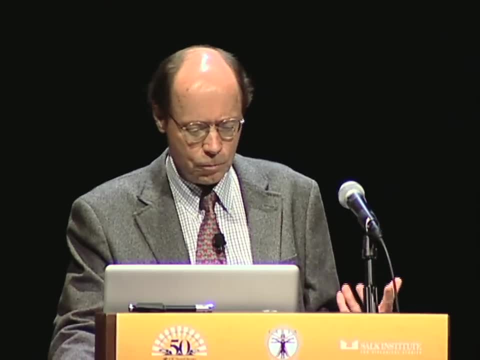 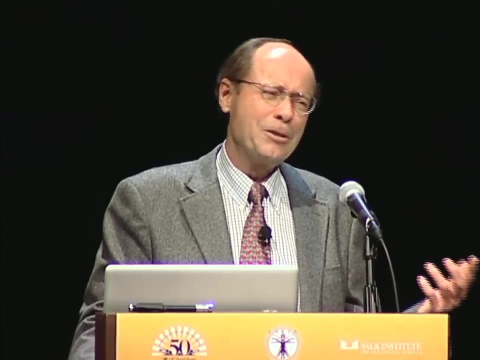 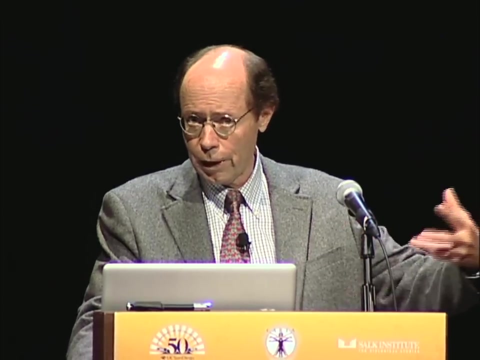 kind of research. I have colleagues who do those kinds of things, and sometimes I'm not a very good biped either. so why don't we think about this? It might be time to have this earliest hominids symposium, because we knew that within the next year a lot of 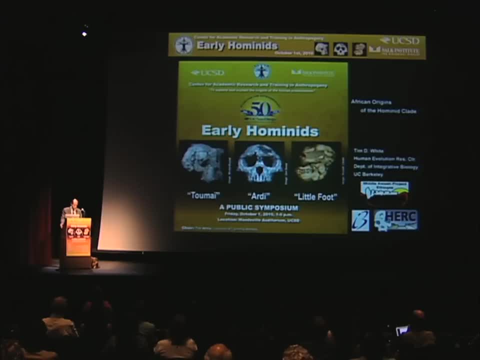 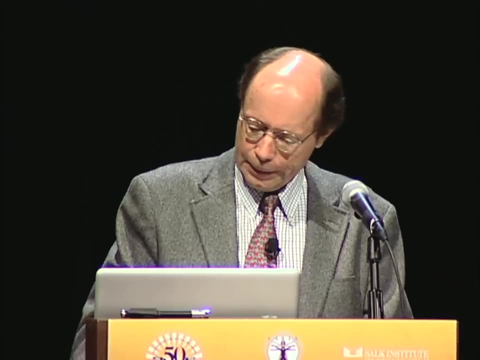 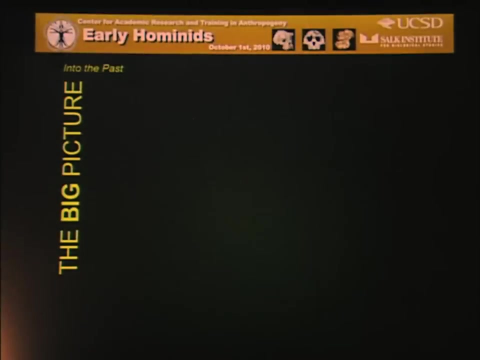 new things were going to be published. So by May of 2009,, the symposium evolved into what you will experience this afternoon. So let's get started. My part of this is to introduce the symposium, and I want to start with the big picture and move into the past. The first: 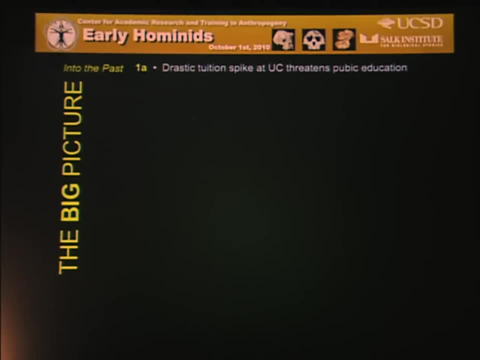 thing I want to do is not go very broad. I want to start with the big picture. I want to start with the big picture. I want to start with the big picture. I want to start with deeply into the past, One year ago- we can still remember this- a drastic tuition spike. 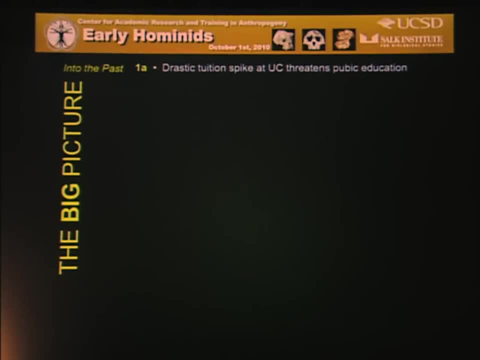 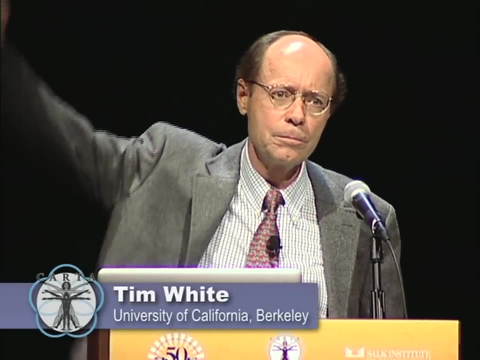 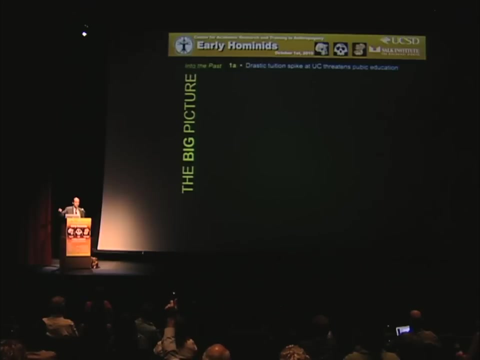 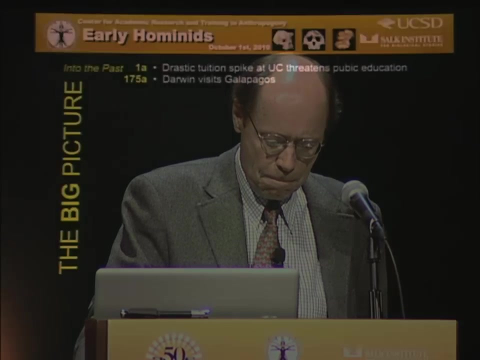 at the University of California threatens public education here. How many students and faculty were outraged by these tuition increases? I'm a faculty member. How many of you were not outraged by these tuition increases? Thanks for being honest. A hundred and seventy-five years ago, Charles Darwin visited the Galapagos. He arrived at 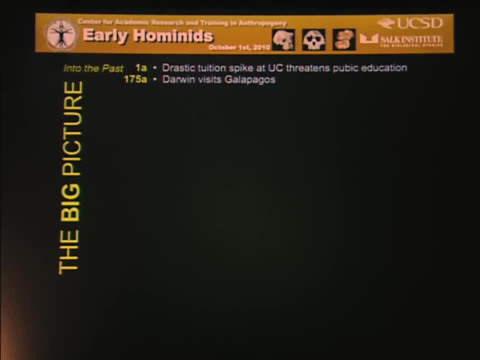 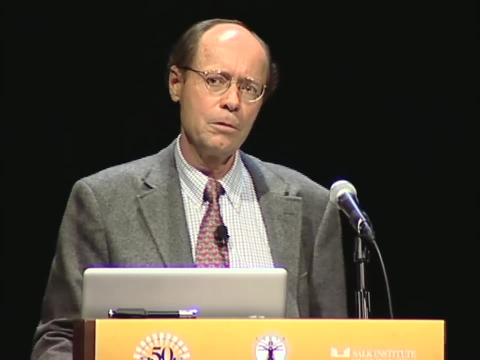 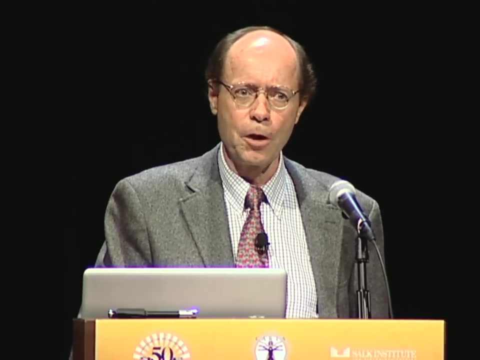 the Galapagos as a creationist and he left the Galapagos as a creationist. He went on to develop his ideas about evolution by natural selection. He went on to develop his historical perspective, But of course, when he visited the Galapagos he'd just come from the New 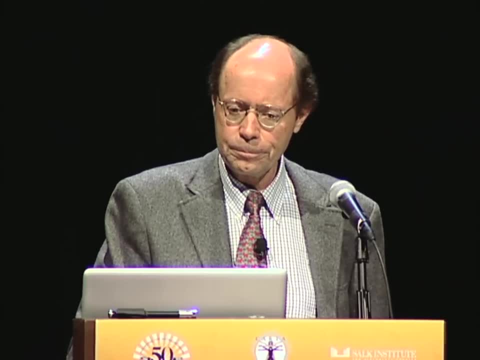 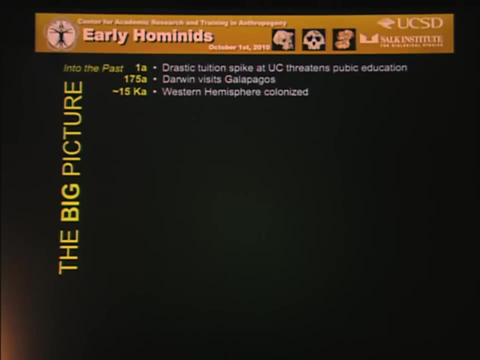 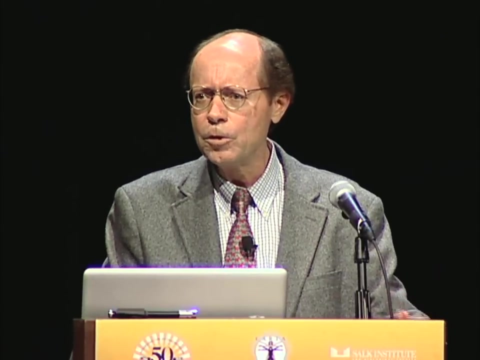 World from South America And this hemisphere. the Galapagos is a place where you can see the Galapagos And this hemisphere. it turns out Darwin couldn't have known it in his time- has only been occupied for about 15,000 years, And there's an amazing part of this. 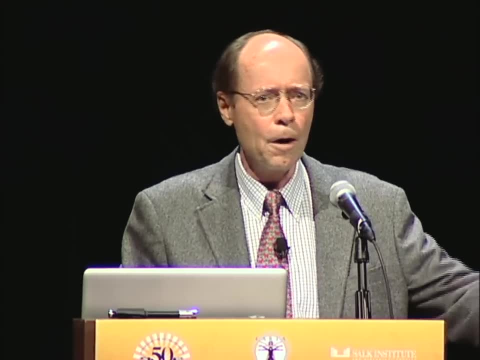 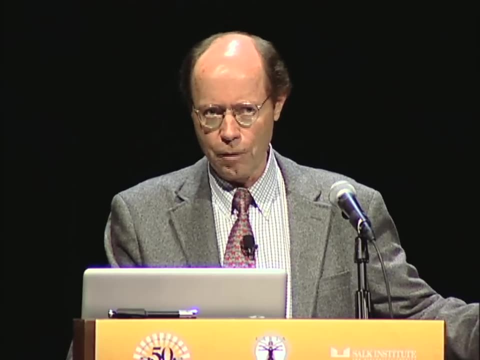 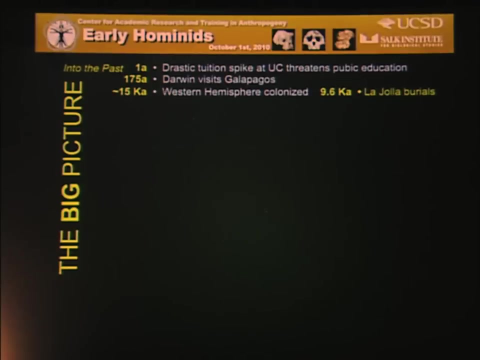 story which is actually local. Right here in La Jolla, right under the Chancellor's residence, in the 1970s, two human skeletons were excavated. These are the La Jolla burials. They're about 9,600 years old. 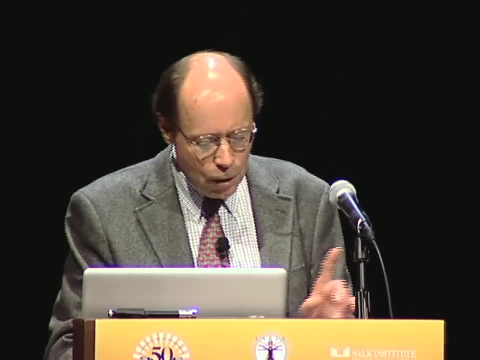 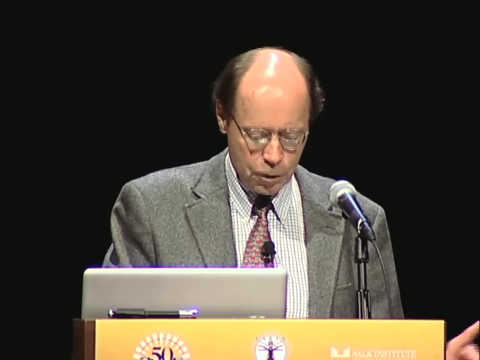 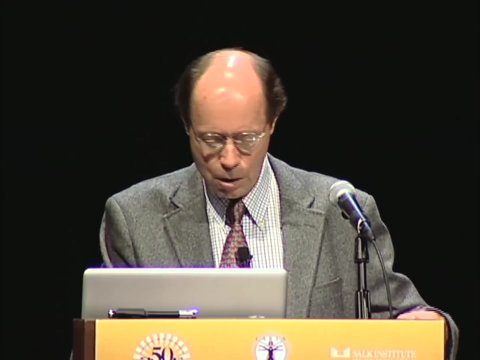 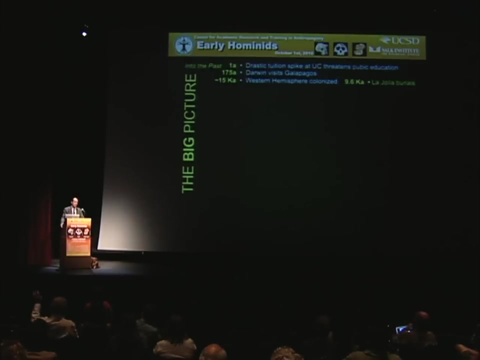 Very, very important evidence. How many of you would be outraged to learn that your Chancellor Fox at UCSD tried to dispossess our university because we're all from the same university of these remains? How many people would be outraged by that? Not as many, I don't understand. 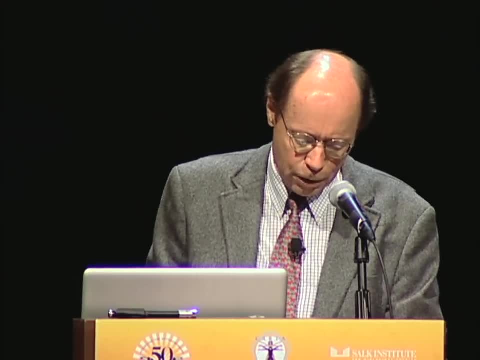 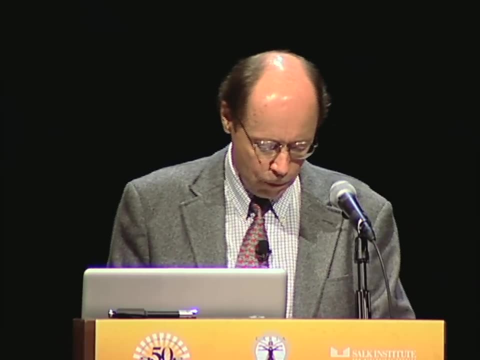 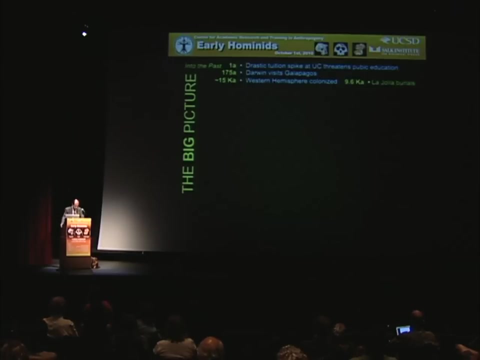 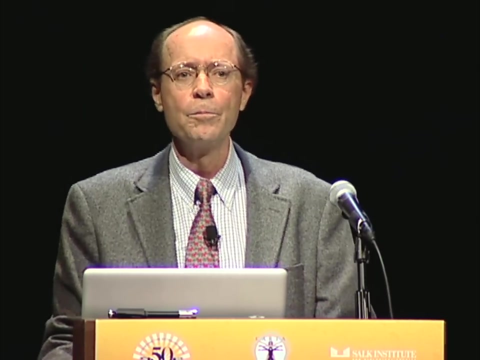 why not? How many of you would be outraged to learn that she wanted to do this due to the complaints of a small but vocal and wealthy group of creationists? How many of you would be outraged that the UC San Diego administration is preventing qualified researchers currently from studying that evidence? Yeah, I find it outrageous too. All right. 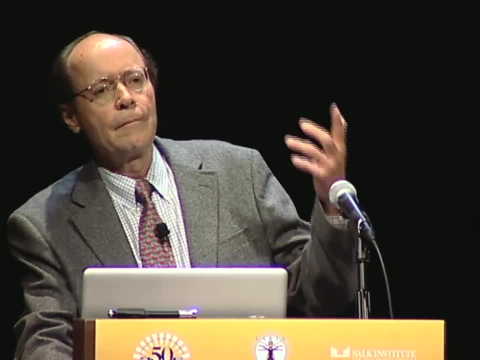 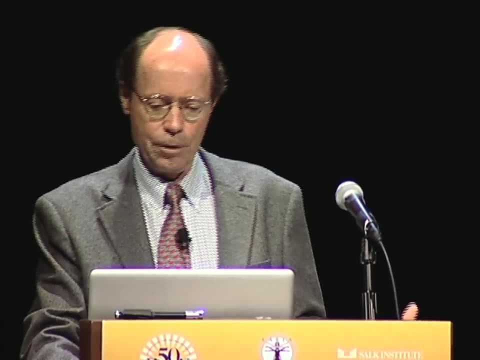 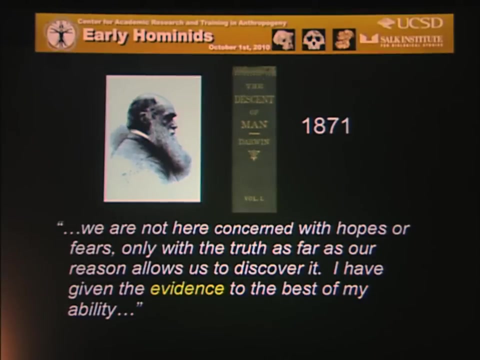 that's the controversial part of my talk. What's not controversial is that when you try to study the human condition and human evolution, you need evidence. Darwin said we're not here concerned with hopes or fears, Only the truth, as far as our reason allows us to discover it. I have given the evidence. 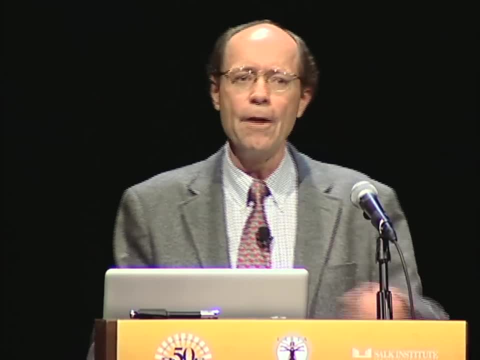 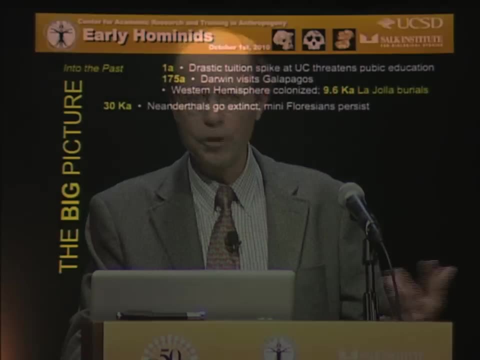 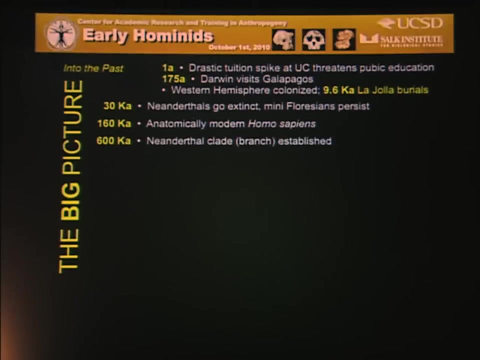 to the best of my ability, 1871.. Darwin had almost no fossil evidence at the time. Today we know that Neanderthals went extinct around 30,000 years ago. That's the first thing we know ago. Our own species appears in Africa at 160,000 years ago, About a half a million years ago. those 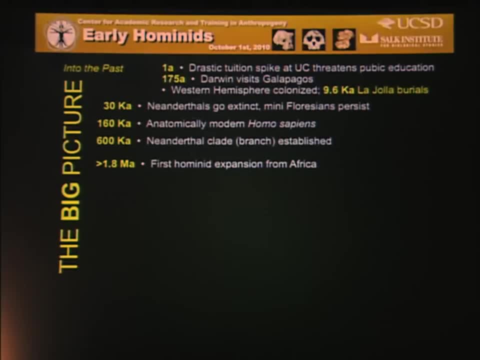 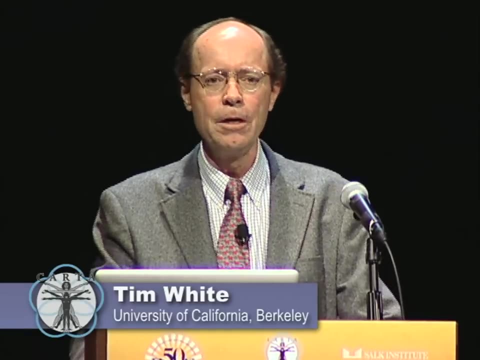 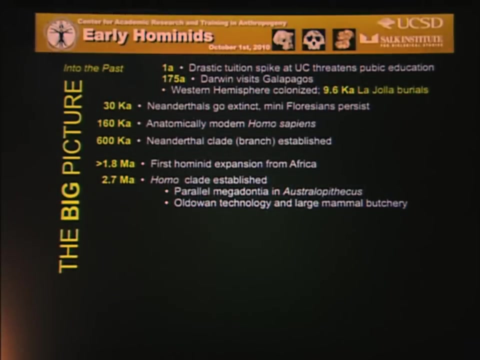 Neanderthals became a separate branch or a clade. We today know that there weren't any hominids anywhere except Africa until after around two million years ago. We know that in Africa, our own branch, what we call Homo evolved Stone tools began to be used about 2.7 million years ago. 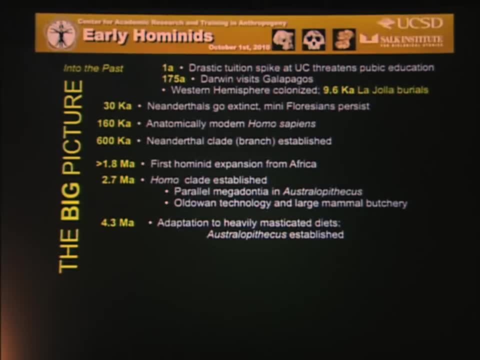 There's another, even earlier genus, known as Australopithecus, that originates around 4.3.. We know that we shared a last common ancestor with chimpanzees more than six million years ago, and we know that this is the segment of human evolution that today's symposium is about. 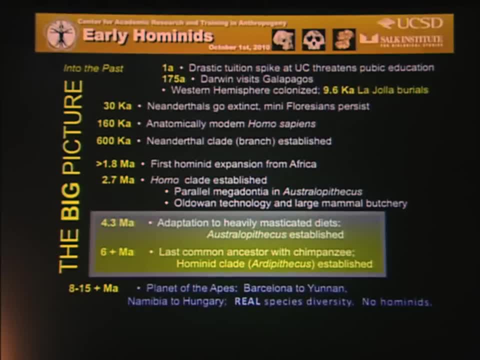 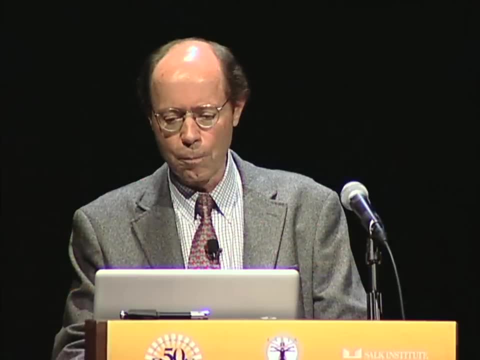 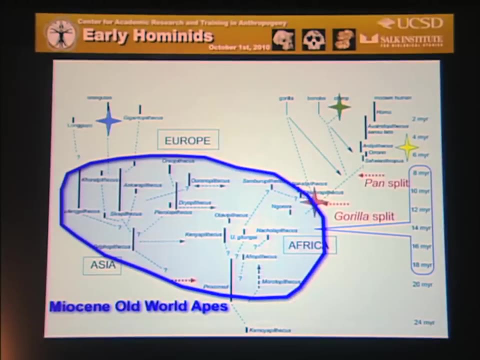 But we have even more more evidence from what we might think of as a planet of the apes, at least an old world of the apes, because from Barcelona to Yunnan, from Namibia to Hungary, there's real species diversity right there in the Miocene, between 8 and 18 million years ago. 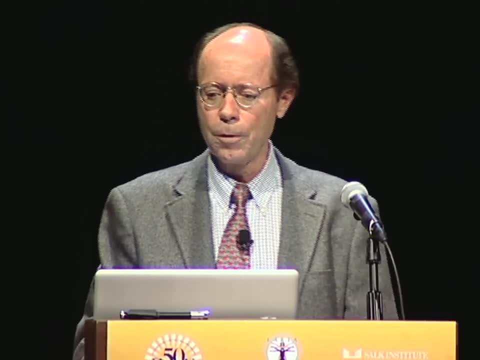 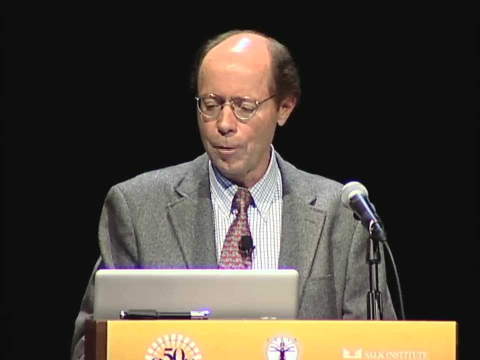 But we're not going to talk about those today. It'd be a great topic of a different symposium. Today we're going to talk about this part of the primate family tree, our part, hominids. Now, it being so, 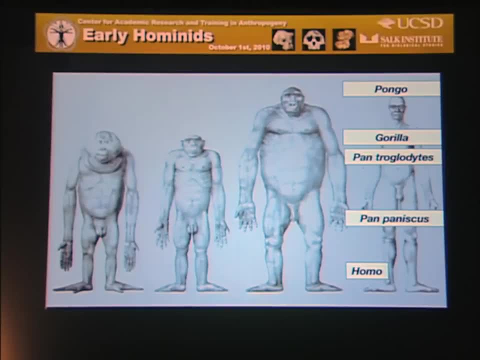 in San Diego, I have the great advantage of not having to take the time to explain what each one of these primates is. You all know that What we didn't know for a very long time is exactly what the genetic relationships were among these primates. 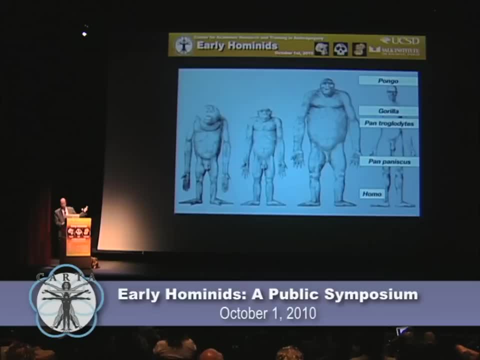 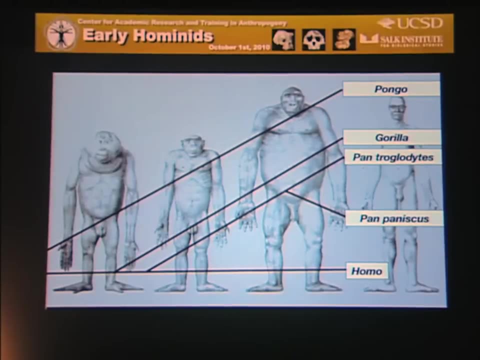 And it was due, starting in the 1960s and continuing all the way up until the modern genomic sequencing. we have now learned what our relationship is. We know that today the living species is the most closely related to ourselves And we know that the most closely related to 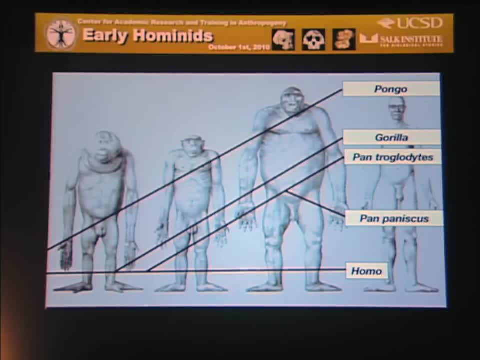 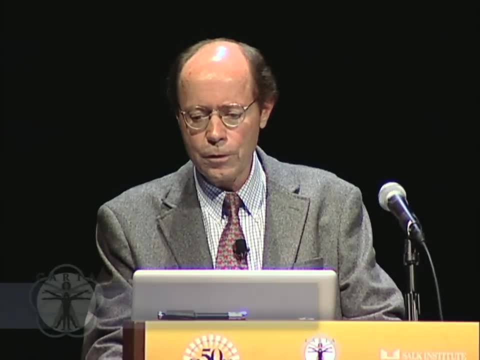 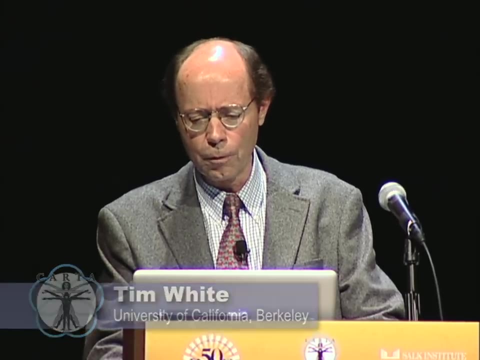 ourselves are the two species of chimpanzees And they're very closely related to each other. They only split about 2 million years ago. Unfortunately for the apes we don't have very good fossil records. But all of these fossils down here along our lineage and a couple off our 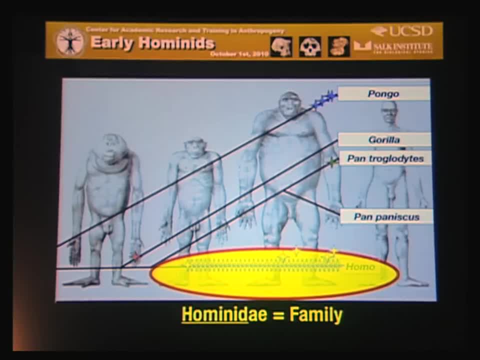 lineage but closely related to us, are placed in the family hominidae, And when I use the term mean- and most of the speakers in this symposium will use that name- and that's what we mean when we say hominid. So that's our real focus And our focus really is on the earlier. 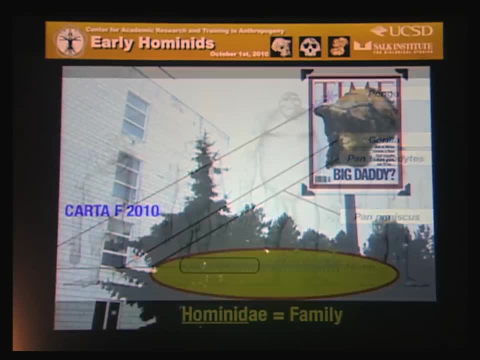 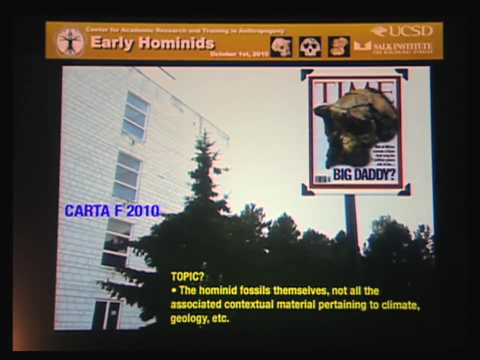 part of this branch or this clade of the family tree. So we thought about: okay, who are we going to invite for speakers at CARTA? Who are you going to invite? Well, first let's set the topic. The topic here we decided was going to be about the hominids themselves. If we go too broadly, 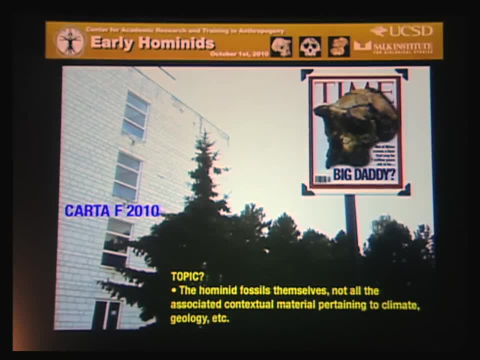 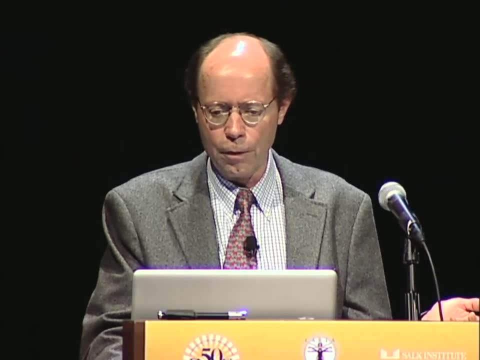 we'd be here all week to talk about the context, the environment, climate, geology and so forth, focusing in on the hominids. So who are you going to call? Who are you going to invite? Well, somebody, maybe, who found the oldest hominid fossils And you want. 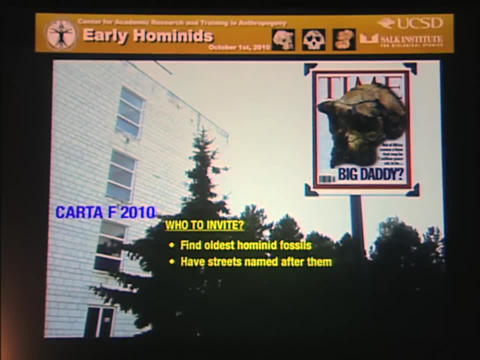 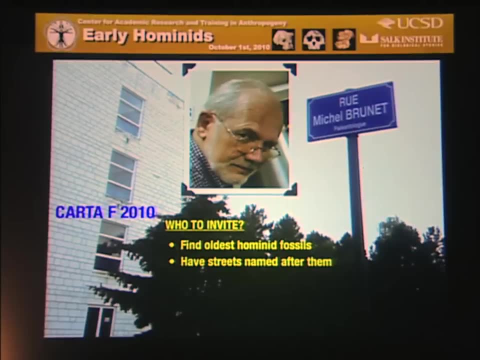 people that are recognized globally for having found the earliest, you know, people that have streets named after them. For example, you would want Michel Brunet, who found the oldest hominid fossil and has a street named after him. So okay, we've got one speaker lined up. What do we do? 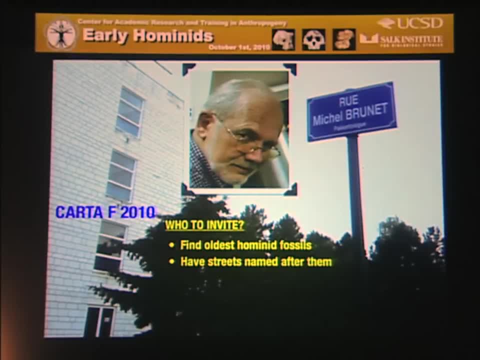 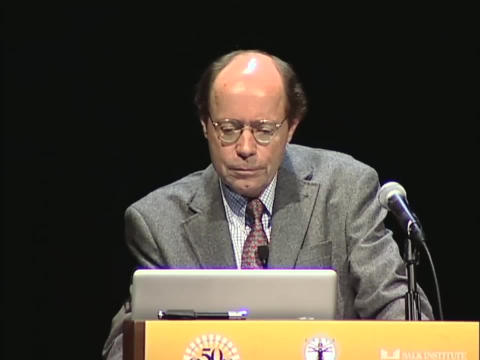 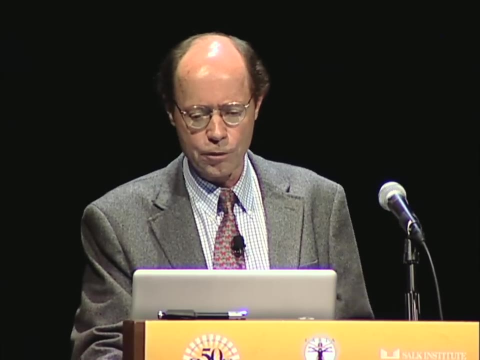 next, Who else has a street named after him? Well, we're going to have to do a little bit of digging, So we had to dip more deeply into the barrel. People who actually lead field research, recover and analyze fossils, people who are still finding fossils- And these people will. 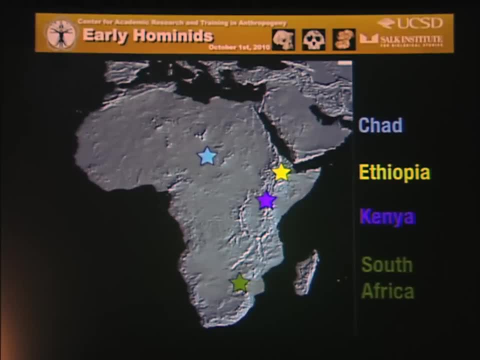 talk about the fossils they are actively finding in places like Chad, Ethiopia, Kenya and South Africa. I work, and some of my colleagues work, in this part of the world, and I'm going to talk about the fossils that we're actively finding in places like Chad, Ethiopia, Kenya and South Africa. 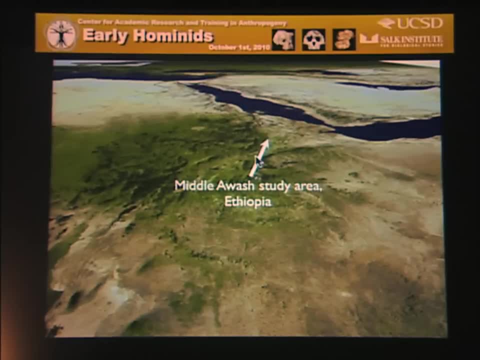 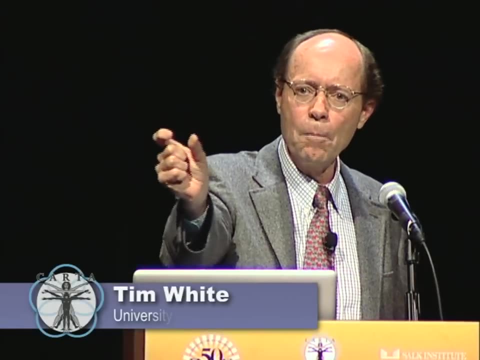 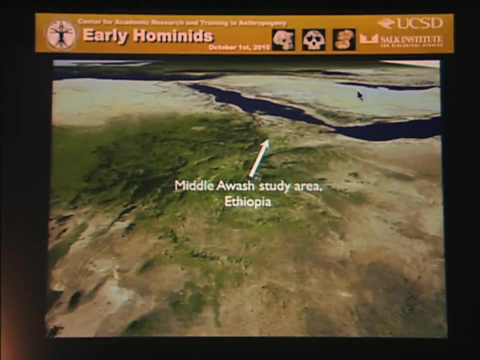 of Ethiopia. It's a lowland depression formed as the Arabian Peninsula rotates away from Africa at a rate of about that much a year, about 17 millimeters, And that's fast in geological terms. So what that means is this valley has been opening up over time due to these tectonic 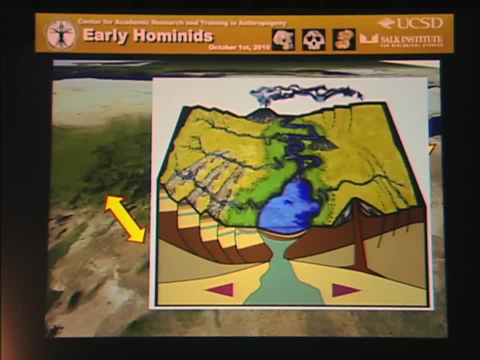 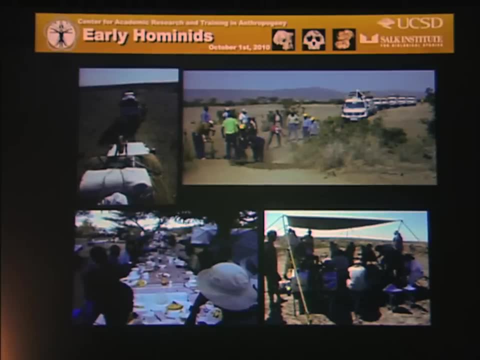 movements, And we have all the ingredients here, in these rift valleys for fossilization of previous life forms. We have the lakes, the sedimentation, the volcanics that can date them, And you'll learn more about this. We go to the field every year. 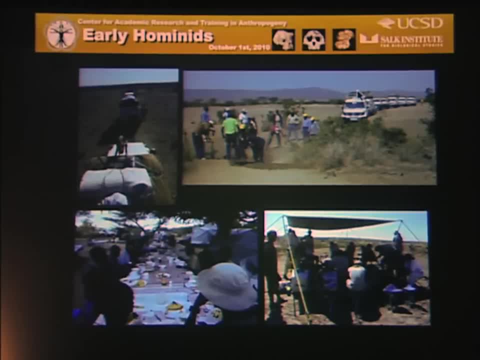 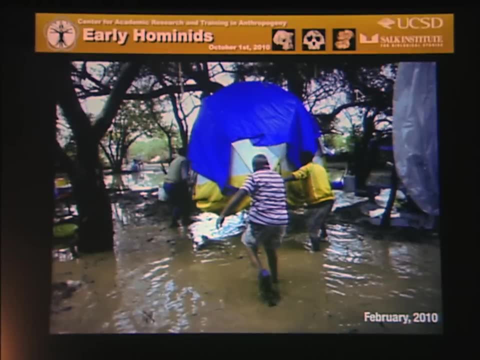 It's a very remote area in the Afar of Ethiopia. This is the field team And occasionally we don't get out of the field before it rains. This was last February. after heavy rains And all of the water from the highlands comes down in ponds And when it dries up you have a little. 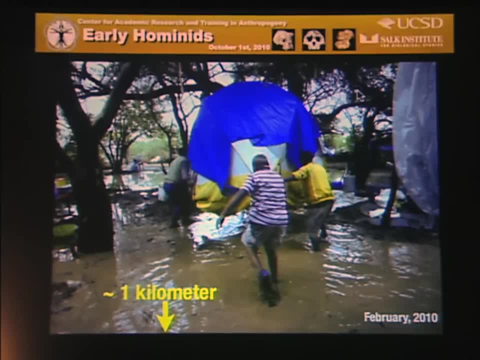 layer of sediment right at the top, Last year's flood sediment. This has been going on for millions of years, So under our feet we have approximately a kilometer of accumulated rocks. So we're going to look down into that kilometer to the bottom half of it. 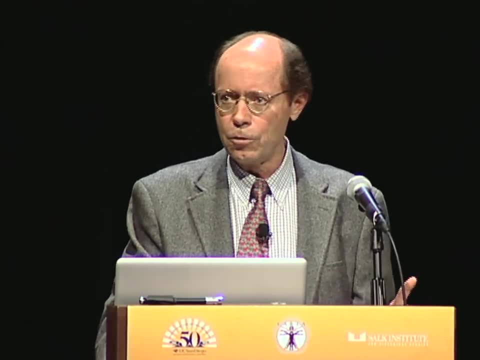 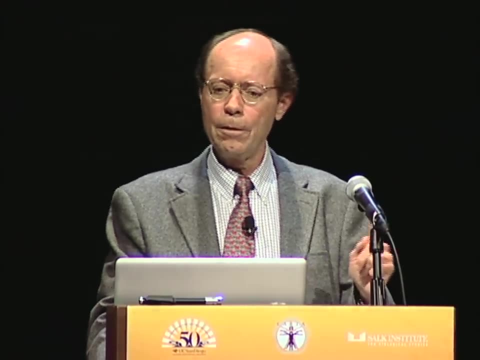 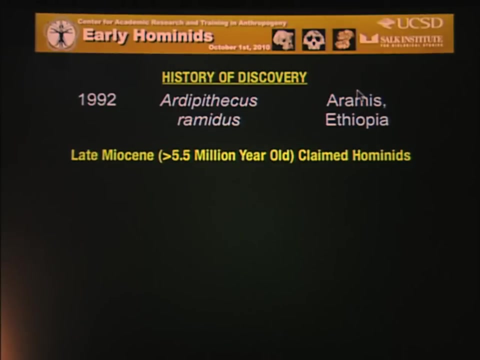 in the middle Awash Valley Beginning in 1992, Gensua, one of our speakers, found the first fossil from a horizon of 4.4 million years ago. We named it Ardipithecus ramidus. It's from Aramis, Ethiopia, But what happens if you go further down in the rock record? 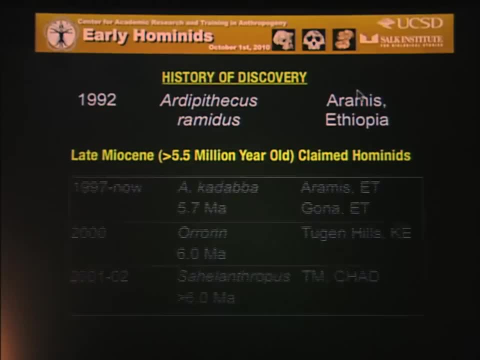 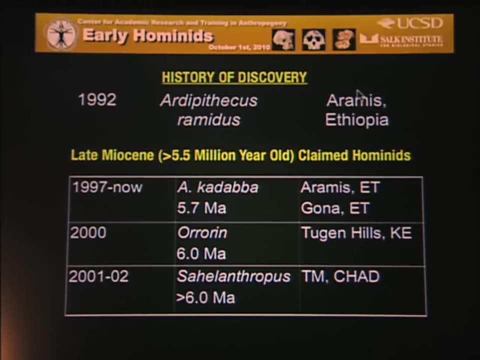 6 million years ago. Well, it proves to be difficult to find these older hominids. Here's a chart of all of them. We'll be talking about them today. in the symposium Starting in 1997, another of our speakers, Yohannes Haile Selassie, found the first. 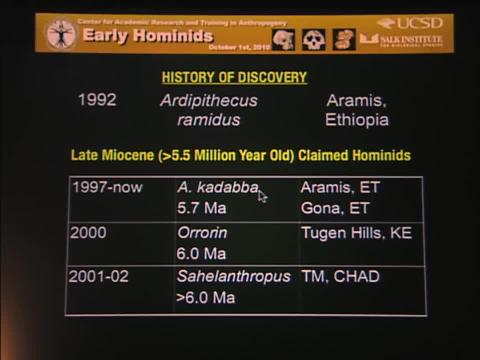 lower jaw of this thing called Ardipithecus kadaba. Shortly thereafter in Kenya, something called Auroran was found. Andrew Hill, one of our speakers, will be talking about this- And Michel Brunet found this thing in Chad. 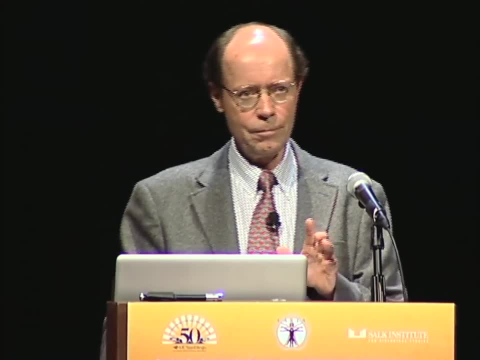 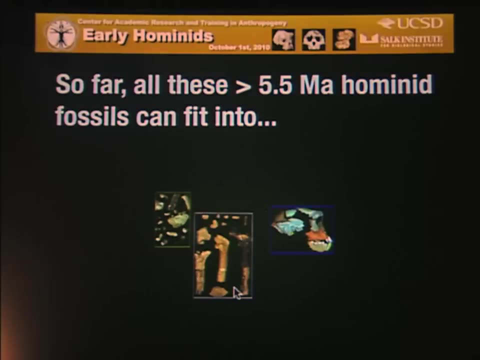 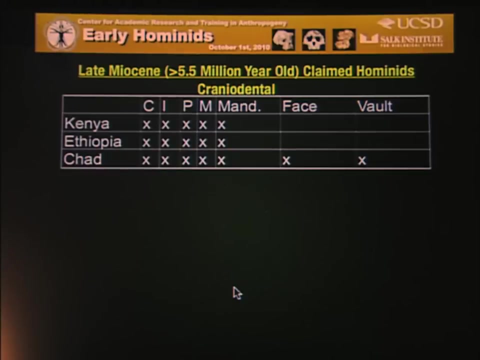 Now disclosure. The total combined remains from these very early rocks late Miocene –, we call them in age – can fit into two shoeboxes When we plot out what's actually been found. older than five and a half million years ago, we have canines, incisors, premolars and molars. 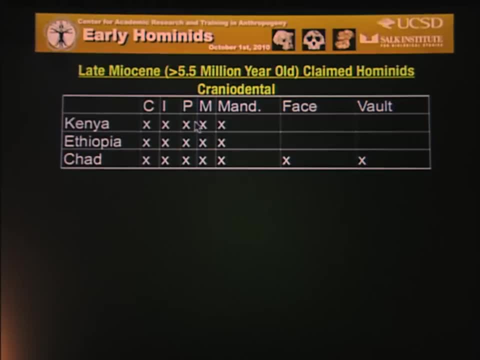 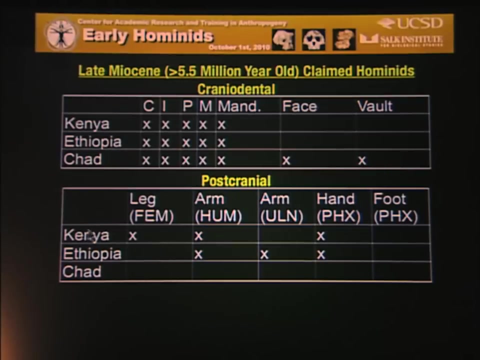 So we have dentition from all of these sites, We have lower jaws from all of the sites, But only one site has yielded the face and the vault that you saw on Time magazine. How have we done below the neck Even more poorly? A couple of leg bones from Kenya, No matching parts from Ethiopia and Chad. 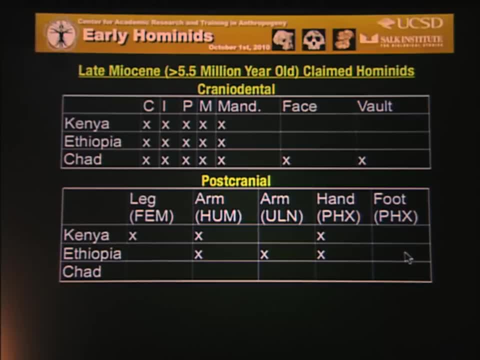 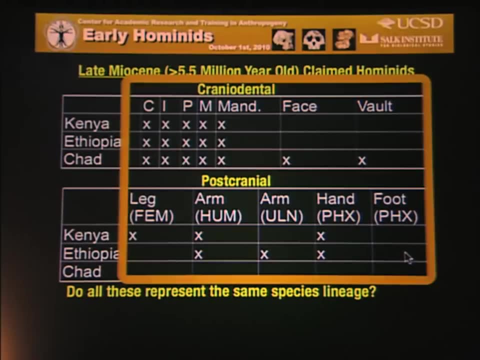 This is really pathetic. There's not even any toe bones. Like I say, fits in a shoebox. Do all these represent the same species lineage? Well, the answer can only be ascertained at this point based on that evidence, which is limited, And when you look at the 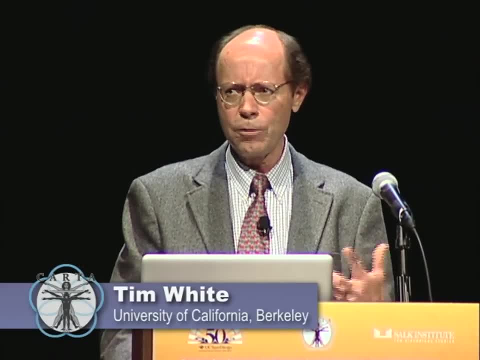 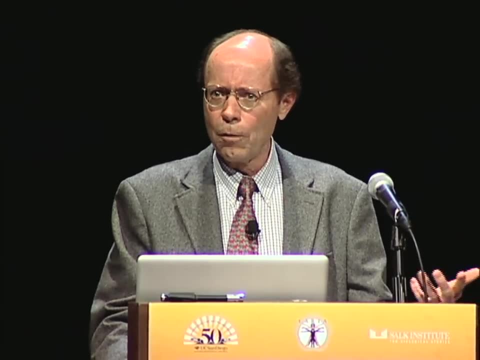 distribution of these traits. what you find is that there's not much variation there at all, Certainly not as much as there is between orangutans, gorillas, chimpanzees. It's really arguable whether there's even as much difference as there is between pygmy chimps and common chimps. 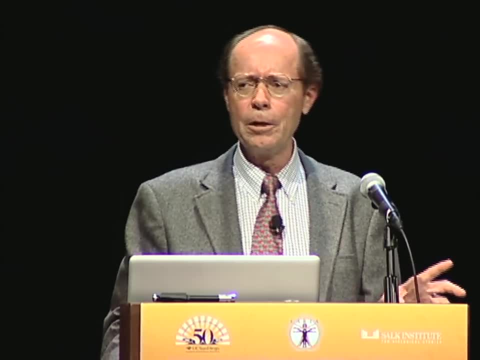 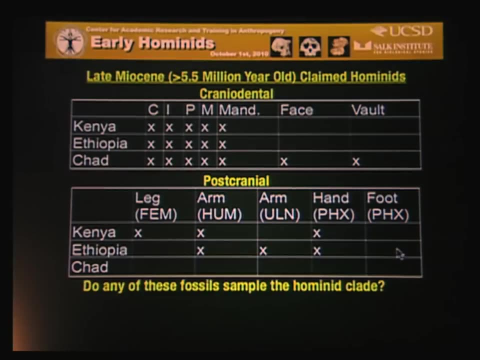 So answer: really too early to tell, but probably, at least, these things are in the same genus. Now, what about these? What else can we tell about the biology from these forms? Well, do any of these fossils sample the hominid clade? Are they more closely related to us than to any? 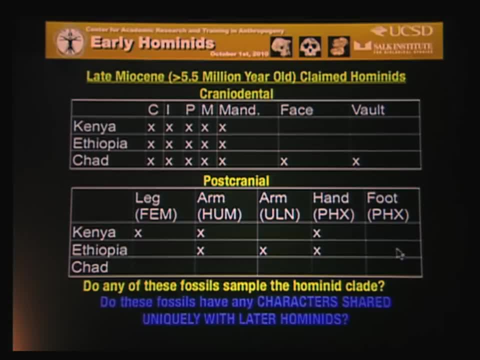 other organism. Another way to ask that question: do these fossils have any characters shared uniquely with later hominids such as Lucy? And the answer is yes, they do, Especially in the canines, in the premolars, the face and the vault and in the leg. 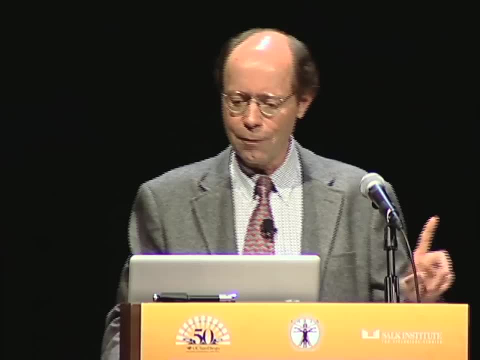 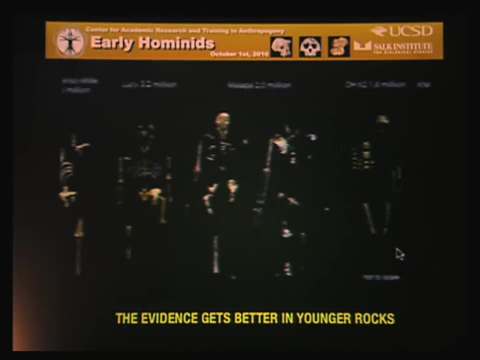 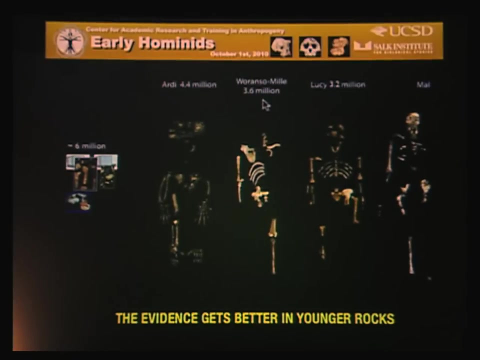 Fortunately for paleontology, the evidence gets better in younger rocks. So, for example, at one six million years ago, we have the Turkana boy. We have some South African skeletons. Here's Lucy from Ethiopia at 3.2 million years ago. Johannes has gone on to open his own site. He just 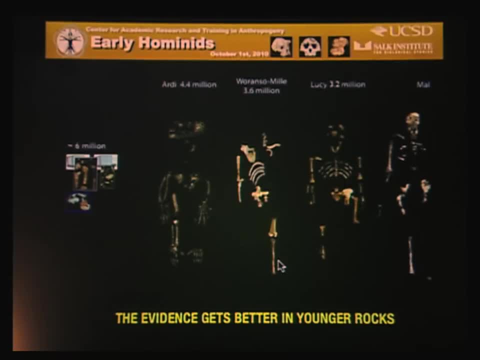 announced this skeleton in the Proceedings of the National Academy of Science And this one here at 4.4 million years ago. There's our shoe boxes over there. Sorry, that's all we can do. So we go to the best, earliest evidence, which is this skeleton. It's from the middle awash, It's from right here. 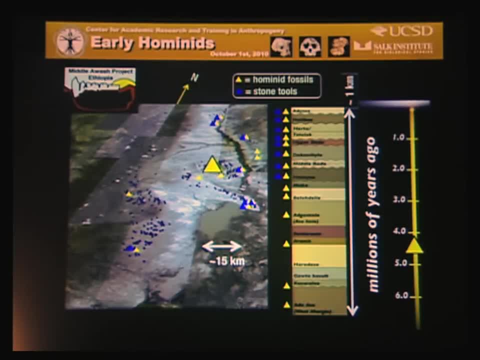 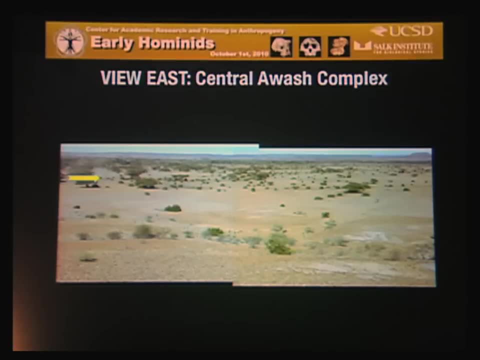 in the middle awash Space And right there in time, 4.4 million years ago, Much of a skeleton For scale. this is the landscape and that's a vehicle. Very, very large landscape. Very, very small fossils. 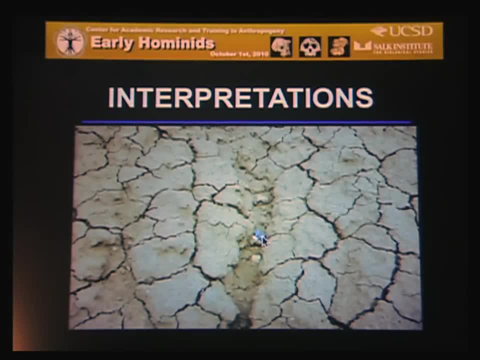 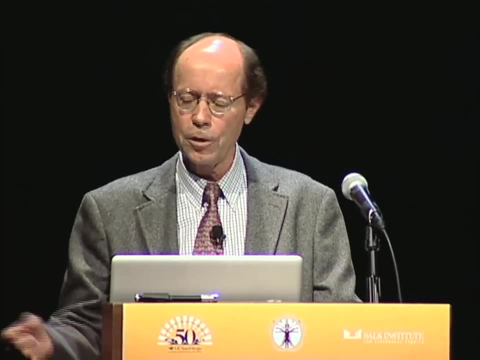 This is what they look like on the ground. That's about three quarters of an inch long. It's a tooth of something. It's a tooth of an antelope that's eroding out of floodplain sediments laying down 4.4 million years ago. Actually, it's a kudu. 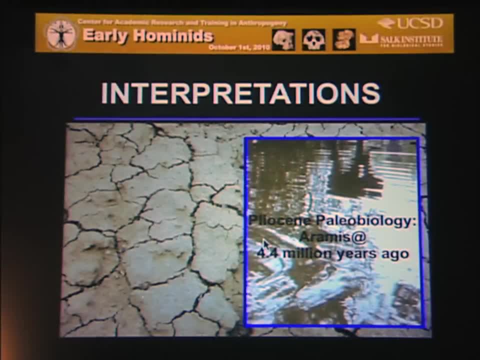 So when we go to the fossil record — we're not going to the fossil record just for the hominids, but for the entire paleobiology and geography of this place — we want to extract as much evidence as we can from this unique horizon. In order to do that, to extract the evidence and then to analyze, 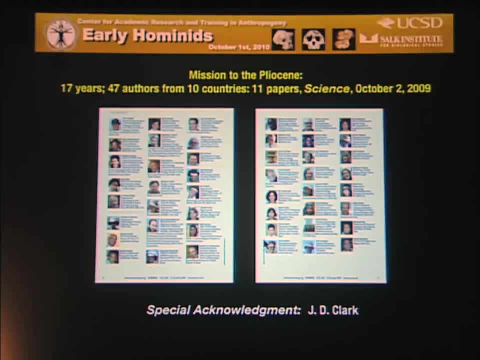 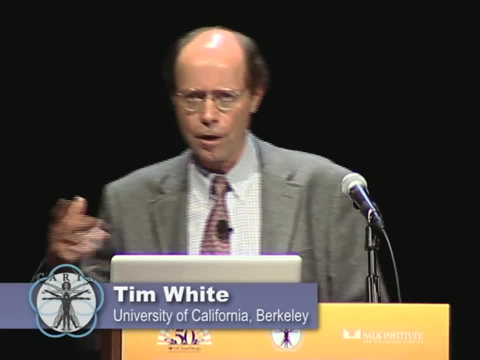 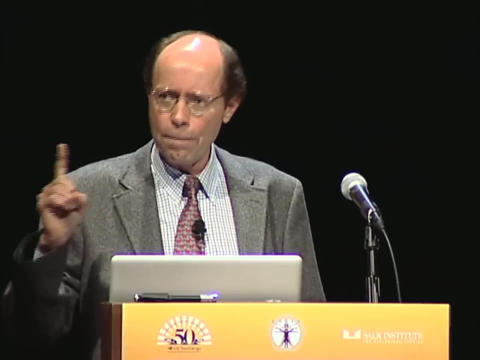 Now, an interesting thing happened along the way, Dad. People criticized us like crazy, Why aren't you publishing faster? We need to know the information. That was true all the way up to the day that we published in science The next day. what was the complaint? 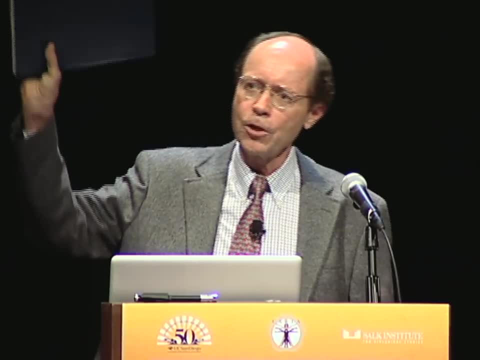 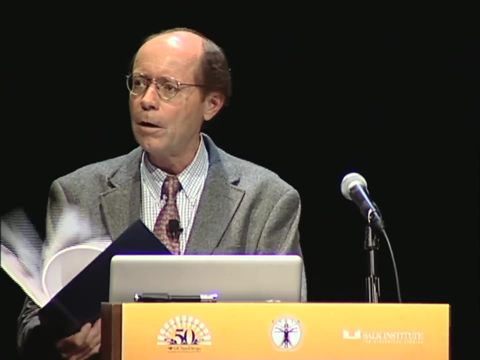 You've published too much. You see, we published about 600 pages on this primate, this Ardipithecus ramidus, from 4.4 million years ago, And it's all here and it's all available online. 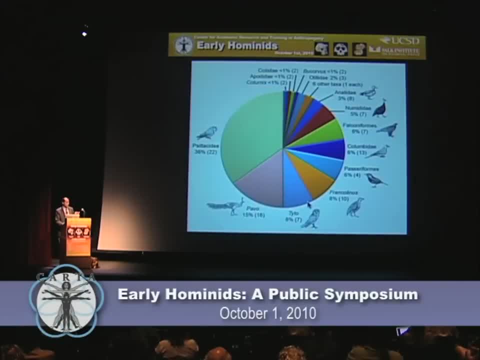 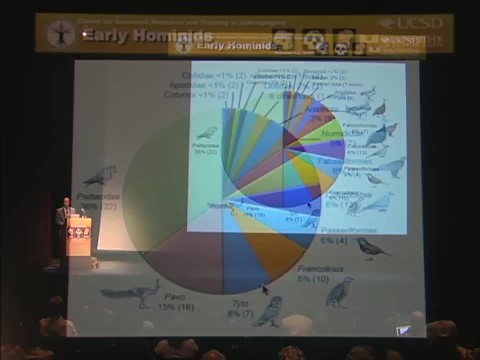 Well, so what? What does it tell us? Well, it tells us amazing detail about the world at 4.4 million years ago in this place. For instance, one of the experts on that picture- one of those authors- works on birds. 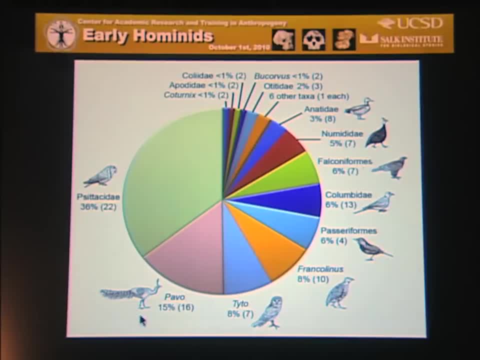 He's able to take a little bone from a bird and tell you it's a parrot or tell you it's a peacock, And it turns out that almost half of the birds from this place found with Ardipithecus are parrots and peacocks. 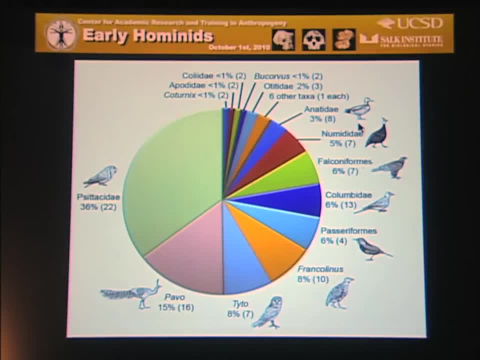 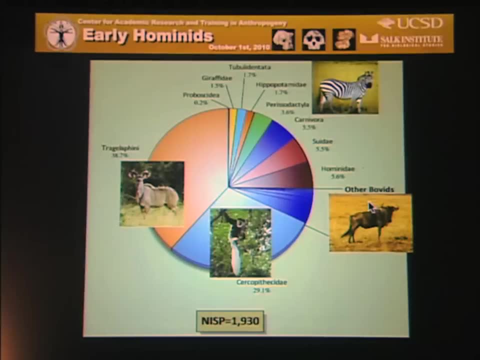 That's really unusual. Most of the sites are dominated by water birds like ducks, who die in water and get buried. Most of the other sites in Africa are dominated by these kinds of animals. They're antelope who eat grass in the grasslands, not by those kudus. 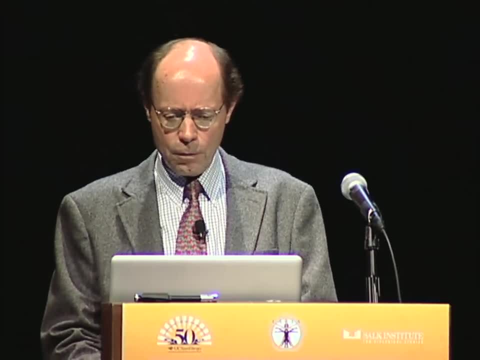 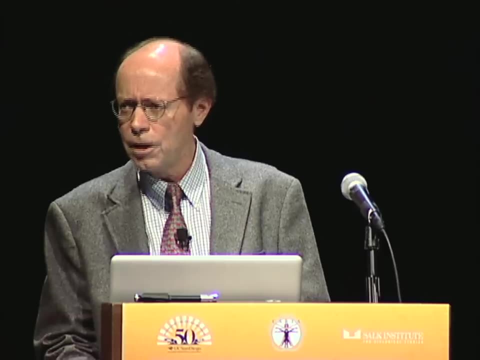 So we can look and we can say: gee, you know, that's interesting. Look how many primates there are. In addition to the hominids, there are all kinds of monkeys, And among the monkeys there are colobus monkeys, leaf-eating monkeys. 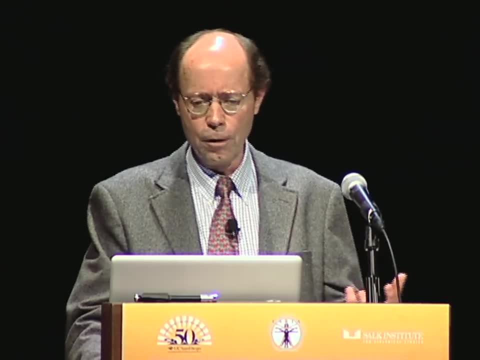 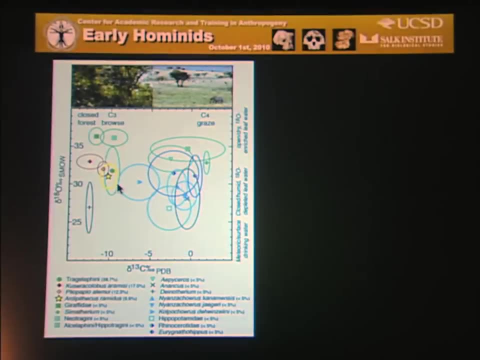 And we can do this with one group of animals after another: invertebrates, plants, mammals, all of these animals. We can even look at the other side. We can see that there are a number of isotopes in that dental enamel. 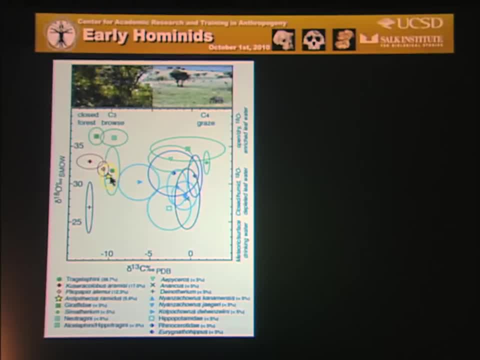 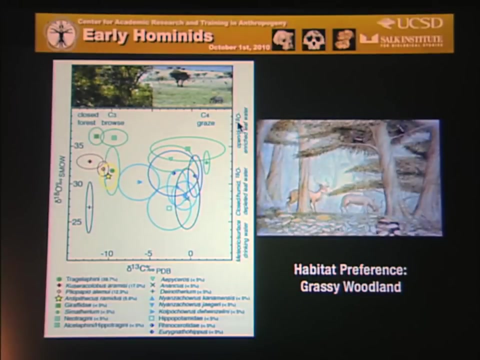 And we can plot out the kudus. Those are these antelope here. Here are the kudus And this yellow one right next to it. same isotopic composition, virtually, is Ardipithecus, And it's in this more closed fauna which is numerically abundant on the site relative to the more open grassland faunas. 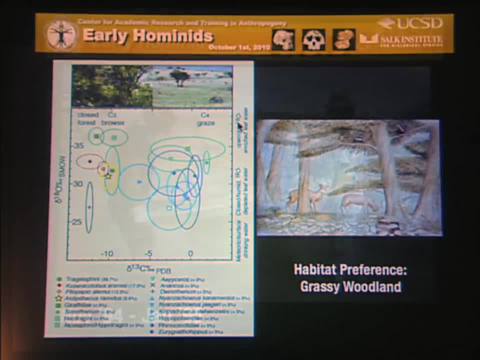 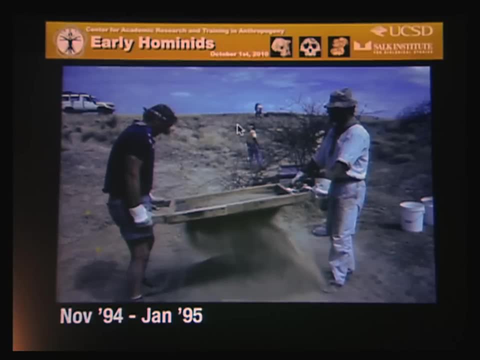 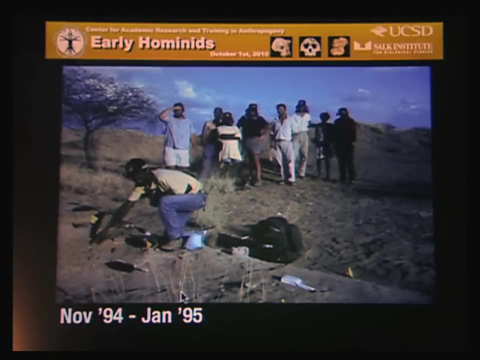 So we infer from this that the habitat preference was a grassy woodland. All right, Fine, I said I wasn't going to talk much about context. It's important in this case, though. In January 1994, this man right here, Johannes, was moving very slowly across this surface when he found a hominid bone. 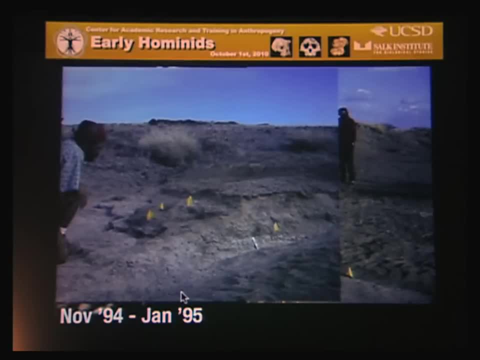 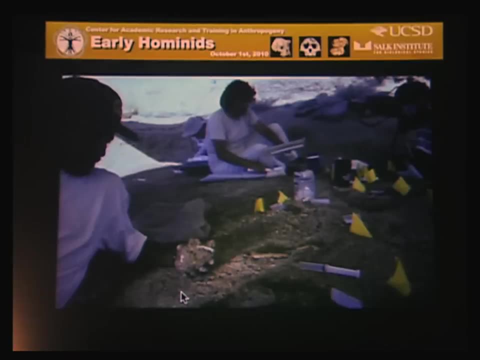 We excavated, We started to find more in place. We removed the top of that hill, And each one of these flags is a separate part of what turned out to be one hominid individual's skeleton. Here's Johannes with a piece of the hand in matrix. 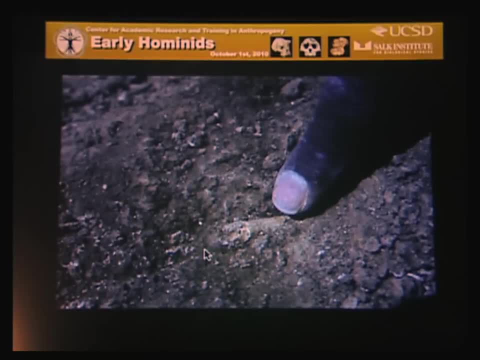 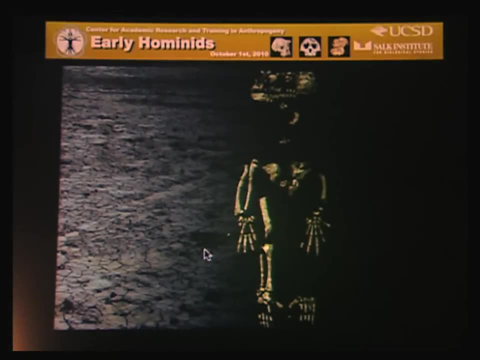 Here's a piece of the hand. This is from the palm of a primate who died here. This is from 4.4 million years ago. Slowly exposed and then removed, These bones were very fragile, very broken. But when we had them all extracted three years later and when we had them all cleaned of matrix another five years later, 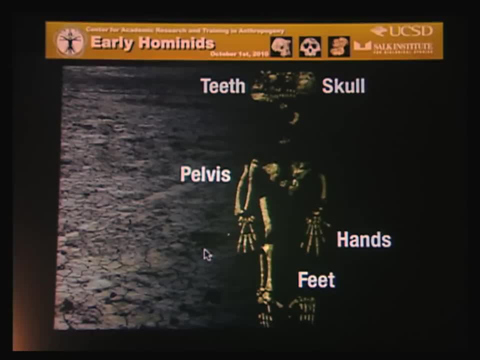 we could start the analysis of the teeth, the skull, the hands, the feet and the pelvis And we ended up with an individual. Only one individual was represented, But at the same time we were working in the same time horizon and we found 115 hominid specimens of other individuals. 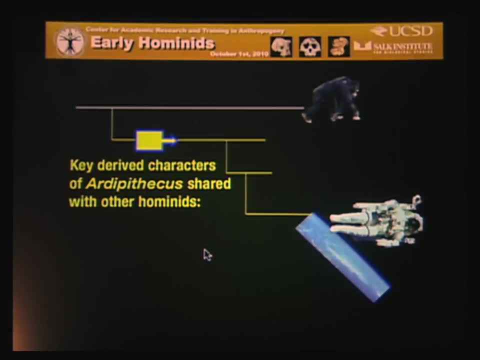 In studying this massive material for all this time, we're able to learn that this skeleton, the new one from Ethiopia, shared a lot of characters with later skeletons like Lucy, and indeed with our own skeleton. What are these characteristics? Well, the canine teeth are very feminized, even in the male individuals. 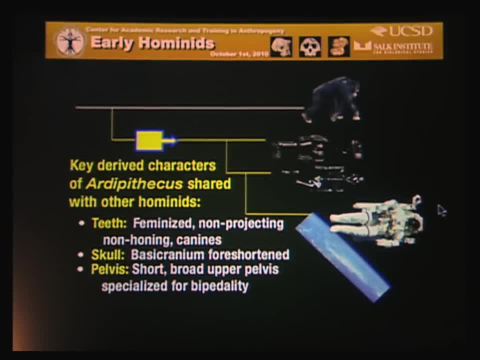 The skull is very short, The pelvis is short and broad in the upper part And the foot is very specialized On the side of the foot. Very interesting organism And since it's so close to the split with the apes, it also casts some light on chimpanzees. 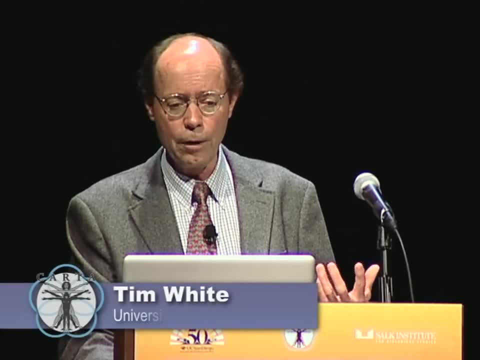 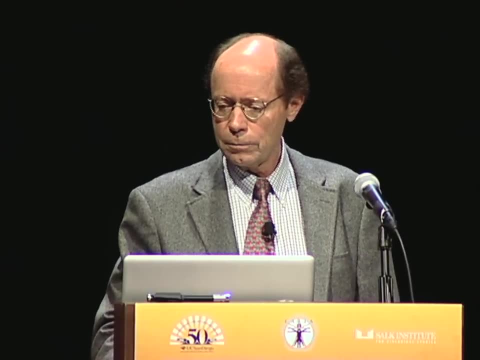 So now we can understand, because of this fossil record, that chimpanzees have been evolving at the same time that humans have. They've evolved these long bones in the palm of their hands. They're not short like the one we dug out of the ground. 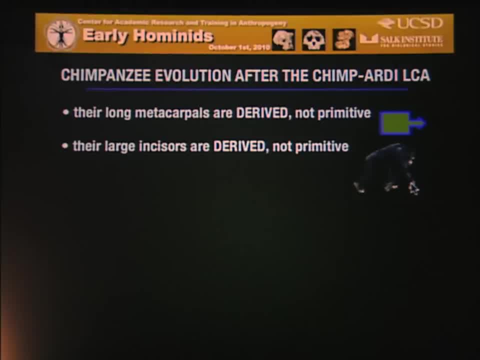 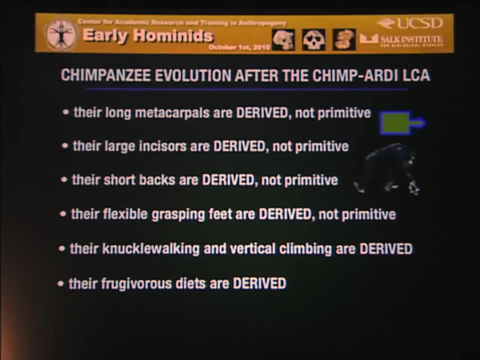 They're very long, They're elongate, They're knuckle walkers. Their huge incisors are highly evolved For their frugivorous diet. Their short backs, Their flexible grasping feet, Their knuckle walking, Their vertical climbing. 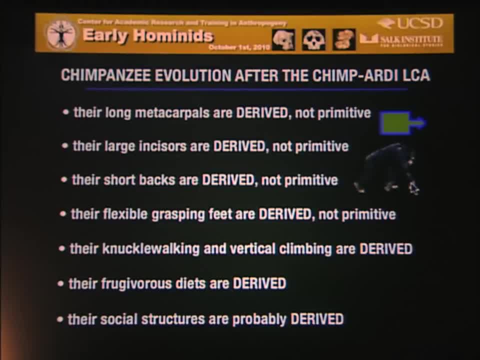 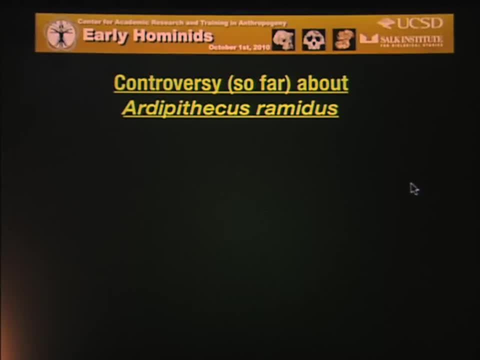 Their diets Indeed, their social structures are probably highly derived, All right, So we published this last October And the controversy so far has been about: did it really prefer a woodland habitat? Is it the ancestor of Australopithecus? 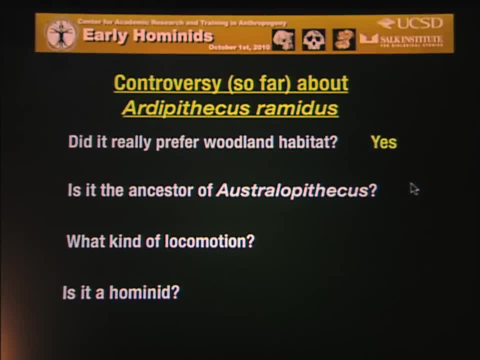 What kind of locomotion did it use And is it a hominid? The answer to the context is yes. You've seen some of the data. There's a lot more. Is it a hominid? Seems to be yes. 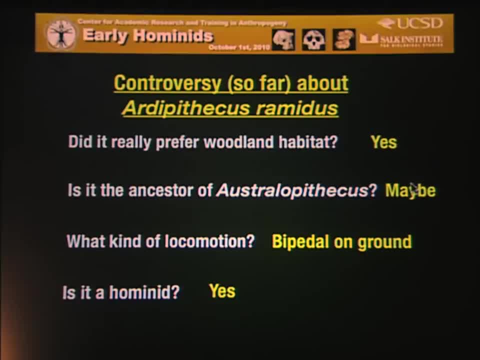 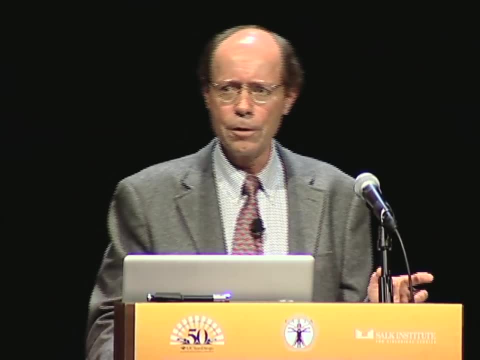 You'll hear more about that in the symposium- Seems to be bipedal on the ground And it may actually be the ancestor of later hominids, at least generically speaking. Let's look at why we would say these kinds of things. 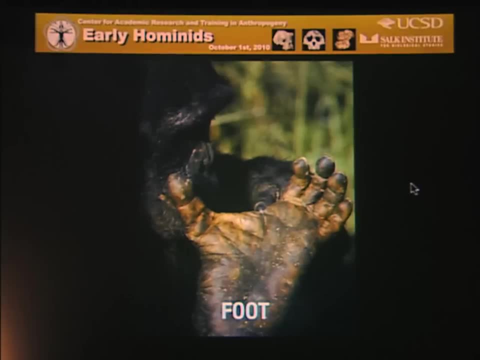 We take a foot of a chimpanzee. The old anatomist used to call the chimpanzees and gorillas the apes, the great apes, quadromanus, Because their feet are so much like hands. Interesting thing we found in studying this fossil from Ethiopia. 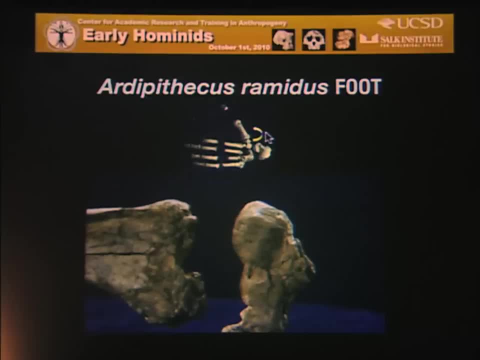 Imagine that you are Ardipithecus and you're looking down at the top of your foot. You've got a problem when you go to the shoe store because your big toe sticks out from the side. How do we know that about this creature? 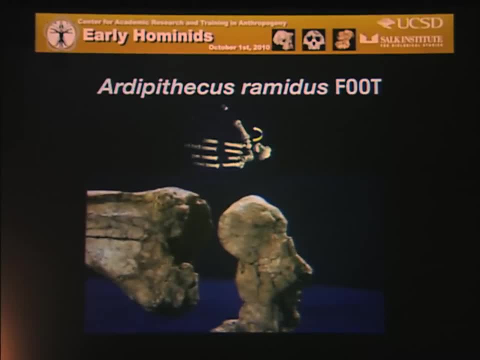 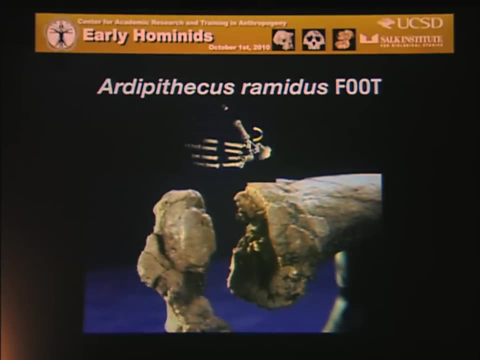 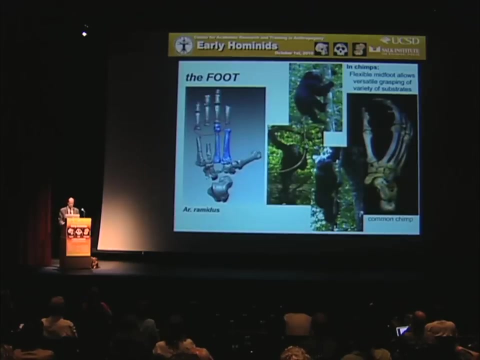 Because we can look in three dimensions at that joint. This is the joint right there And it's a hinge joint. Your toe won't do this. Nobody's toe in this room. your large toe can't do this. It can't rotate away from the foot like Ardi's can. 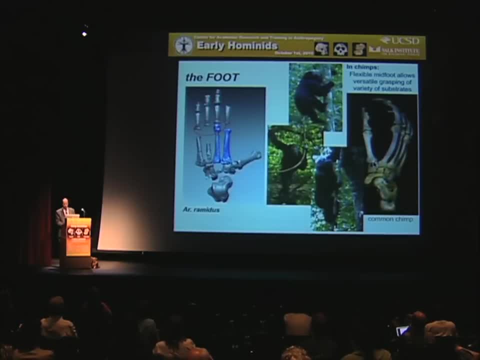 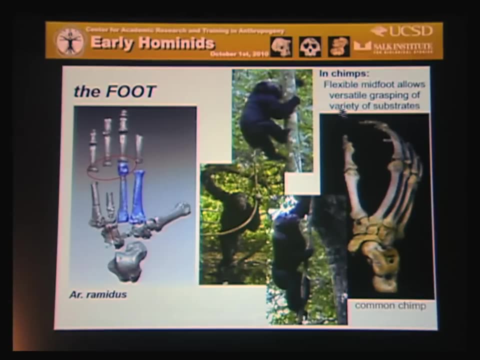 So there's the divergent big toe. That's kind of ape-like, But the rest of the foot is not ape-like at all In chimpanzees. they have very flexible mid-feet and they allow versatile grasping of a variety of substrates. 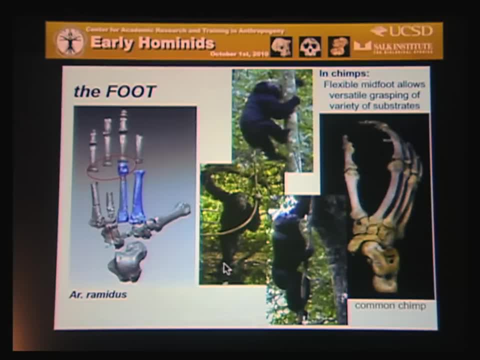 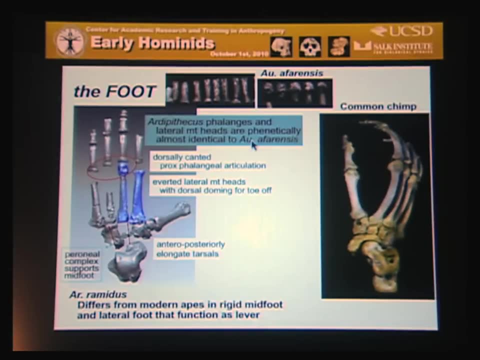 Here we see chimps grasping with their feet on these substrates In Ardipithecus. very different Their phalanges and these bones. here the metatarsals are very similar to later hominids like the Lucy hominid. 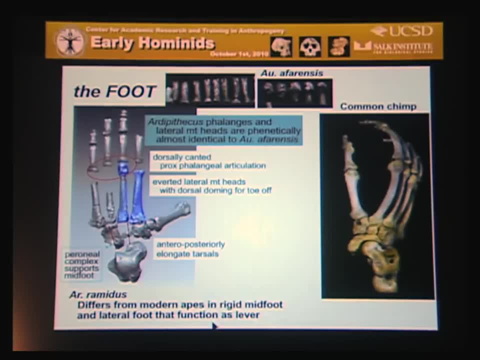 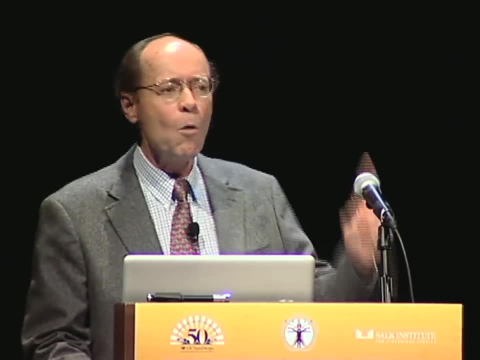 And they differ from modern apes in a rigid mid-foot and the lateral foot is functioning as a lever. Nobody's ever seen a primate like this before. The only way we can see it is to get the historical evidence, extract it from the record and analyze it. 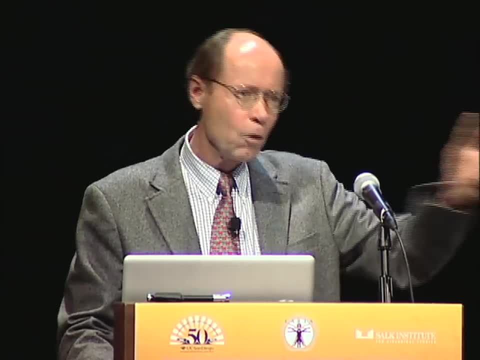 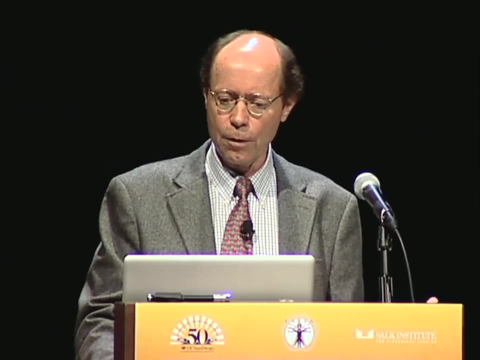 You cannot discover this looking at living chimps or looking at molecules of living chimps or living humans. You can only get these data from the paleontological record. The pelvis gave a similar interesting story. This is the pelvis. It doesn't look like much. 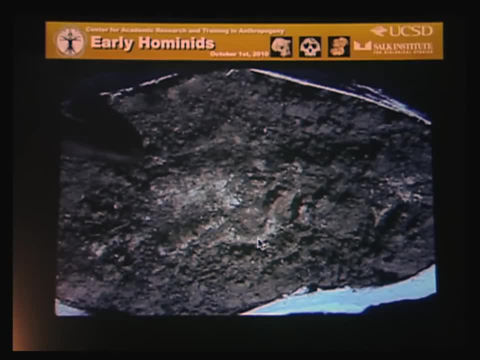 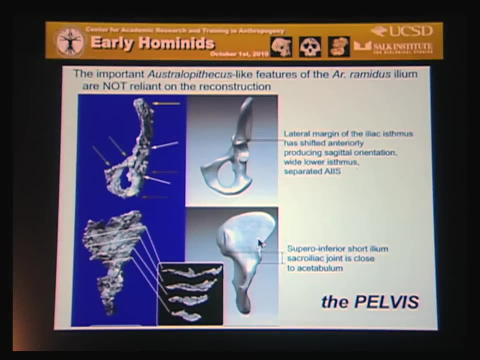 When you dig it out of the ground, you extract it in a plaster jacket because the thing's almost ready to fall apart. You clean it up. You clean it up more. It took a long time to clean this up. Then you have important australopithecus-like features of the ilium. 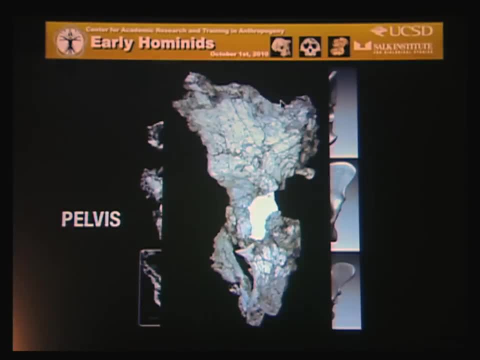 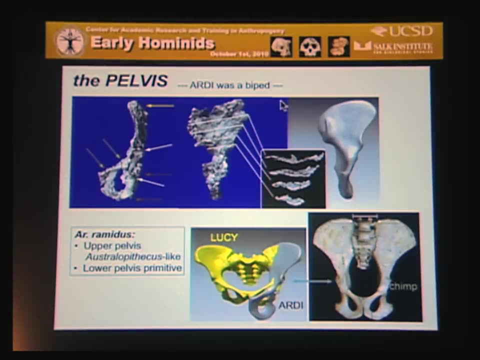 that aren't really reliant on this reconstruction. We can look at the bone itself. This is continuous bone across that surface. It's a very broad upper pelvis, Very australopithecus-like, But look at how far it projects down below Lucy in the back. 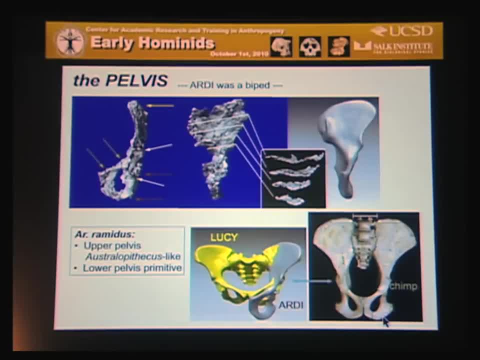 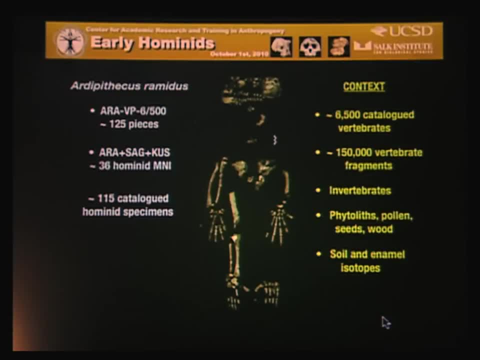 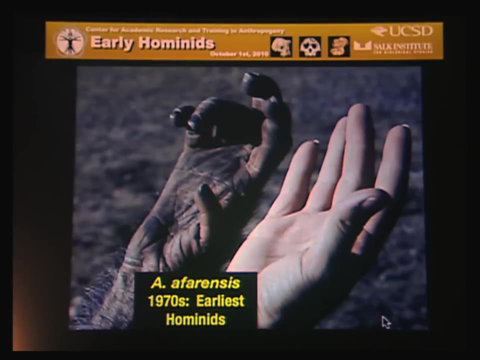 This is the part of the bone you sit on. Much more like a climbing chimpanzee, This is a mosaic organism. We have lots of pieces of it and other individuals. We have a lot of contexts, And so what that means is that we have new insights into relationships. In the old days, when the Lucy species was found in the 1970s, we were going with a kind of a bad model Afarensis. the fossils in the middle We compared to humans and chimps. In the 1970s we were impressed by how primitive Lucy and her colleagues were. 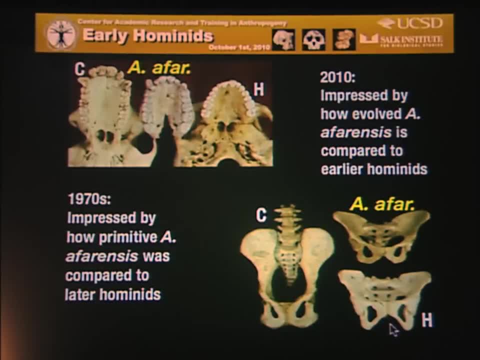 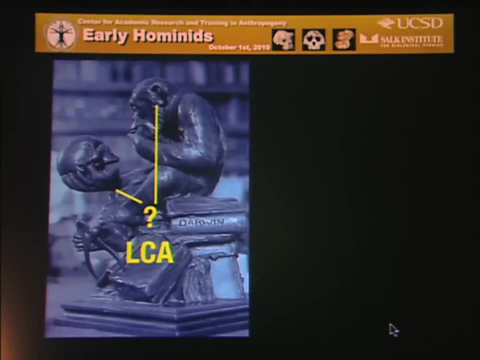 compared to later hominids. In 2010, we were impressed by how evolved Afarensis is compared to earlier hominids like Artie, Which brings us back to Darwin. When Darwin thought about this issue, Darwin didn't say: we evolved from chimpanzees. 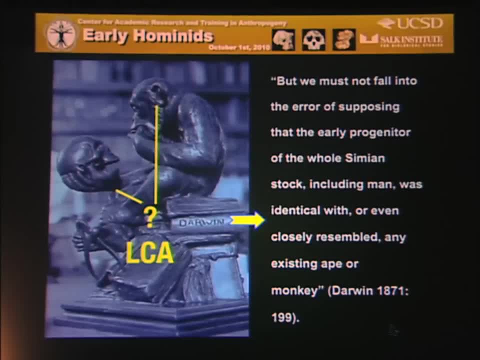 Darwin actually said: be careful here. We must not fall into the error of supposing the early progenitor or the whole simian stock, including humans, was identical with or even closely resembled any existing ape or monkey. He said that in 1871, with no fossil evidence. 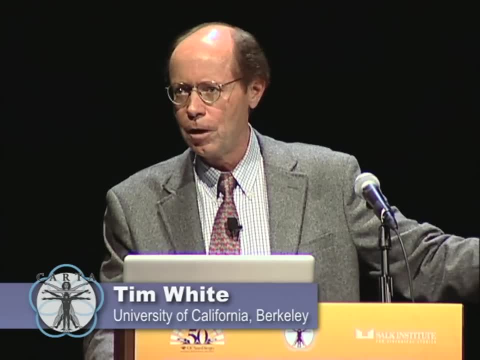 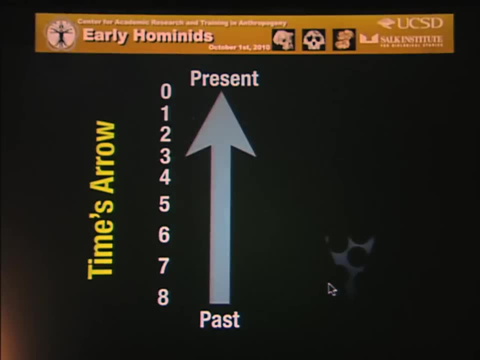 It was a clear warning that was ignored by generations of anthropologists who expected that we would find chimpanzees the further back we went into the fossil record. But it's hard because the further you go back in the fossil record, the harder it is to recover paleobiologically. 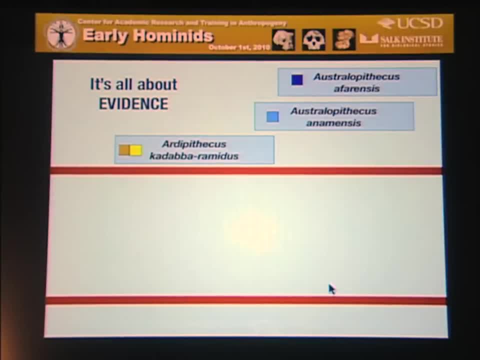 It's hard to recover the biological data. This subject is all about evidence. All of this evidence, all of the colored windows, are evidence from Kenya, from Ethiopia, from Tanzania, of completely new creatures that have been found since 1990.. 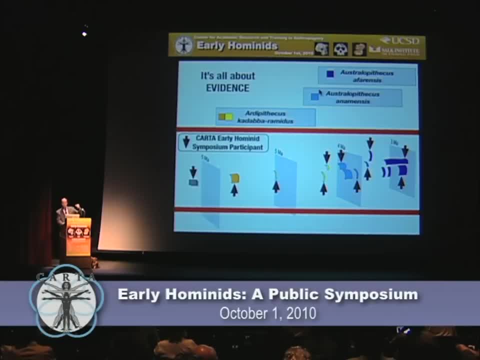 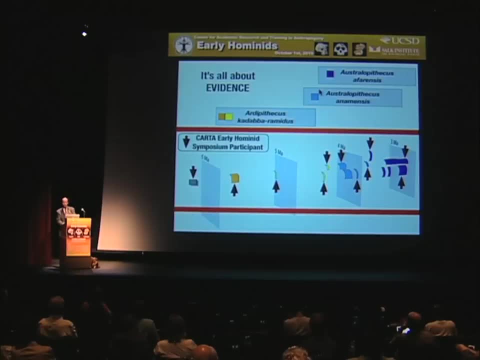 Today in this symposium, we have the people who found these fossils, who analyze these fossils. Every one of these single patches is represented by somebody here today who's going to discuss the fossils with us. But look at the thing: There are still mostly gaps. 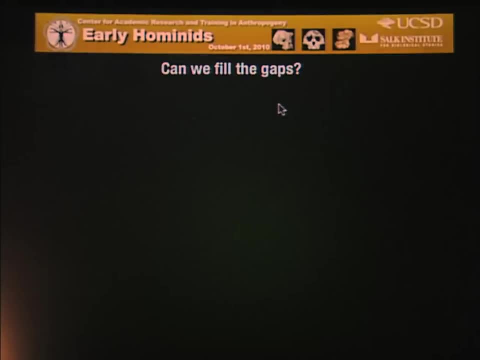 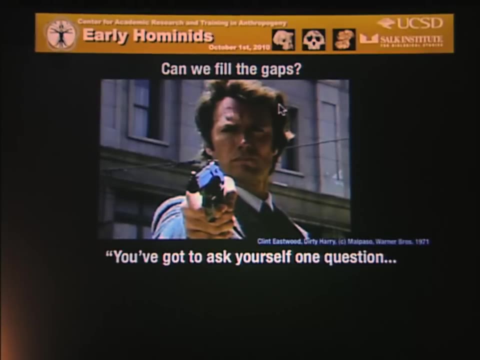 It's mostly not evidence, it's mostly gaps. Can we fill the gaps? Well, when you ask that question, can we fill the gaps? it reminds us of this guy, Dirty Harry, who said in 1971, you've got to ask yourself one question. 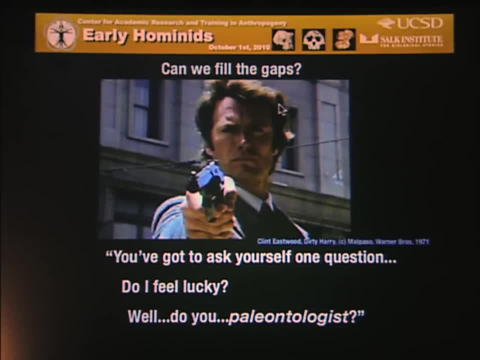 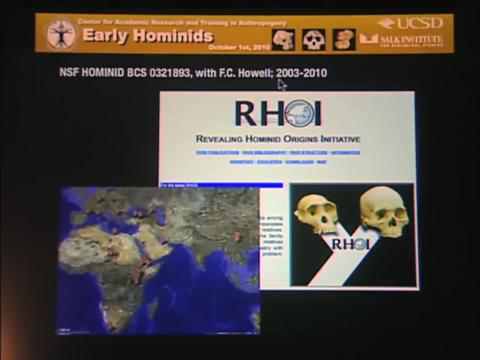 do I feel lucky? Well, do you? Well, back in 2003, we felt lucky and we got a lot of money from the National Science Foundation. We spent it before last year. Lots of those apes all over Europe. 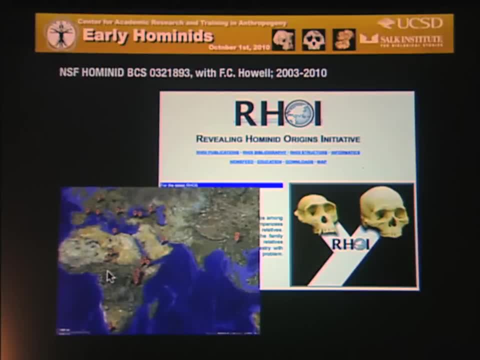 all the way over into China. were found A lot of things here in Africa: younger hominids, but the early hominids very, very difficult to find. You can read more about that at the website rhoiberkeleyedu. 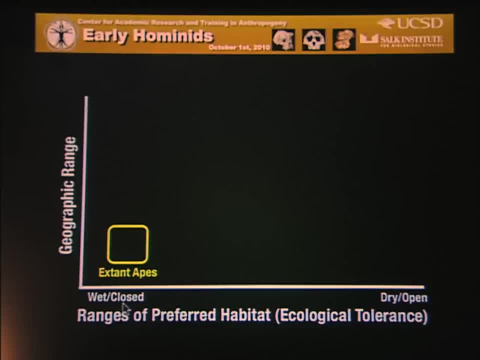 And here's what I think is going on. If we think of extant apes today, with geographic range, they also have a very tight range of habitat preference. The last common ancestor had a wider range of preferred habitats already, a little wider. 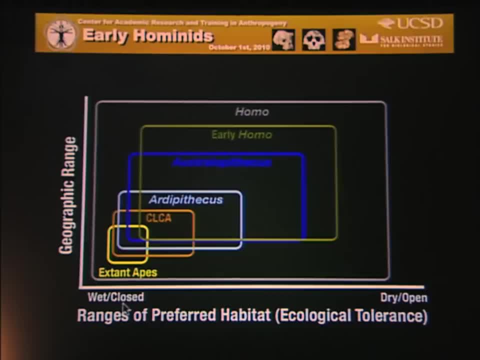 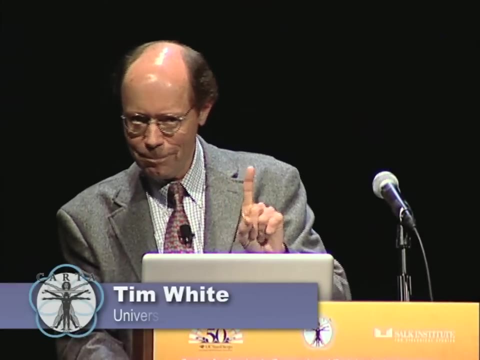 Australopithecus, wider, early homo, expanding with technology and finally we have homo sapiens. This niche expansion has been brought about by our evolving anatomy and technology in an interface, and there are a couple of pieces of bad news about this. 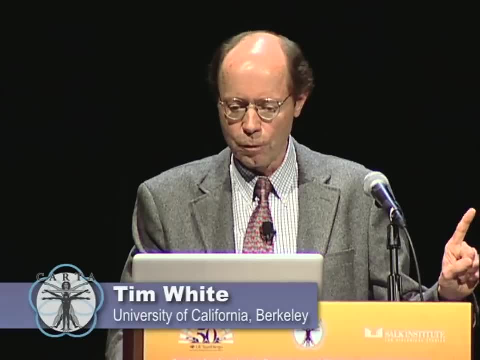 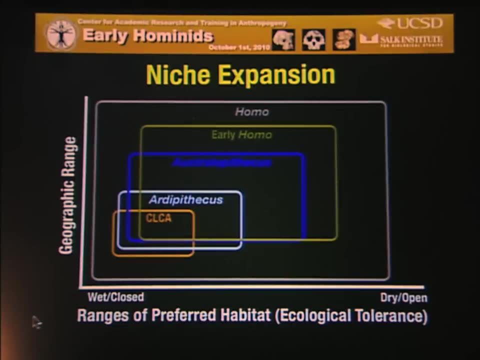 One, it's really bad news if you're an extant ape, because your habitats have been encroached upon and you're near extinction. And the other bad news is if you're a paleontologist, because the things that we're looking for down here 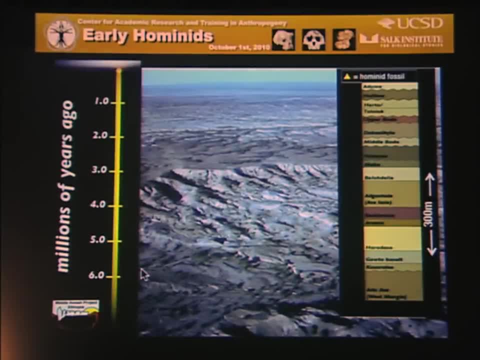 with this last common ancestor is very restricted in geographic range. So when we go to a big site like the Middle Awash, we can find Australopithecus above and Ardipithecus below. but to bridge that gap, right in there, 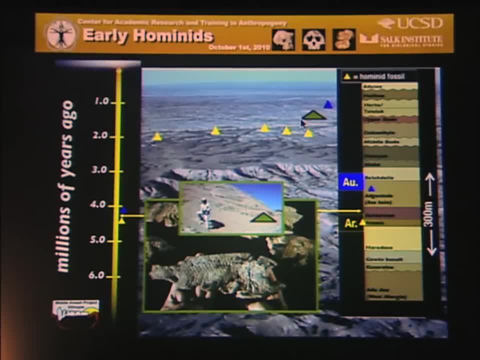 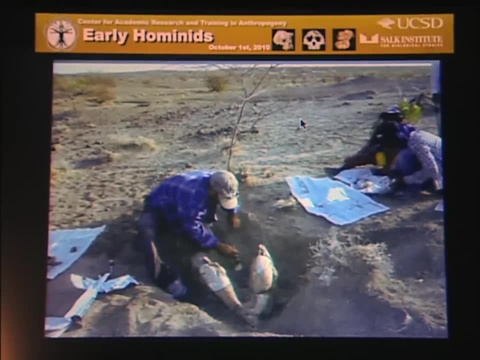 we find our outcrop is a lake. There are lots of fish but no primates. And still we go back to the field every year and we hope to find something Here, excavating a wonderful elephant mandible 5.2 million years ago. 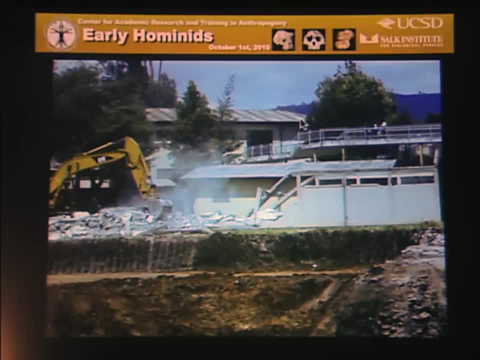 Here's another excavation. What the hell's going on here? Are they starting from the top and digging down? And the answer is no. We're taking down a National Science Foundation-sponsored laboratory that served as a repository of these fossils until about five years ago. 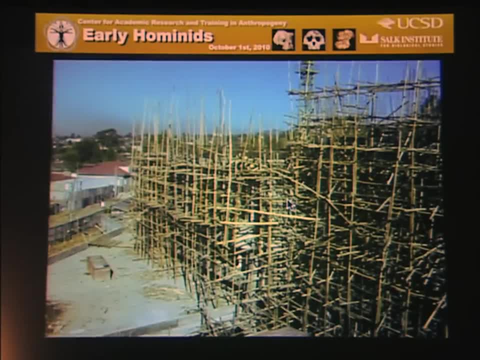 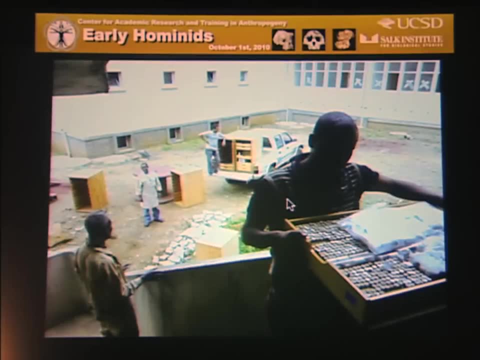 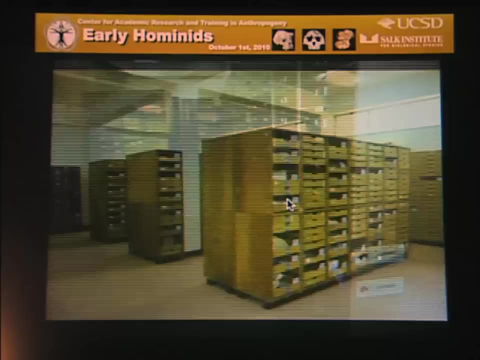 when the Ethiopian government began to build a gigantic new facility in Addis Ababa. This is the paleoanthropology wing It opened this spring. These are the fossils moving into that facility: Elephants, rodents, birds, all those fossils. 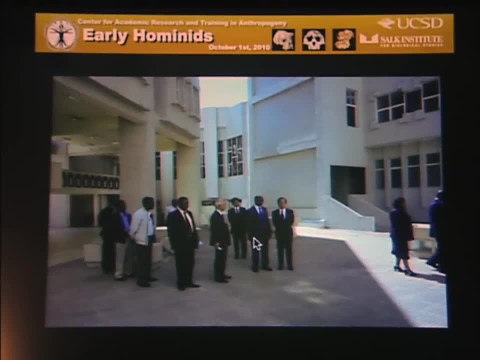 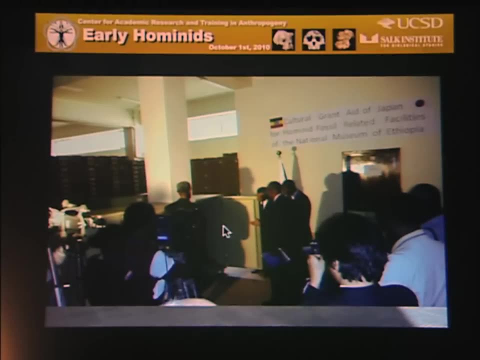 including the hominids. This is the Ethiopian Minister of Culture and the Japanese ambassador to Ethiopia, who donated wonderful new materials. Gansuwa, who's here today, instrumental in this, in the creation of a facility. And so I'm going to close this talk. 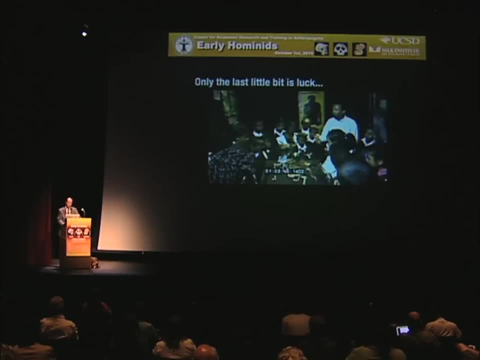 not by looking to the past, but by thinking about the future. One of the points I want to make is: the things that you're going to hear about today are not here because of luck. Only the last little bit is luck. The rest of it's hard work. 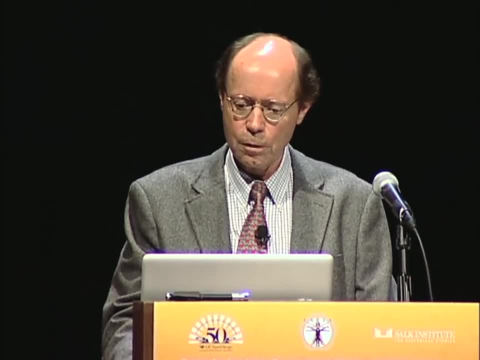 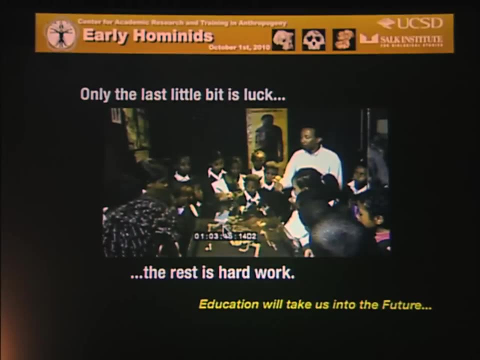 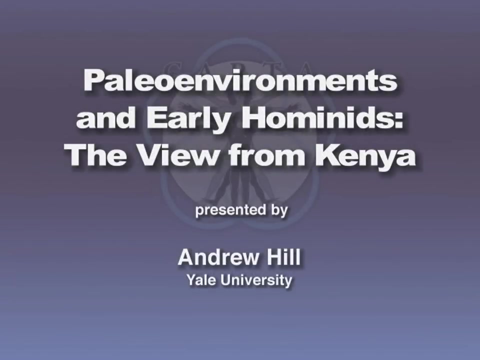 And these are the people who have done the hard work to generate these fossils. And the other thing I want to close with is that education, evidence, rationality and science is what's going to take us into the future. We are now going to hear from Andrew Hill. 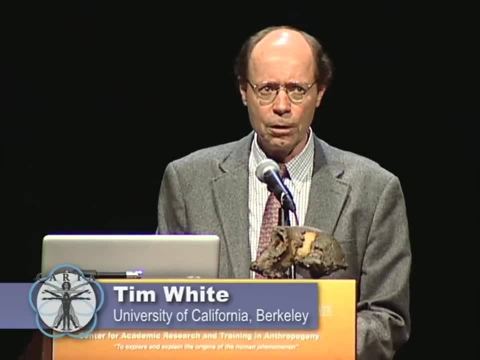 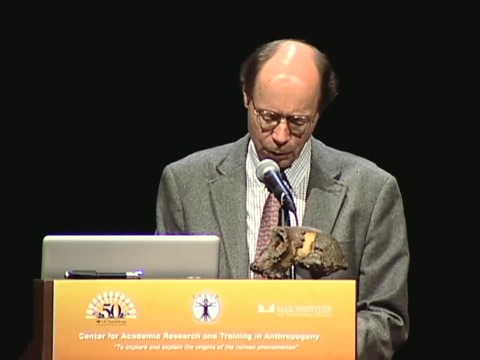 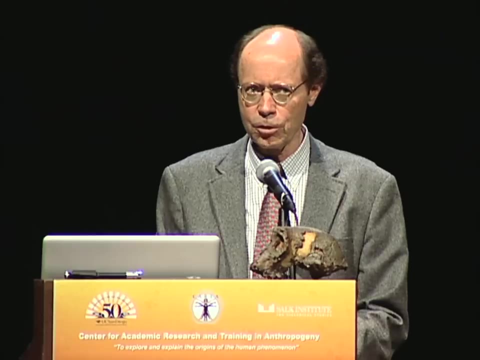 of Yale University, who has been working in the Tugan Hills of Kenya for as long as any of us can remember. He'll be talking about paleoenvironments and early hominids and giving us a unique view from a little bit to the south. 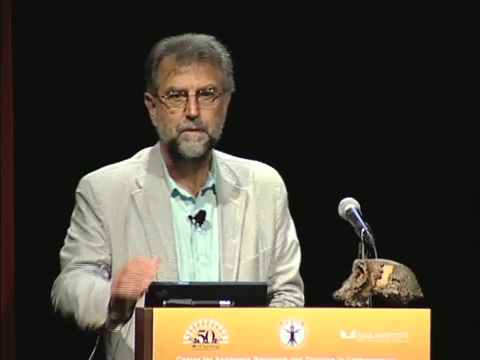 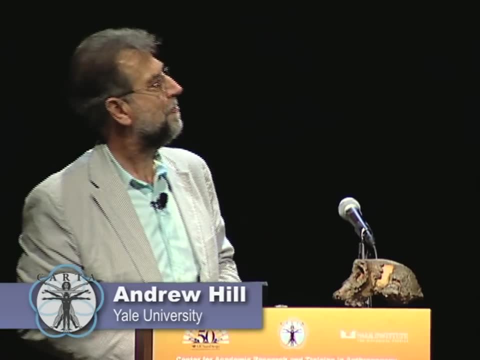 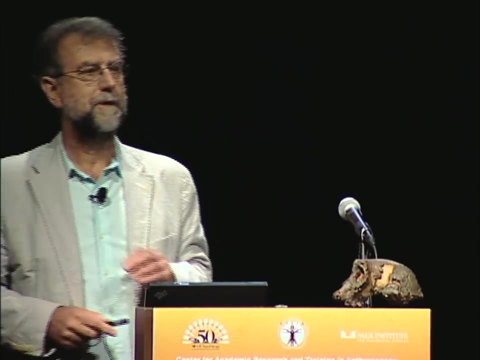 in the Kenyan Rift Valley, Andrew Hill. Good Well, thank you, Tim, and thank you for the organizers for inviting me to take part in this amazing event. I'm going to be talking mainly about context, which Tim said we were not really talking about. 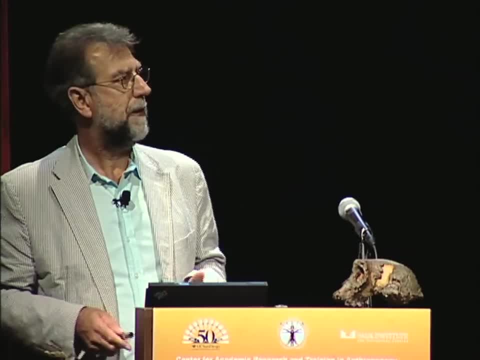 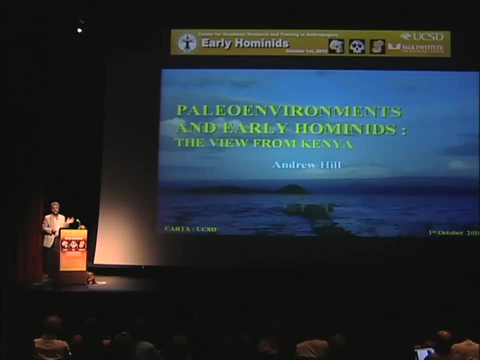 in great detail, but I think it's really important to understand perhaps how hominids arose at some remote time in the past. And there are early hominids from Kenya, some of which even my own expedition has found, but I'm not going to be referring to those today. 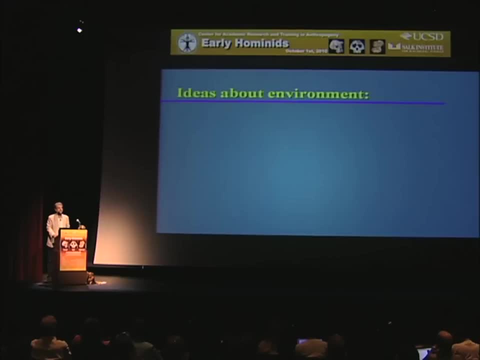 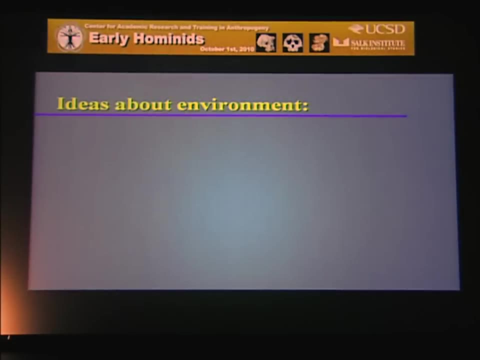 but to talk more about environment. There's been a number of ideas about the environment of the earliest hominids knocking around. They're buried- but they all focus on two main elements, And one of them is the concern that the origin of the human lineage. 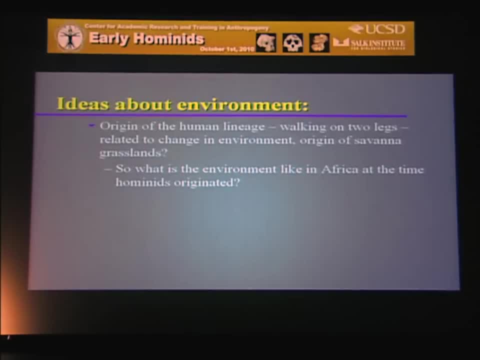 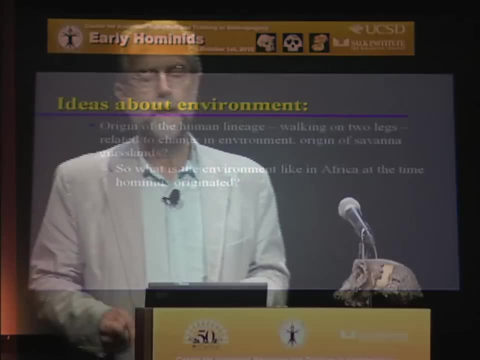 which is mainly characterized by walking around on your back legs, which is a rather unusual thing to do, has got something to do with climate and environmental change, And this goes back all the way to Darwin, who thought that bipedalism and the origin of humans. 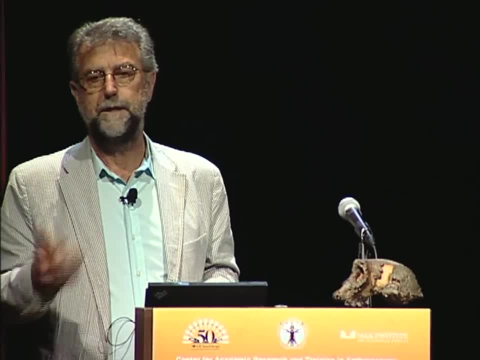 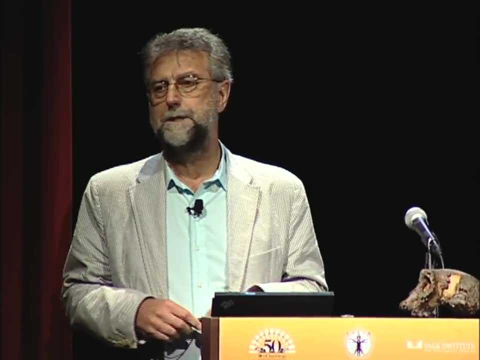 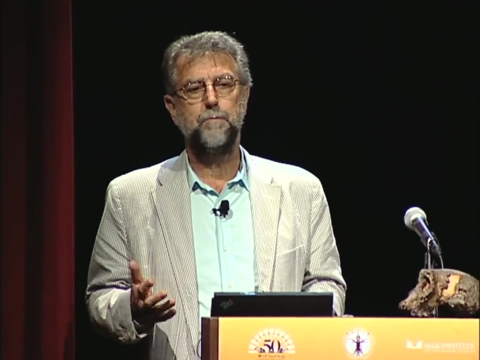 probably came about as a result of changes in the environment And particularly it's been related to the alleged origin of grasslands in Africa, the idea that it was once covered in forest and then changed to grasslands. So it's really important to try and find out. 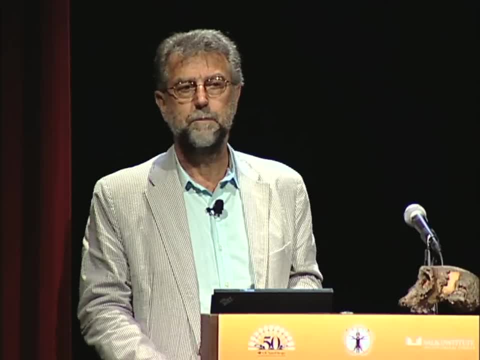 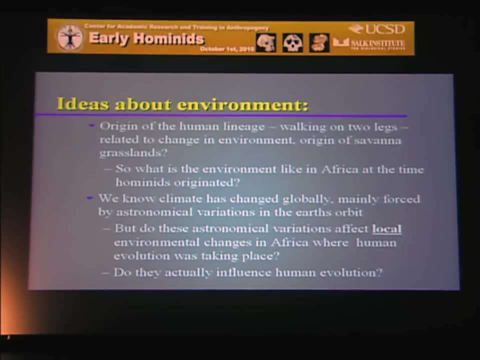 what the environment was like in Africa at the time that hominids originated, to be able to see if this is true. The other element that's going around, which is really rather similar and related to it, but has some differences, is that we now know from a lot of work. 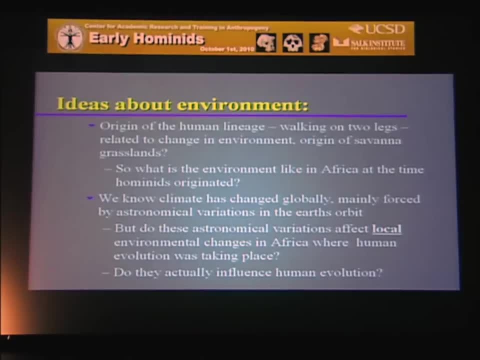 that global climate has changed quite radically over the last. well, certainly three more million years, six, seven, But it's done so. the data relates to global change and to, of course, of average global change, And it's mainly caused by variations. 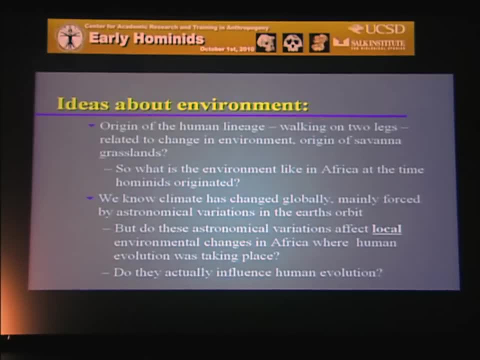 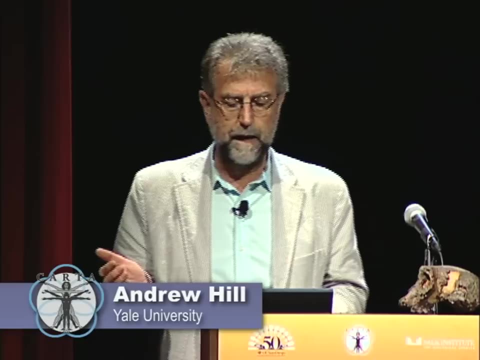 in astronomical wiggles of the earth as it goes around the sun, And so the question is- and this has been implicated in the origin of humans as well- often linked to the origin of grasslands. but the question is: do these astronomical changes? 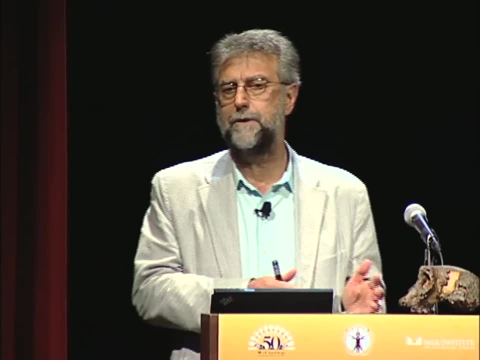 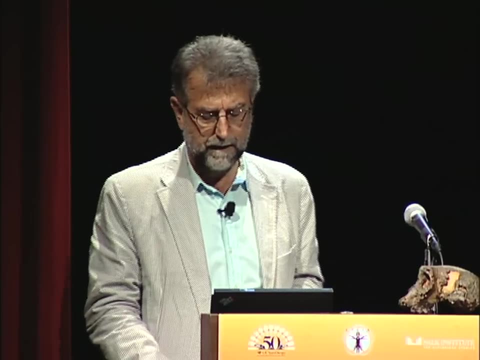 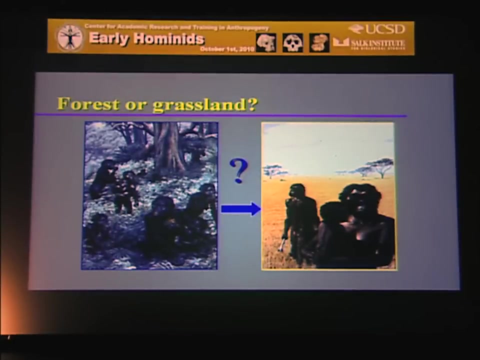 really affect relatively local areas of Africa where we believe human evolution is actually taking place, places in the middle of the African continent? Does it really affect them and does it really influence human evolution? So that boils down to this vague cartoon here about whether you've had the origin of grasslands. 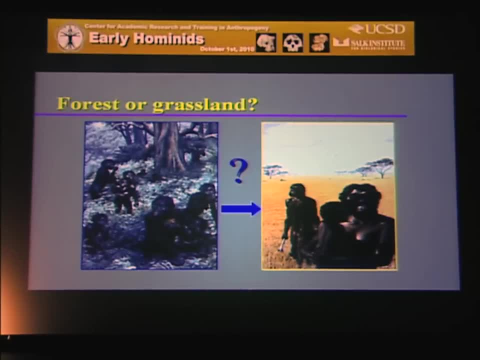 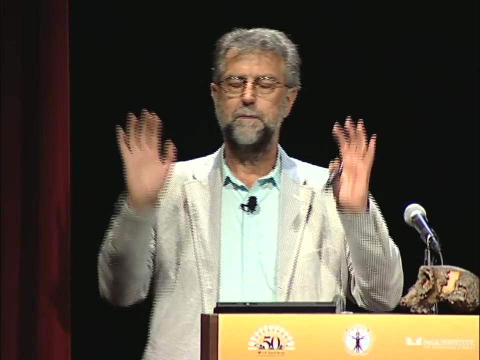 at some relevant time? and if so, and if not, where did early hominids originally evolve and live? Did they evolve in woodlands and forests, or did they evolve in grasslands? The idea is sort of appealing that grasslands come along and some ape gets up on its back legs. 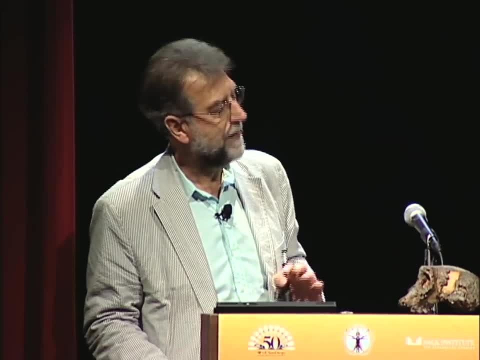 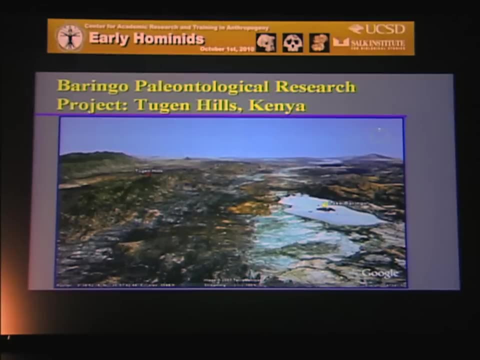 and waves its hands about and wonders what to do with them. But is this grounded in any truth? My project, the Beringo Paleontological Research Project, as Tim says, has worked for longer than even I can remember in the Tugan Hills in Kenya. 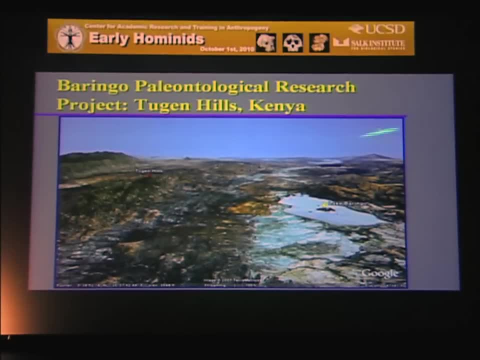 And this is Lake Beringo, just here, looking north along the Rift Valley. Lake Takana is somewhere on the horizon. This is the western edge of the rift, This is the eastern edge And these are the Tugan Hills in the rift. 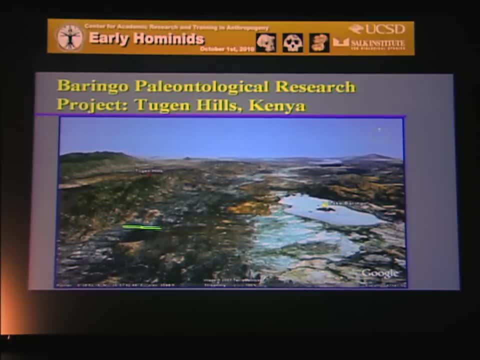 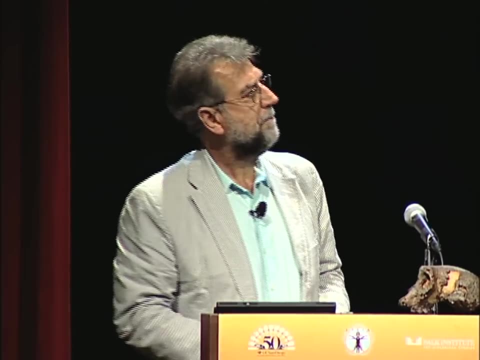 extending all the way along for 150 kilometers, with down here lots of fossiliferous sediment that go from about 15.5 million to about now. I'm going to talk about three lines of evidence. Finding out about environments is more difficult, perhaps, than most people would think. 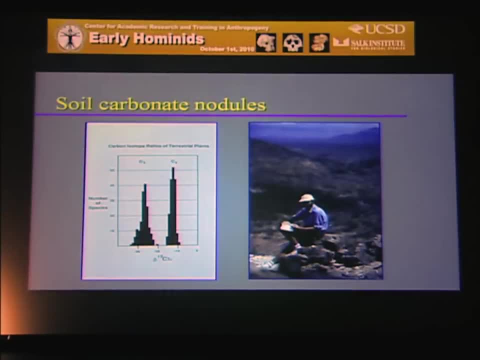 and more difficult than I would hope. But I'm going to talk first about soil carbonate nodules And soil carbonates form in soils where they sort of coalesce, And you can find them in fossil soils as well, And it turns out. 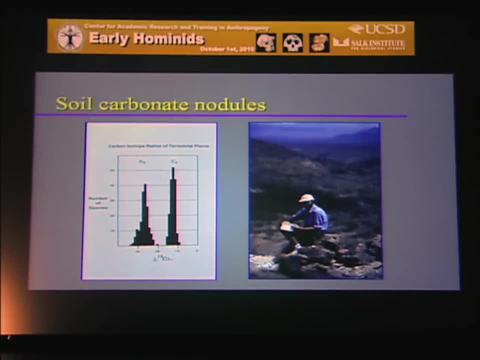 This is John Kingston, a colleague of mine who's done most of the work on this and works with me in the Tugan Hills. It turns out that plants of different kinds fractionate on incorporating their tissues carbon isotopes to different degrees according to what kinds of plants they are. 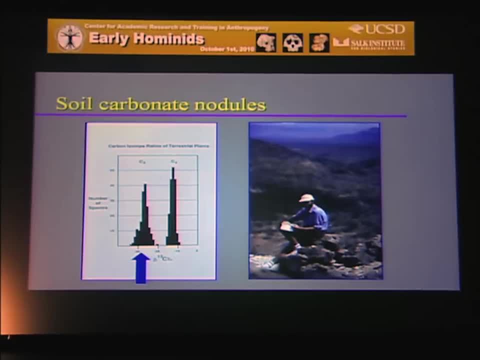 And plants that you find in woodlands and forests have carbon isotopes that range over carbon 13- over this sort of range, And grasslands which are out in the open in sunlight have carbon 13 in that sort of range And we didn't really worry about that. 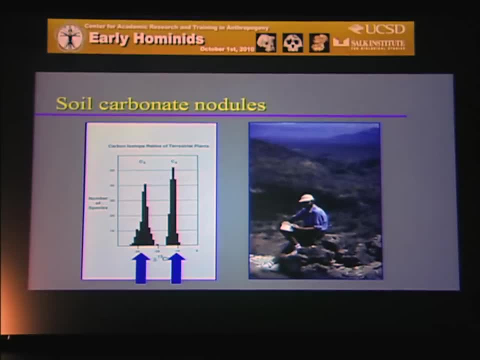 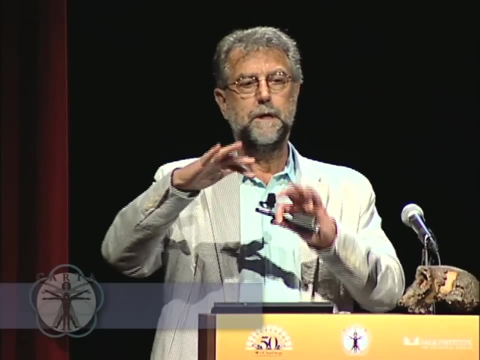 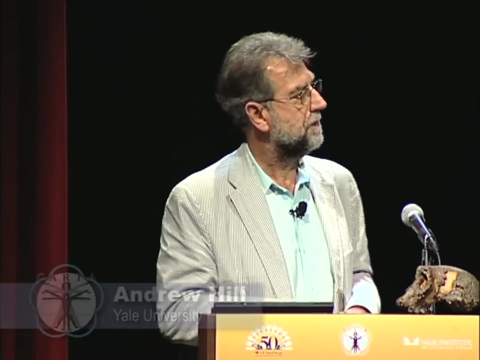 It's simply that this provides a means of detecting one kind of plant from the other, because it turns out that rainwater and soil water preserves this signal. It gets incorporated in these little lines called nodules in soils And you analyze the soil nodules for the carbon isotopes. 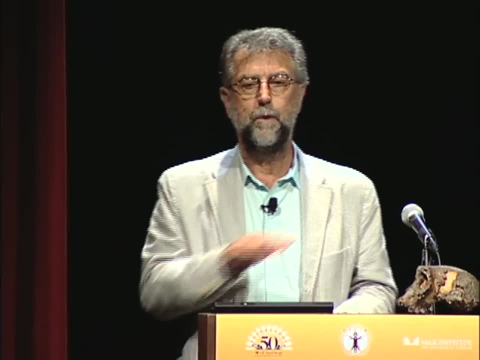 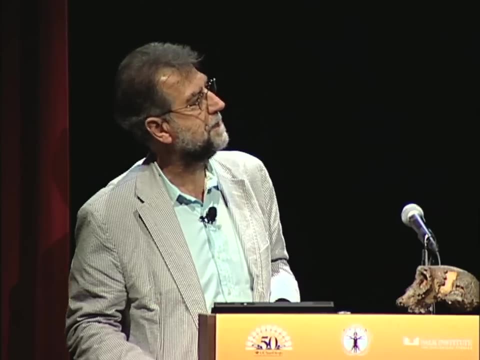 and you can tell what sort of plants were living on the surface, whether they were grasslands or whether they were forest or woodland, And it's a very neat little trick that gets at some of the information we feel we want This started, really, as far as I was concerned, 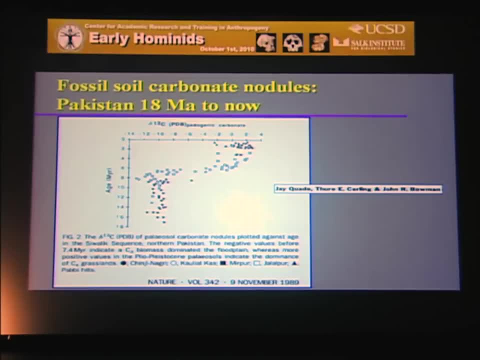 with some very neat work a long time ago by someone called Terry Serling and his group. And this is Pakistan, And you didn't worry about the details of the graph, But this is 18 million years here and zero here, And all that means is that these are samples. 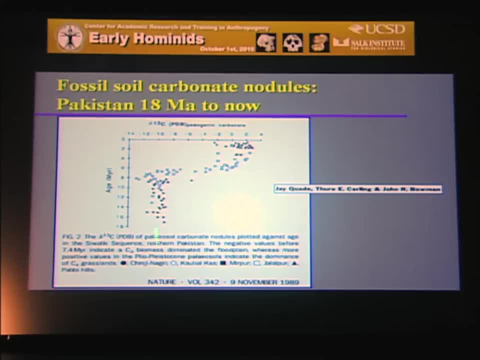 of soil carbonates through this time period that represent woodland and perhaps some forest, but certainly closed environments. And then all of a sudden, at around 7 million years- wow, it goes straight across here. And from then onwards it's all grasslands. 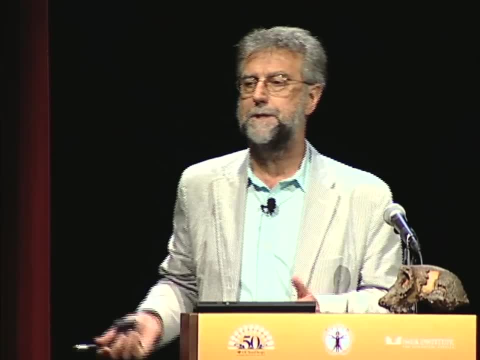 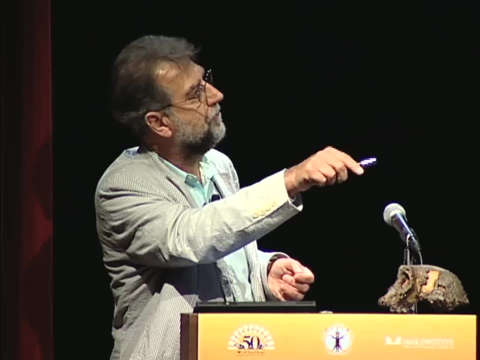 And it's really very neat because this correlates very nicely with changes in the animals at the time. Apes disappear, monkeys come in, There are all kinds of wonderful things in the fauna changing, And John Kingston and I and probably 1,000 other people- 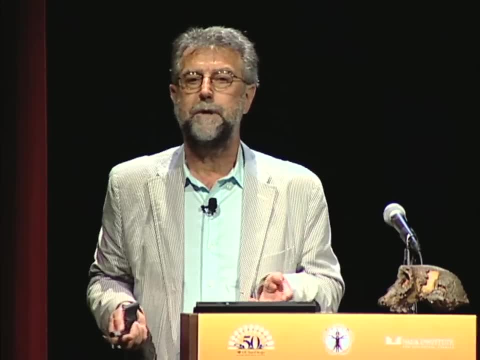 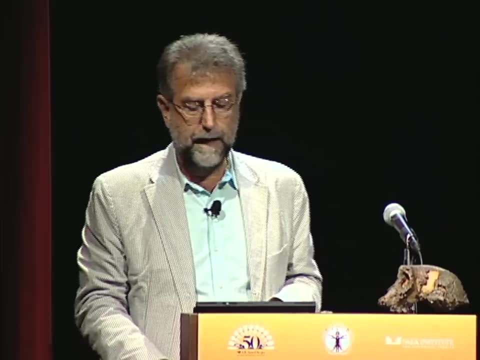 thought: well, this is very clever. What if this is going on in Africa? Because that's just about the time that we thought that hominids were beginning to evolve And we had a section of rock from 15 million to now which made it possible to test this. 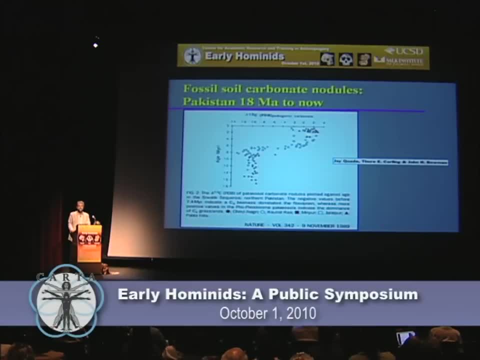 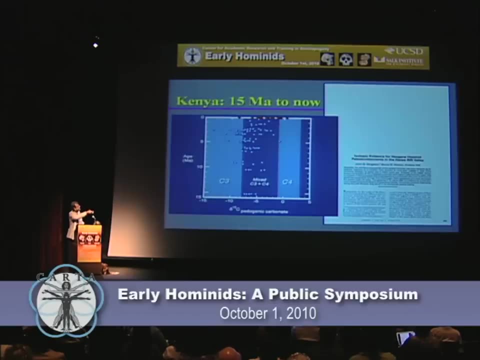 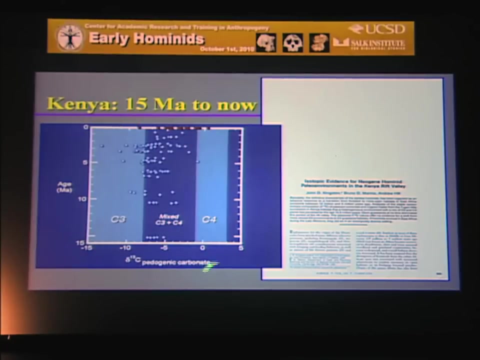 So John went back there to Kenya and we sampled all of this. All of these carbonate nodules are rather heated and worked out the carbon isotope ratios. This band here includes things that are woodland and forest. This here is grassland. 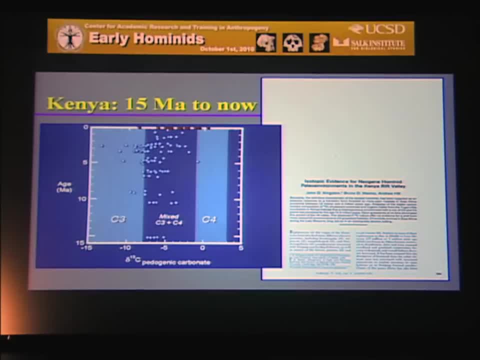 And you can see that the results are not at all like Pakistan. All these dots are somewhere in the middle and they're very, very mixed. There's some more extreme ones. Here's a good bit of forest. There's one here that's almost in grassland. 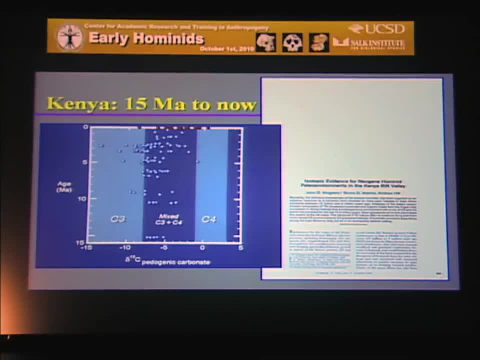 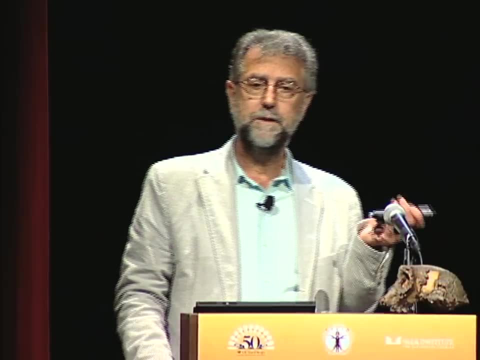 But essentially they're changing through time, but with no predictable changes. You don't see grasslands suddenly coming in. There are no savannas here, And this is in the Rift Valley, where the majority- practically all, with the exception of this lovely person. 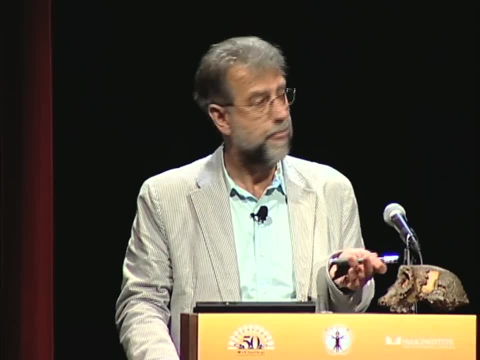 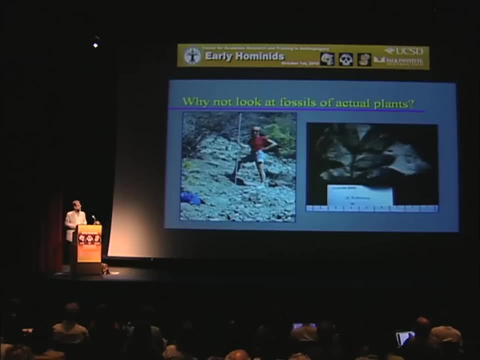 where all of the hominids that we know about have come from. Why don't we look at actual fossil plants? Well, we do, But these are very rare And we're fortunate in having quite a few fossil plants in this sequence. 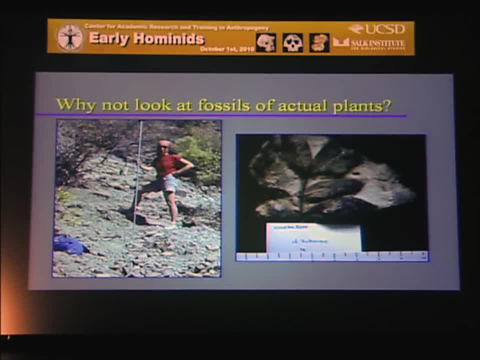 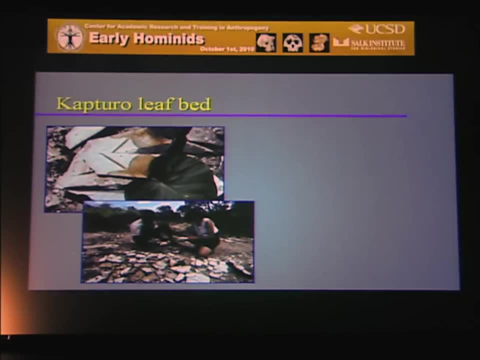 This is Bonnie Jacobs from SMU, who has been working on our plants for a long time, And I'm just going to mention two sites of several that are particularly relevant. This is one called the Capturo leaf bed, And its age is between 7.2 and 6.7,. 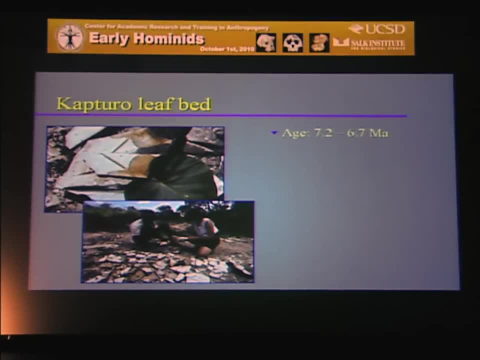 just about this time round about the origin of hominids, And the leaves here are preserved in what's known as diatomite, which I'm going to talk about more in a minute. They're beautiful, clean rocks that are bedded beautifully like sheets of paper. 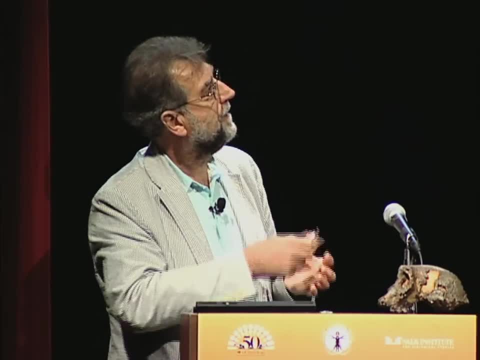 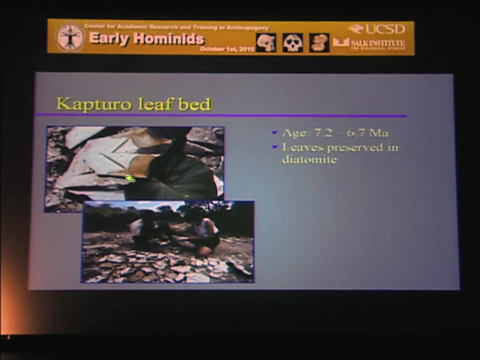 And you can just sort of fold these sheets of paper open and you find plant fossils impressed upon the pages, as it were. This is one that I plucked down from a tree above me when I found that, but I'm told it's not the same species. 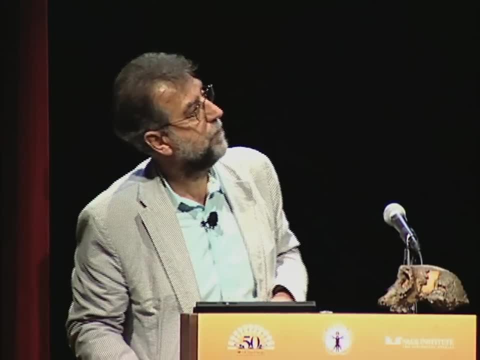 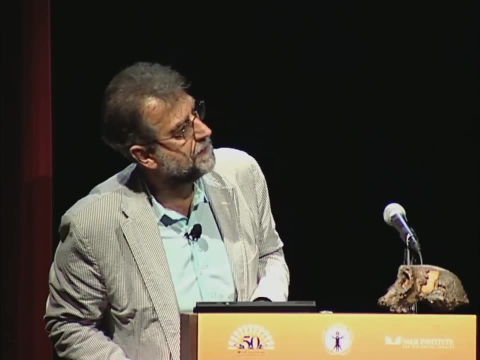 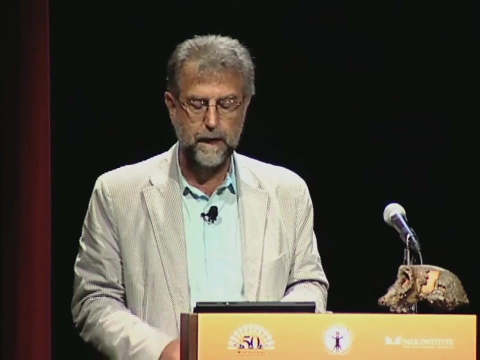 which is a pity, But we got a lot of plants from this place And the environment- from looking at what species they are- suggests that this is a seasonal, deciduous woodland. It's not a total forest and it is seasonal. Now here's something that I'm not going to have time to go into. 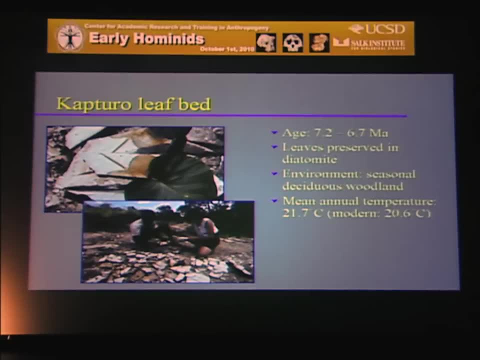 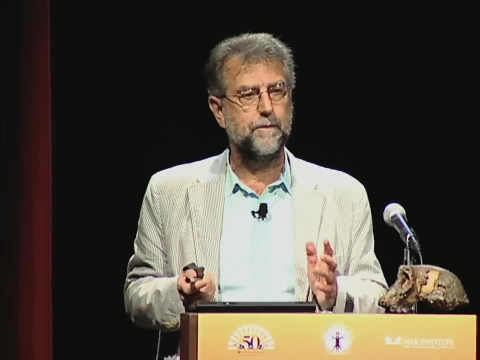 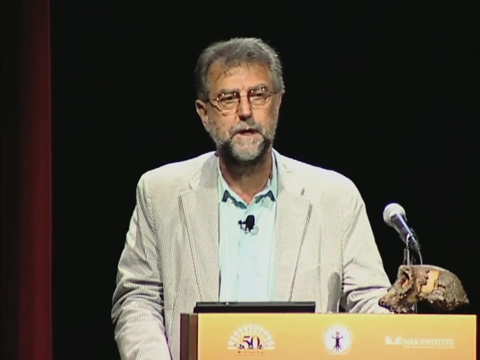 and you may not believe, but trust me, It turns out that you can. from the indentations on the edges of leaves, you can work out the temperature and rainfall that they grew in- And Bonnie has done this work- and the mean annual temperature at the time of this site. 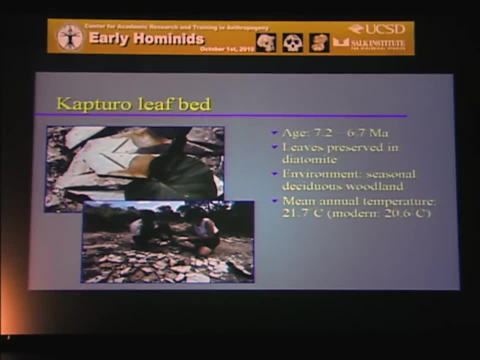 was 21.7 degrees, which is slightly higher than the temperature now, and it's not cold there by any means. So this is quite warm. You can work out the wet month precipitation, which is 627 millimeters a year, which is not very, very wet either. 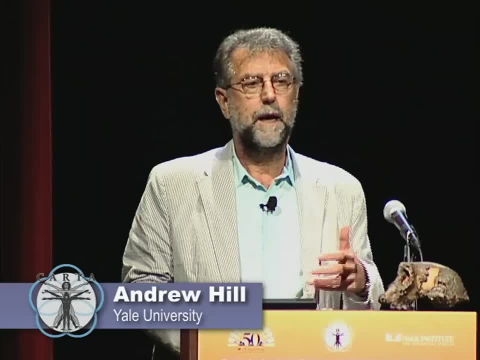 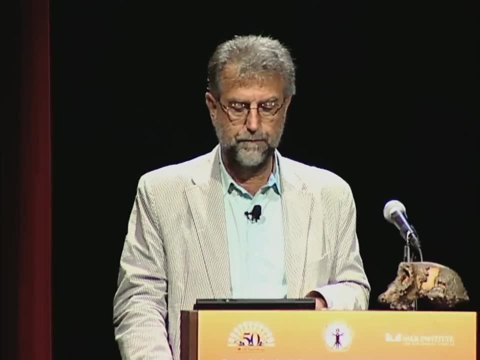 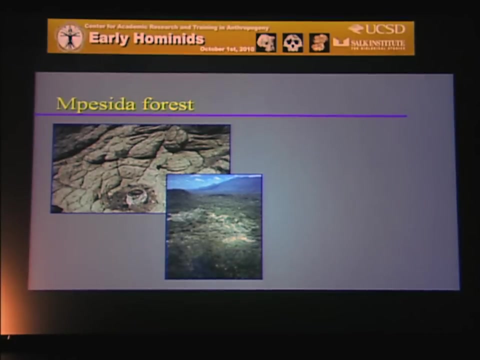 But even though it's relatively dry and relatively warm, this is not a grassland by any means at all. This is a full woodland right at the beginning of the human lineage. The next example is something we call the Imposida Forest. This is 6.3 million years. 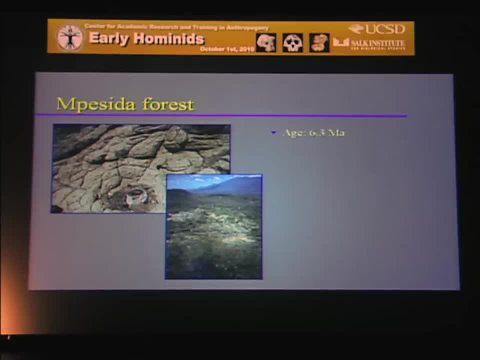 a little younger, not much, and still relevant to our origins, And what's happened here is that trees have been preserved in a massive airfall: tuff, It's gunk that's come out of a volcano, very hot and coarse, and has fallen down right on the forest. 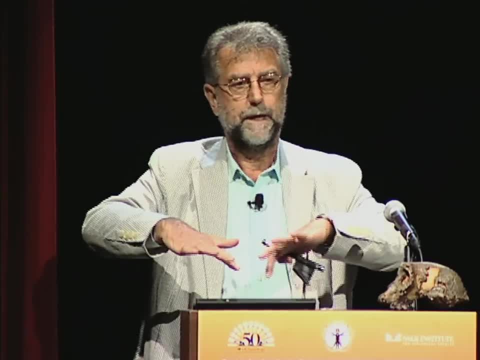 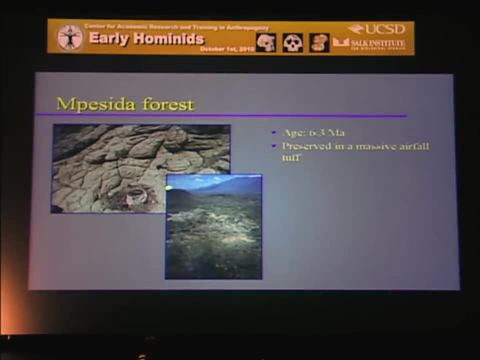 killed it. It's kind of planty Pompeii really. It just preserves stuff underneath And it's preserved some of these trees actually in place, And so what you're seeing here is a tree trunk. That's just the middle bit. 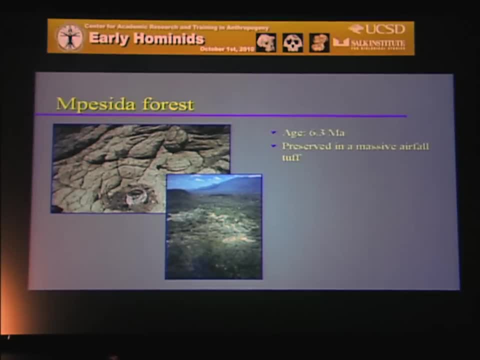 and the whole base of the tree is that And it's been preserved in this very coarse rock and you can actually see trees in their growth position. This is mainly silicified wood. There's a lot of other wood available there And it covers quite a large area. 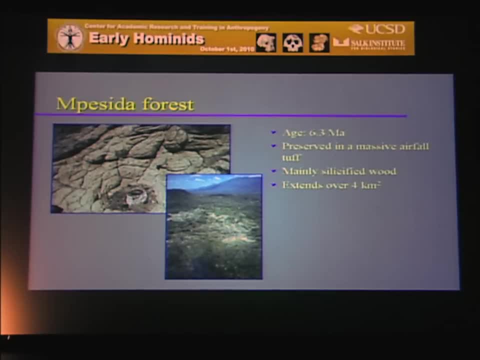 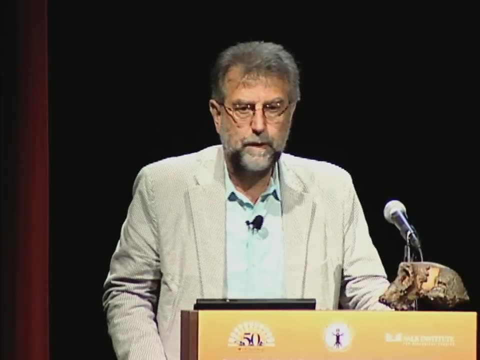 You're looking down on it here. It's about four square kilometers and you've got quite a bit of the forest there. There are only six species identified so far, but they all show that this is a wet or moist lowland or upland forest. 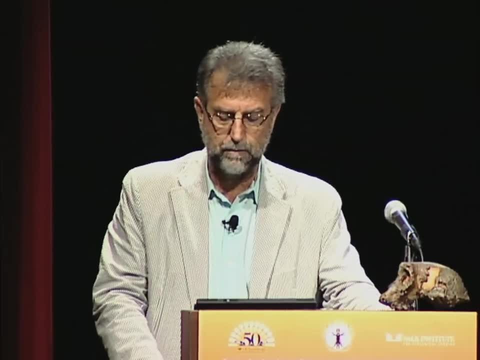 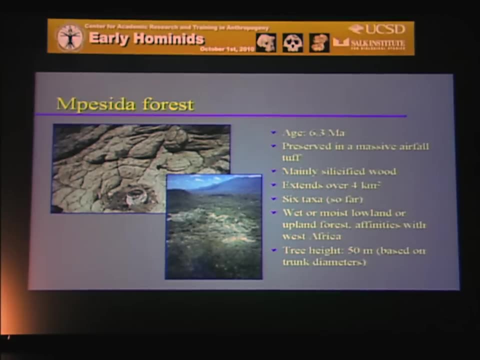 with affinities to real West African rainforests. Now there's a good correlation between the diameter of a tree trunk at the base and its height, and what we can conclude from measurements on several trees that are in position is that these trees were at least. 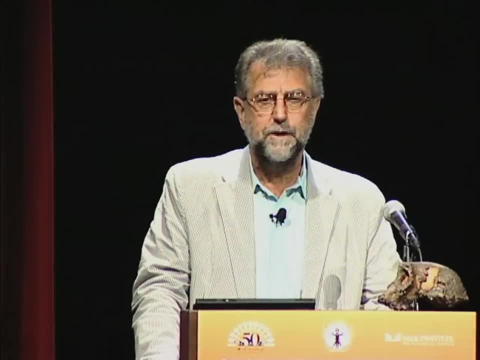 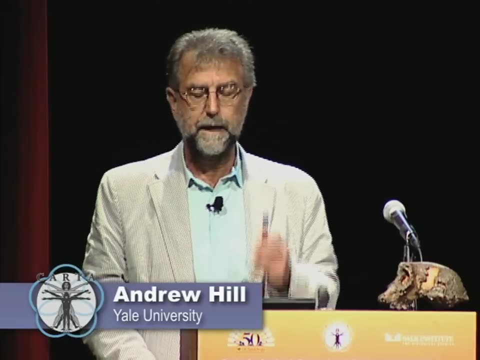 50 meters in height. These are huge trees. I mean, this is not some little woodland, These are giant forests with enormous trees growing there In the Rift Valley, where we know hominids lived at the time or shortly after. 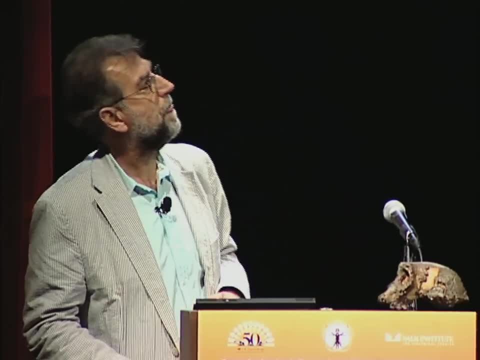 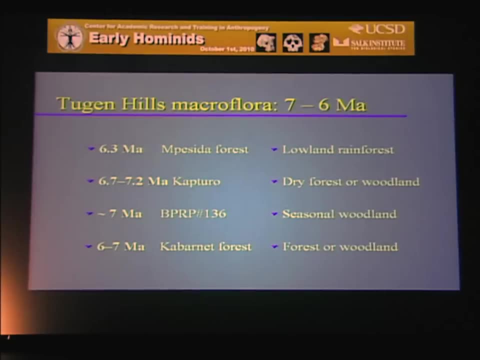 they were diverging from the line leading to chimpanzees. Here's just a few other sites around this period. You can see that, although there's some variation, ranging from this dry woodland that I spoke about to the real rainforest, they are all forests. 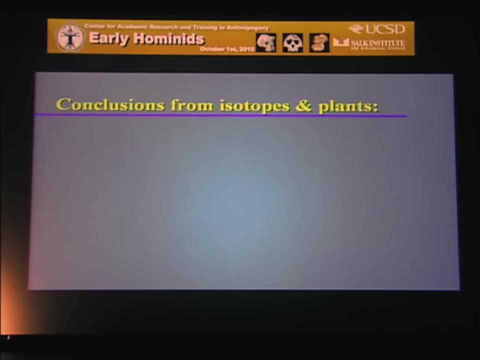 There is no sign of grassland at all during this time. So the conclusions from both the isotope work of John Kingston and the plants from Bonnie Jacobs is: firstly, with the isotopes the signal is not at all like it is in Pakistan. There are no significant trends through time. There's no abrupt changes. There's no change into grasslands- The conditions in the Rift Valley have been variable through time- but no sign of these grassland ecosystems or savannas at any point. At times they were forests of various kinds. 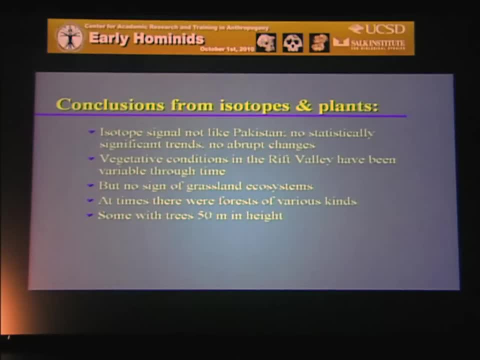 and in fact, for much of the time, some with trees 50 meters in height. So you have these serious forests in the Rift, more or less at the time of divergence of hominids. Moving on to some other information which we're more recently developing, 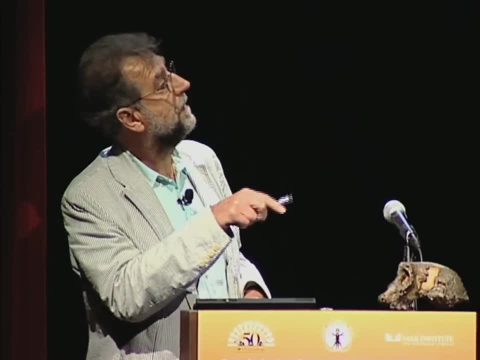 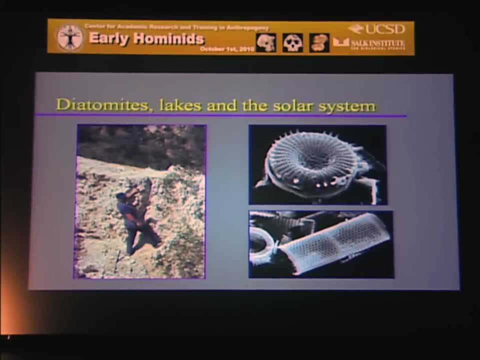 is to do with diatomites, these beautiful rocks that I mentioned with regard to preserving the leaves, And this is Bob Edgar from the Farlow Herbarium at Harvard, who actually works on the diatoms. And these are diatoms: They're microscopic. 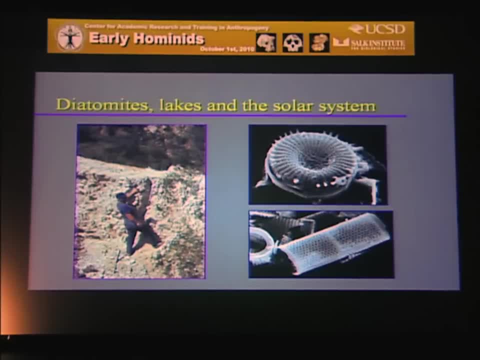 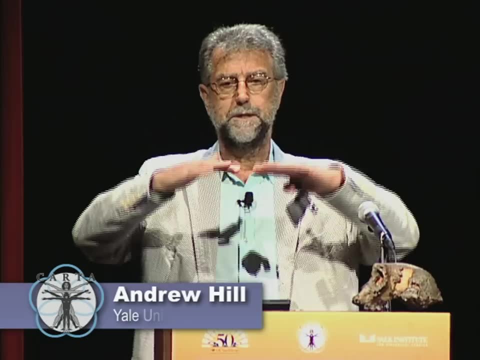 They're blue-green algae and they have these little skeletons made of silica and they look like little cheese graters And they basically the rock is formed of these things, just because when they die, there are lakes that are undisturbed. 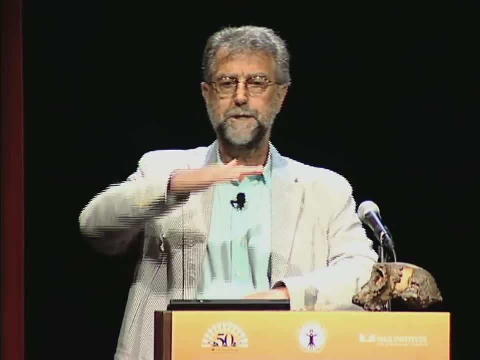 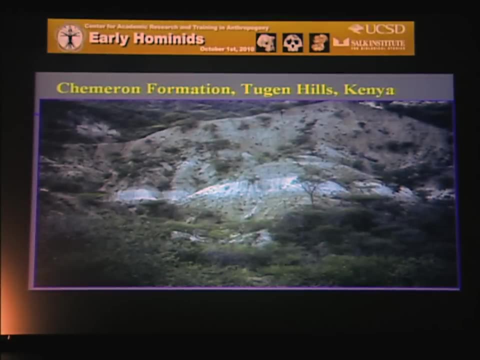 and they just sort of rain down their little corpses onto the bottom of the lakes and gradually accumulate, And this is very convenient for us. We were working in the Chemron Formation, one of the units that we have in the Tugendhills. 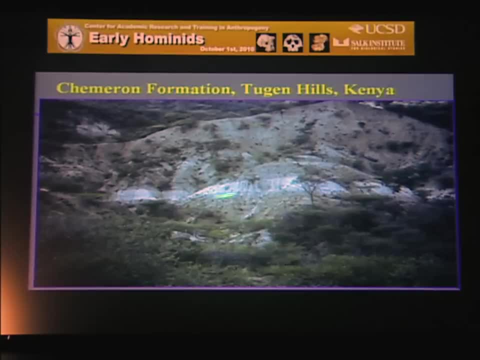 and noticed that what we had here were. There's a diatomite here that you can see, nice clean white rock. There's another one here, I think, there's another one there, There's another one just here. There were five of these things. 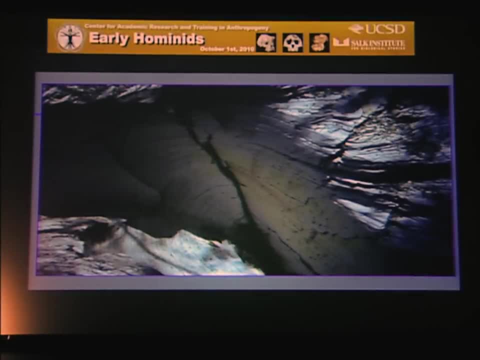 in a very short bit of section. Here you can see what they look like. You can perhaps detect these beautiful, fine bedding planes that are perfectly smooth and even and uninterrupted, And here's what they look like. This is one of them. I'm standing here for scale. 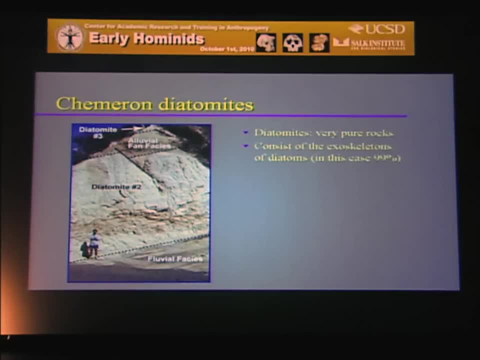 It's quite a large one, And so they're these very pure rocks. They consist almost entirely. In this case, 99% of the rock is just these little exoskeletons of the diatoms of microscopic things. We've got five of them in this part of the section. 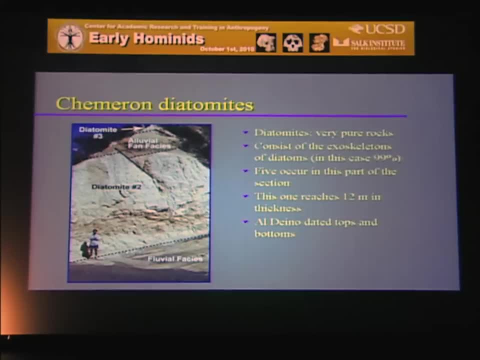 Some are very large. This is 12 meters in thickness And Al Dano from the Berkeley Geochronology Center dated these very accurately. as it turns out, We got very good materials to do dates for the bottom and the tops of these. 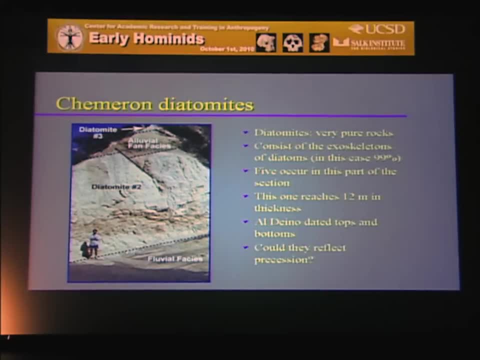 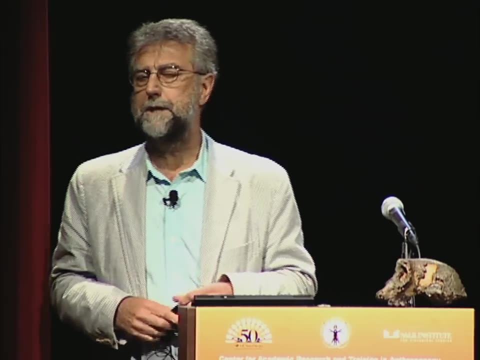 So we knew exactly how old they were And we thought: could these things reflect precession? Well, what is precession? Some of you probably know what precession is better than I do, And many of you will have heard of Milankovitch cycles. 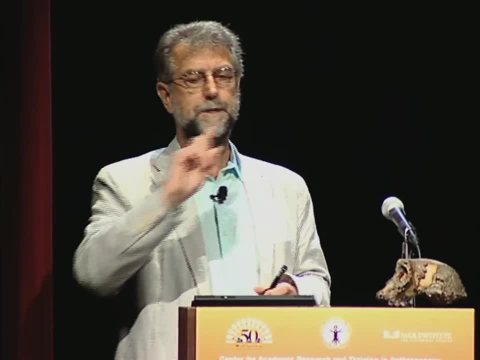 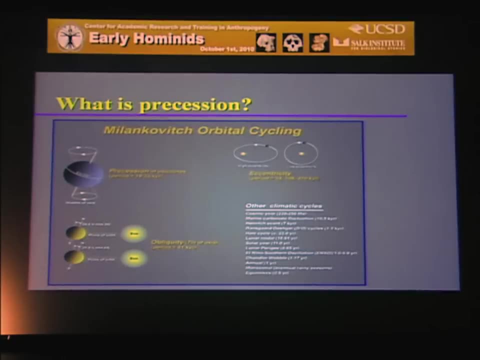 And they're all to do with the way that the Earth goes around the sun and how it wobbles, Because it wobbles in predictable and repeated ways, And precession is one of the Milankovitch cycles, which involves the wobble of the axis of the Earth. 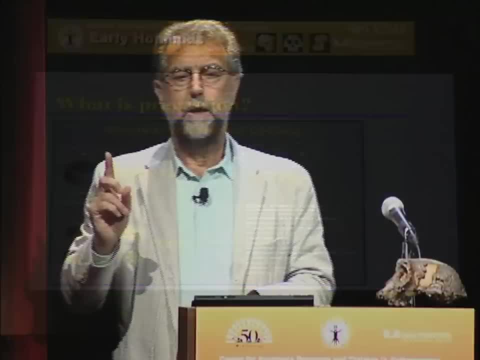 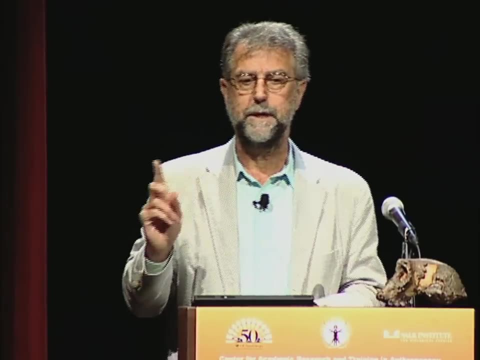 And it wobbles in a gentle way as it moves around in a repeated periodicity of 23,000 years. So every 23,000 years it goes through this same cycle. Now, another one we might mention is eccentricity over here, which is extremely simple. 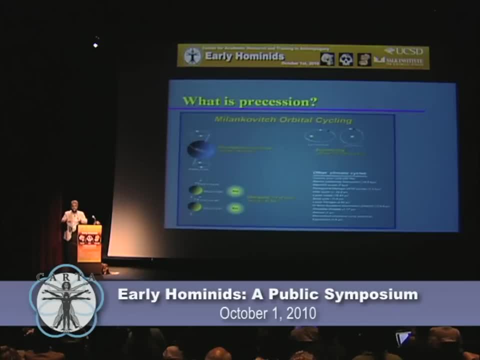 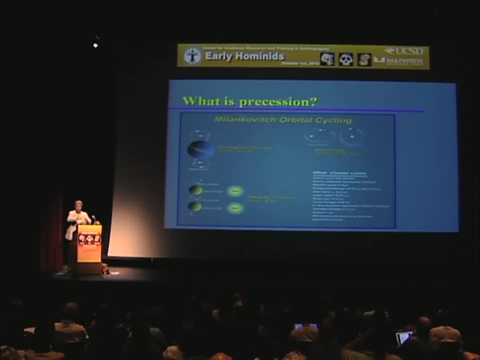 That's just that the orbit of the Earth around the sun is sometimes almost a perfect circle, And at other times it's distended a little bit, so it's more oblate and is more of an oval. Now, both of these things as far as we're concerned. 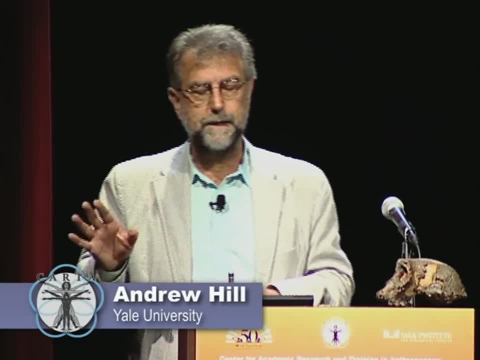 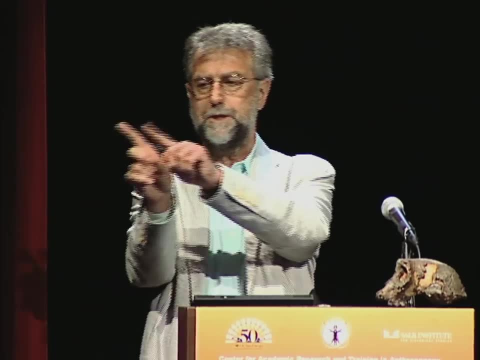 what they do is control the amount of sunlight that's hitting different parts of the Earth at different times. That's all you have to know about this, Because you know if the axis is wobbling, it's changing the bit of the Earth that's closest to the sun. 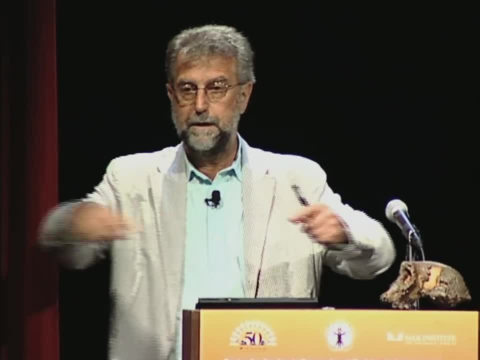 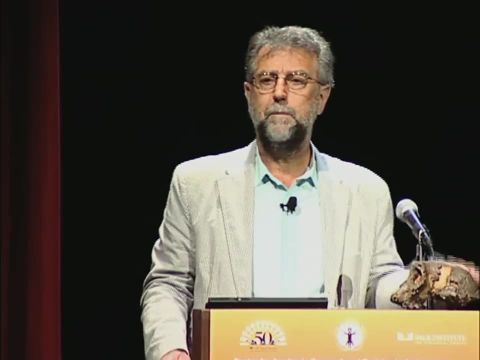 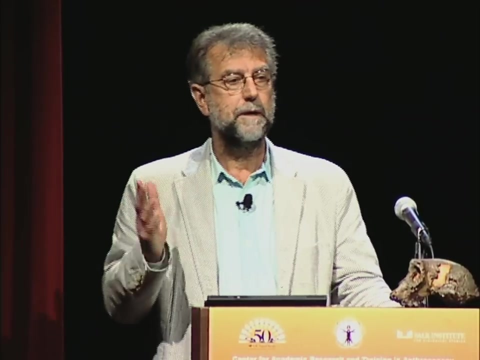 If the orbit is oval, then sometimes the Earth is farther away from the sun than it is at other times. Astronomically, these motions are extremely well understood. Well, I was going to say I can calculate. I can't calculate, but astronomers can calculate. 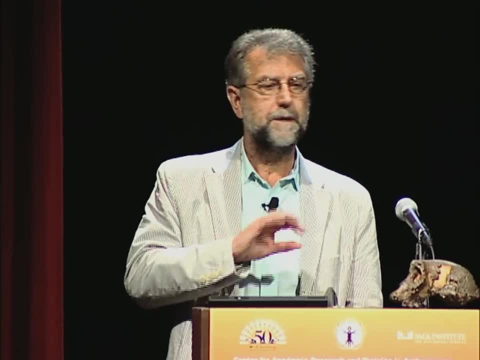 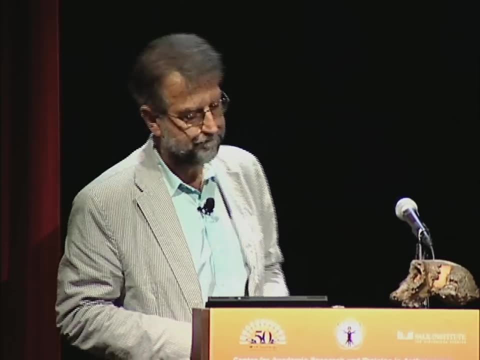 the amount of sunlight hitting the Earth at any place on Earth at any time in the past. It's a relatively simple calculation by the standards of most physics And you can get on some web page and download this and find out how much sunlight's hitting. 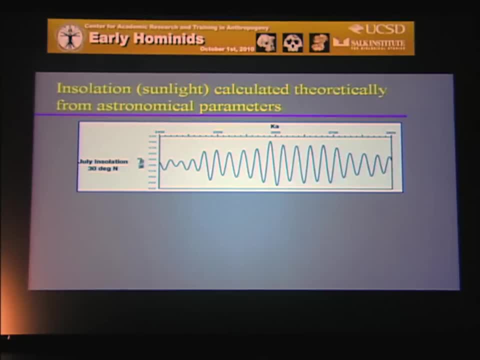 And that's what's going on here. It's called insulation. It's just the amount of sunlight, And what we've got here is the amount of sunlight hitting at 30 degrees north in Africa in July between 2.4 million years and 2.8 million years. 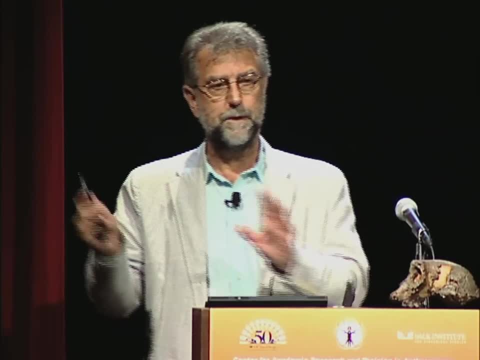 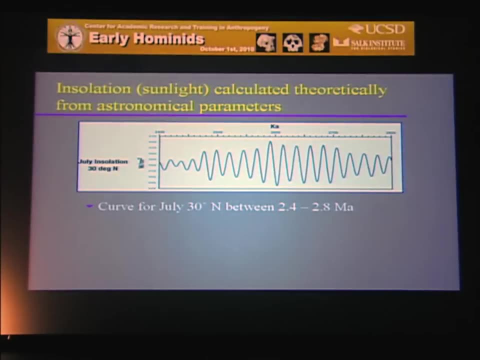 I know I'm out of the time frame, but I'm going to justify myself in a minute, I hope. And so this is the pattern: that you have These individual peaks, and that means a lot of sun when it's up there and then less. 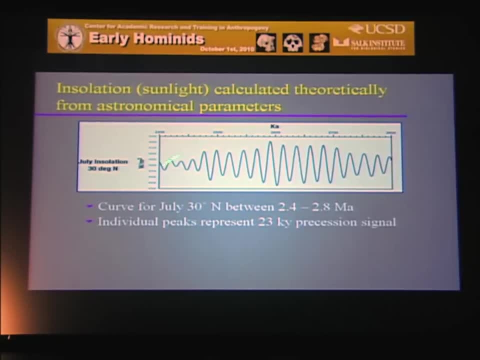 So it alternates, but gradually you have more and more sunlight over this period. These individual peaks are precession. That's just due to the wobble of the axis. The reason that it builds up to really high amounts of sunlight up here is because 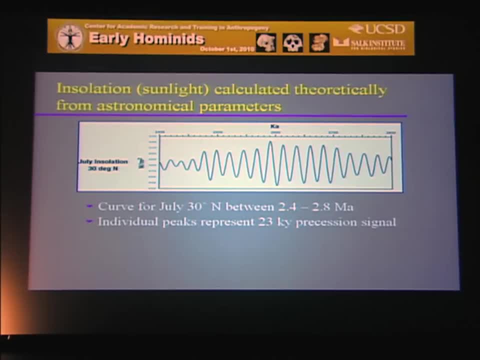 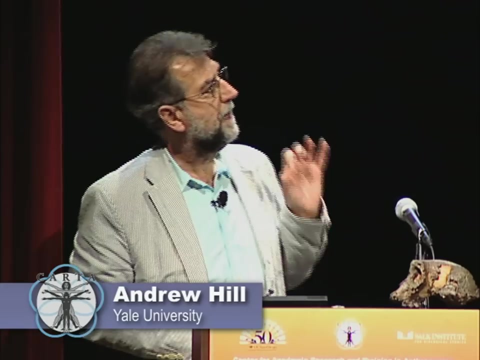 uh, eccentricity is going, is kicking in at the same time and is boosting the amount of sunlight that happens there. So you have it gradually building up and gradually dying down like that. So basically, what we thought here was then: how does our independently dated diatomites 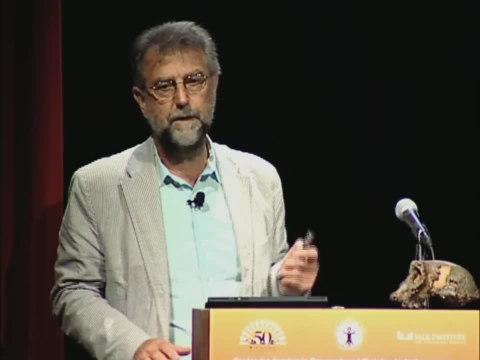 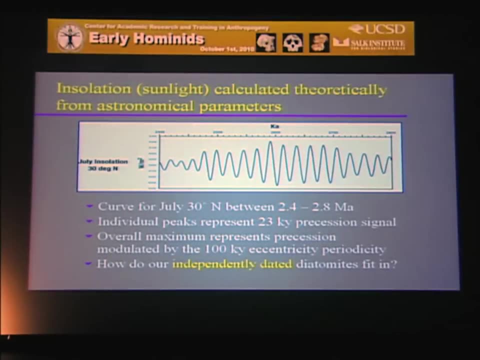 these that indicate these enormous lakes? how do they fit on this? Is it just random? Are they just some random lakes? we have And we've got the dates, independently from Aldano, having done work on radiometric dating. Well, they fit like that. 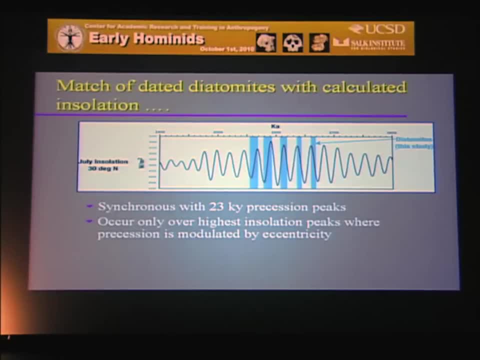 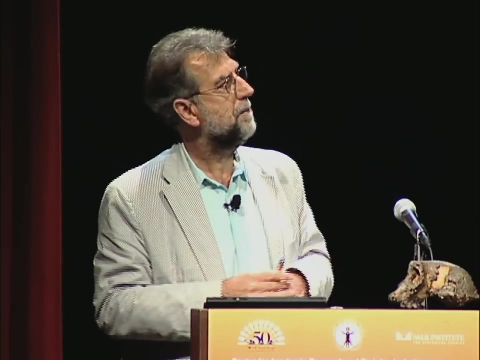 And I just couldn't believe this when this came back, because it's so perfect. You only have these lakes where you've got the highest amounts of sunlight and, in this case, where this precession signal is modulated by these eccentricity signals. So when you have really high amounts of sunlight, 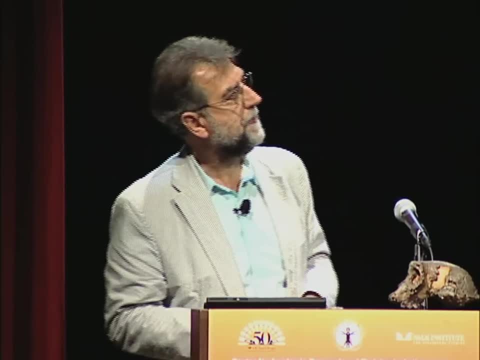 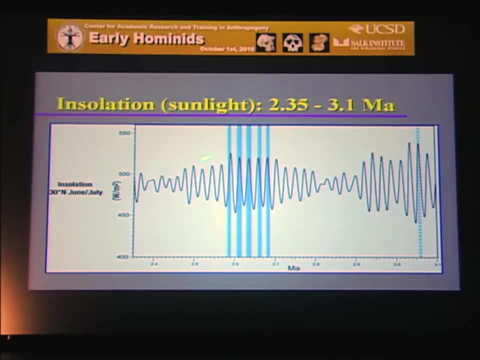 you have these massive lakes. This is a sort of more detailed picture showing this little package I've been talking about, with the diatomites on it right at the peaks of the high sunlight periods every 23,000 years, And then it's extended down here to 3.1 million years. 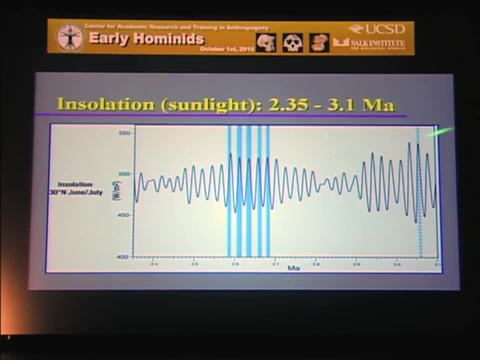 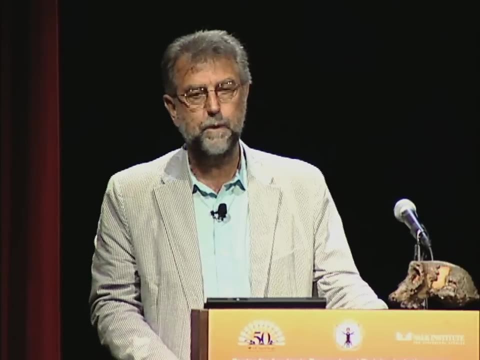 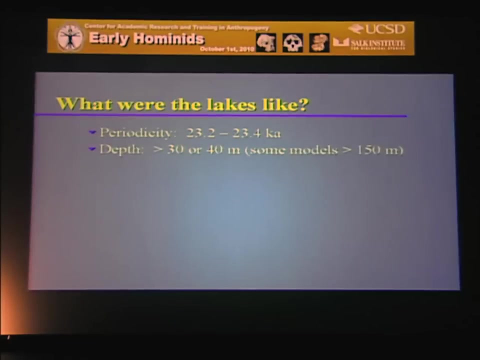 and you can see. also, we found a diatomite there that fits exactly on top of one of these peaks. So what were these lakes like? Well, they occur every 23,000 years. At certain times, when eccentricity is favorable, The depth we can work out. 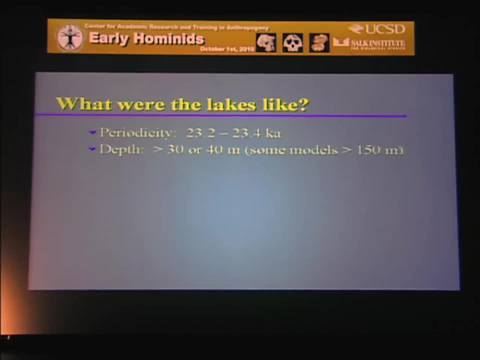 a minimum of 30 or 40 meters, and some models have suggested, quite plausibly, that they may be 150 meters deep. So these are very large lakes. The area they extend in is several hundred kilometers and, as I'll show in a minute, 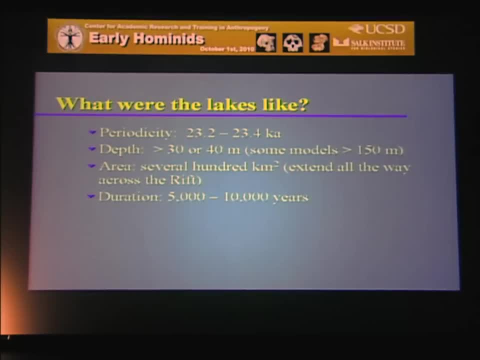 they extend all the way across the Rift Valley. They last about 5,000 to 10,000 years, And then they dry out completely, at least in the sides of them, and between these cycles, And they're driven by these astronomical factors but mediated through the monsoon system. 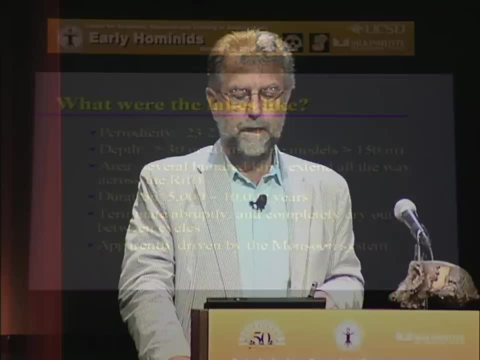 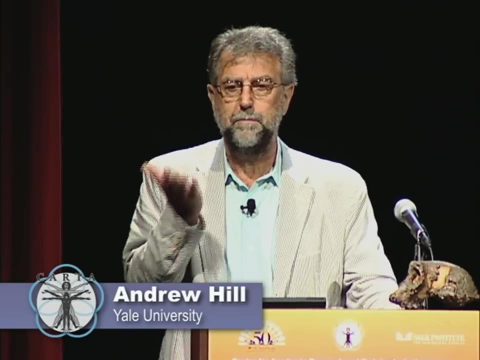 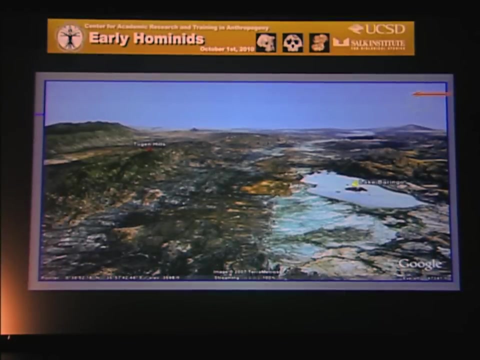 which affects Eastern Africa. I have a graduate student, Emily Goebel, who is very good with remote sensing and GIS, and so I suggested that we fill up the rift to 30 or 40 meters and 150 meters and see what happens. And so here's the view of the rift again. 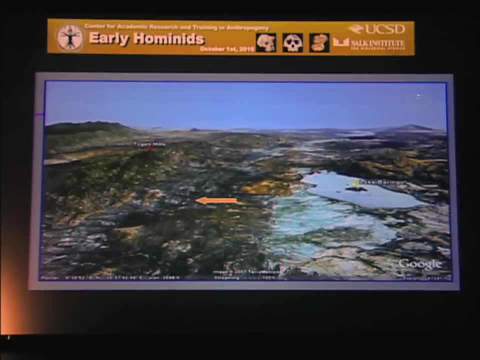 And this is where the diatomites actually occur today. And so we filled up the Rift Valley to 40 meters and then to 150 meters to see where it went, And notice the Tugan Hills here We're tilting up now into a map. 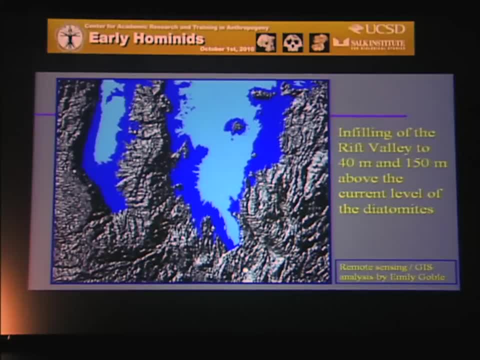 And there's the Tugan Hills going along the floor of the rift. The light color is 40 meters, The dark is 150. And in either case they more or less this lake goes all the way across the Rift Valley And that's an amazingly large lake. 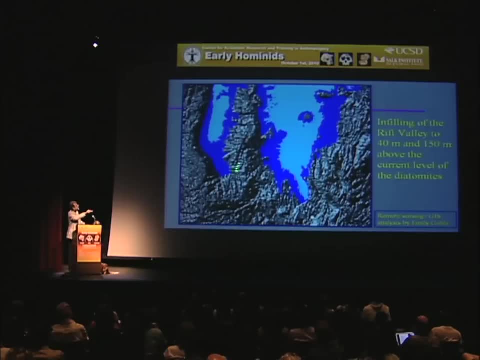 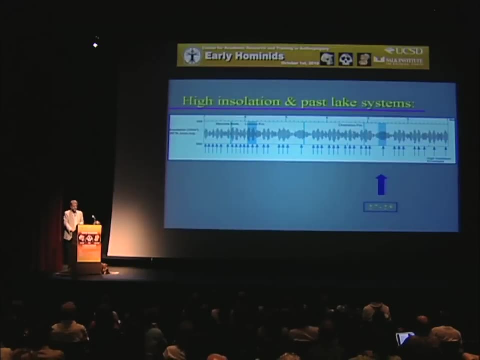 This is 60 kilometers across. The Rift Valley is an enormous structure. We know that the Tugan Hills weren't there at the time. It was a continuous lake all the way across. Now, how does this relate to the earliest hominins? 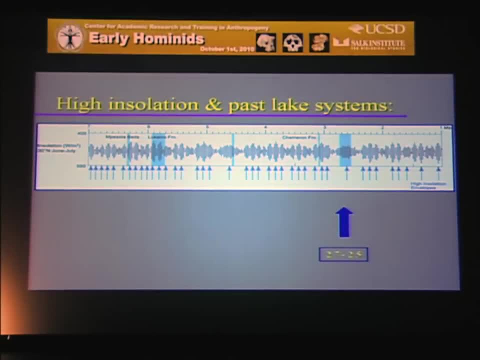 Well, I believe in this way, This is not as confusing as it might appear. All I've done here is take the insulation curve, the sunlight curve, as calculated by astronomers, and extended it from whatever I'm at here, zero one million years. 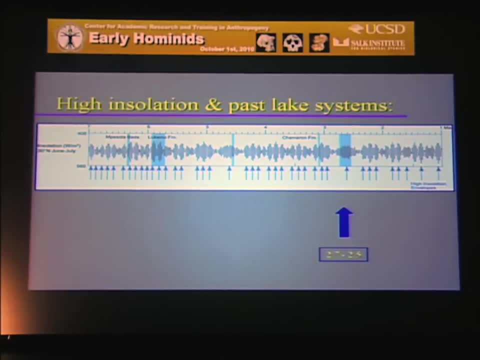 back to seven million years, to around the origin of hominins. here- And you can see there's a number of these little peaks occur every now and again where precession is kicked up by eccentricity. This is the lot we've been working on in detail. 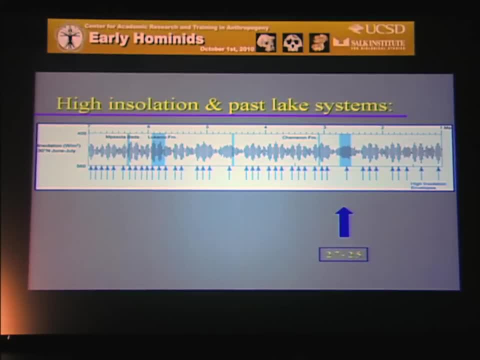 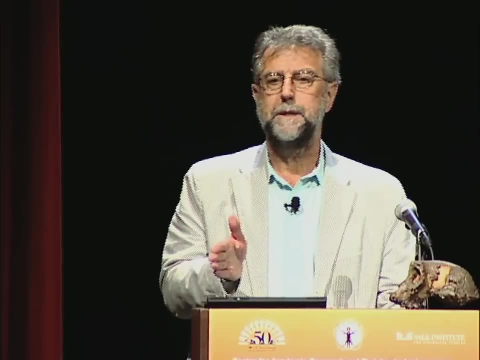 over the last few years that go from 2.7 to 2.5. And so it's not relevant to these things. But in the last season we went back in time and tried to find diatomites that might match with these earlier little peaks. 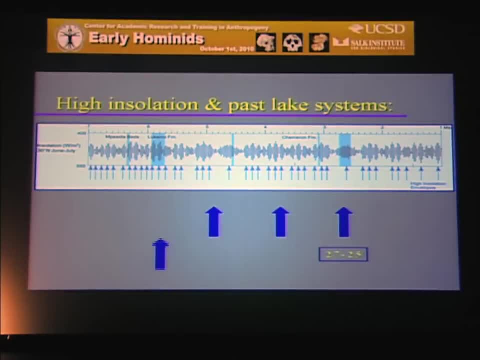 And so far we've found them there and here and here, And the dates were just done a couple of weeks ago, so a preliminary One is 3.8 to 3.7 million, one 4.9 to 4.8,. 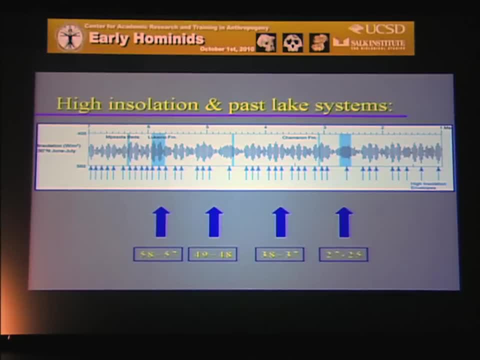 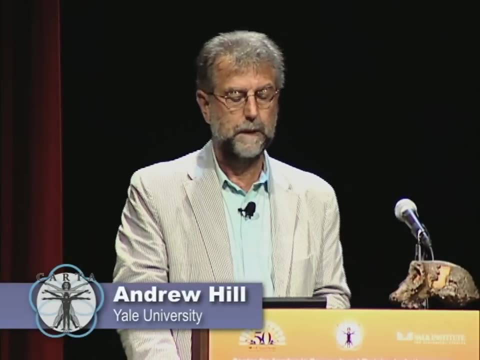 and the other 5.8 to 5.7.. And these will continue into the past as well. All of these are getting into the area where it might matter for human evolution, for early human evolution. Now the reason I think this is perhaps important. 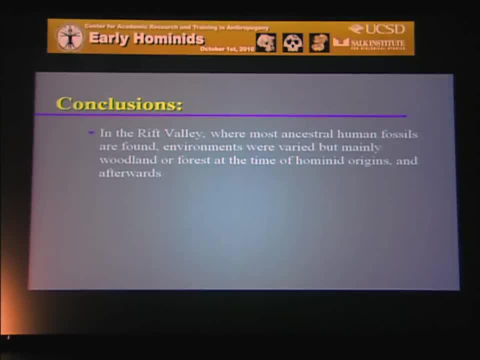 and these are the conclusions- is that where most of the fossils are actually found, the environments were clearly varied and patchy, which may be important in itself for our evolution, but they were mainly woodland or forest at the time of hominid origins. 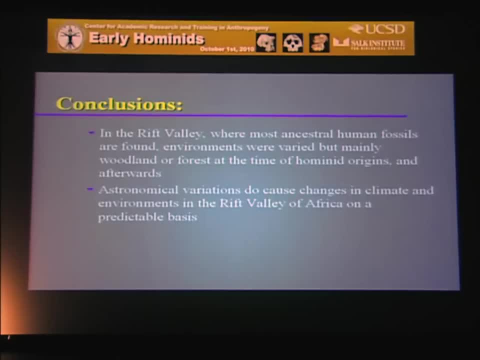 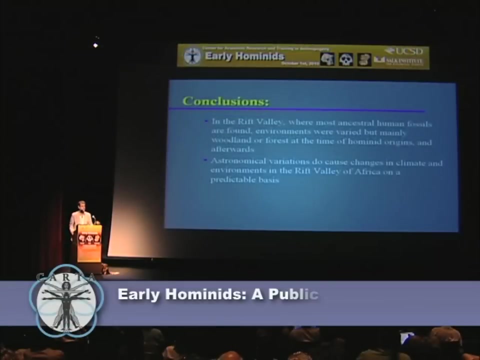 and for a good length of time to be found afterwards. The other thing is that these astronomical variations actually do cause remarkable changes in climate and environments in the Rift Valley of Africa on a predictable basis, And I'd argued against this for years. I thought this was highly unlikely. 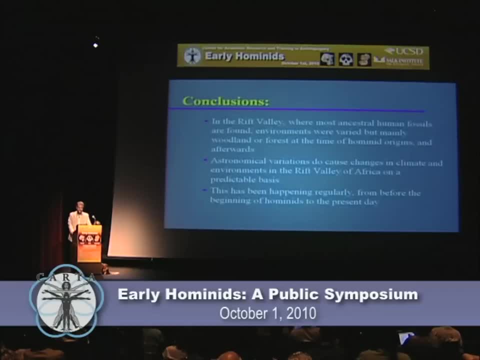 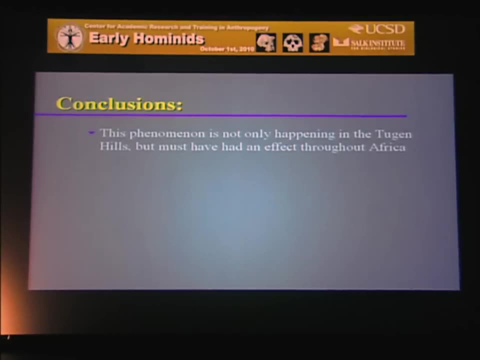 but it's quite clear that it's true And it's been happening regularly from before the beginning of hominids to the present day. It's not only happening in the Tugan Hills. This is not something that's just about my expedition. 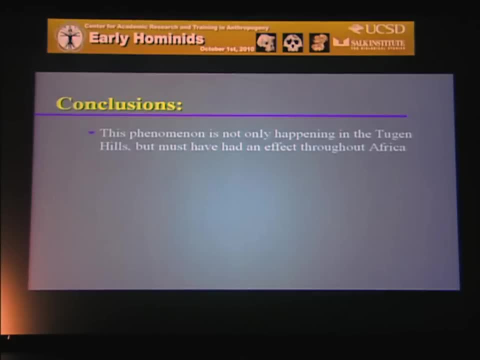 But since it's caused by astronomical variations, which we understand pretty well, it must have had some effect all the way through Africa. And you're not always going to get lakes. You need a situation where a lake basin can be and form. You don't have this happening, say. 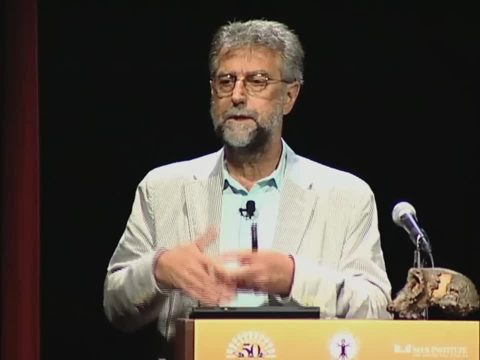 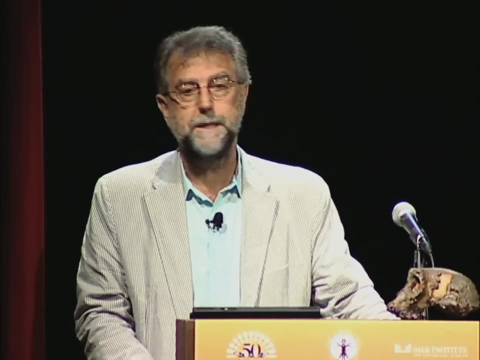 in the Hadar, for example, at 2.5 million years, because it's not a structure that would have a lake basin But it will have some strong climatic effects there, just as much as it does in the Tugan Hills. 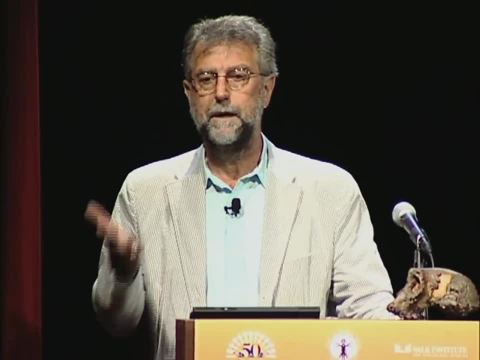 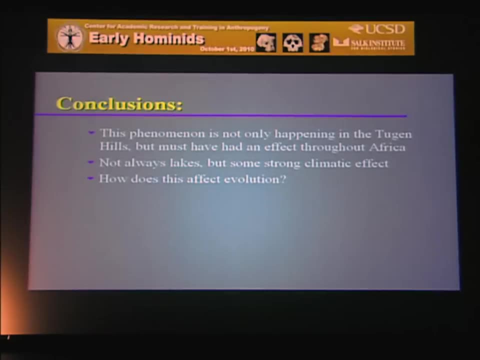 The lakes are simply a symbol and a sign that some really strong environmental short-term change is taking place. How does it affect evolution? Well, it's hard to be specific And I'm certainly not saying, OK, we've got a lake. 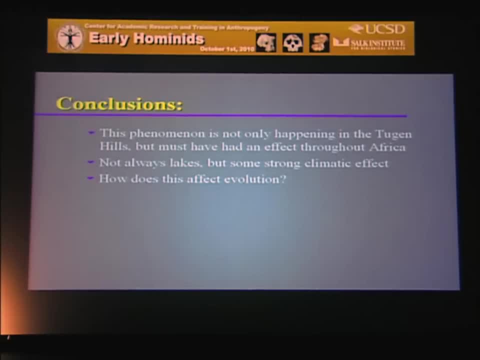 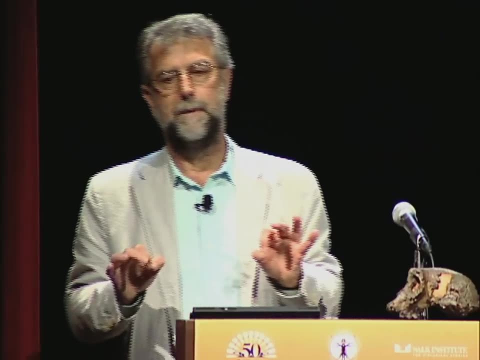 and either the hominids become extinct and have to come from somewhere else, or they get up on their back legs so they don't get their hands wet or anything like this, But what's going to happen is that it's going to cause the breakup. 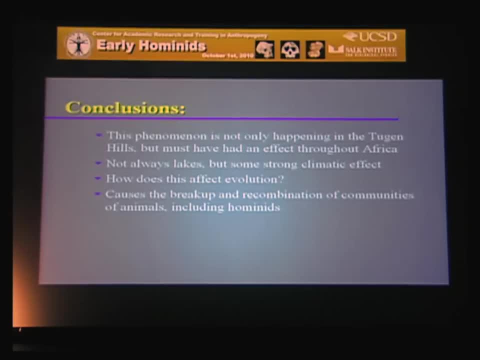 of communities to which they belong, And it will then, after a few thousand years, which is a relatively short time scale, they'll come back together again and recombine, but they'll do it in different ways And you'll have a kind of 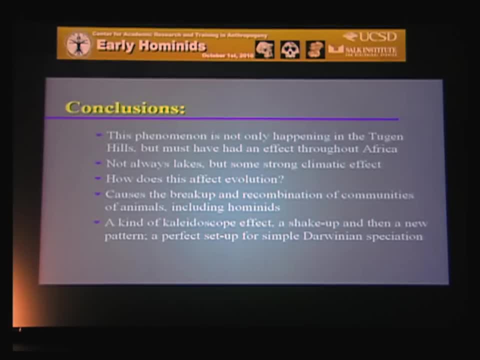 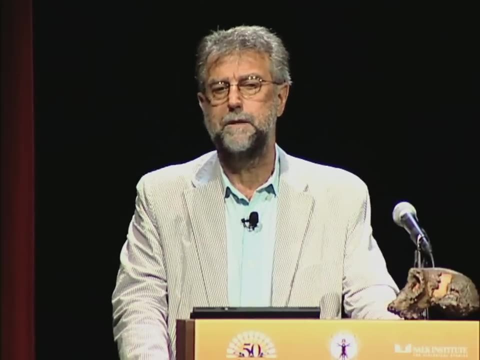 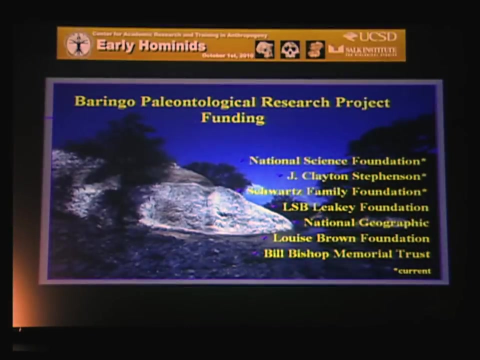 kaleidoscope effect, a shake-up of animal communities and then, within eight, ten thousand years, re-coalescing into another pattern. And this is a perfect example of a perfect set-up for relatively simple Darwinian speciation, These diatomites that you can see here: 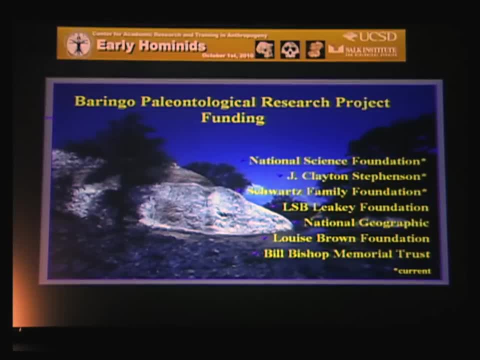 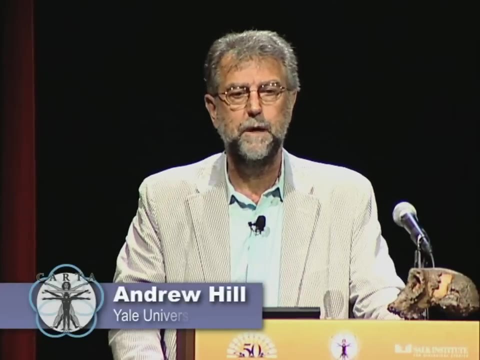 this being one of them, are also incredibly good archives of all kinds of other climatic information that we believe we're going to be able to get temperatures on a yearly basis back in time, Even at, say, seven million years. we'll be able to have a record. 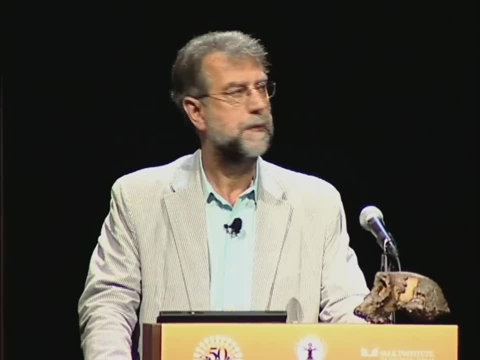 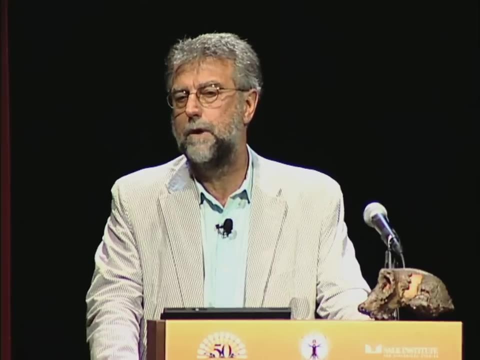 of annual temperatures and we'll be able to see what's happening over these periods, And I think they're a really remarkable archive that I hope will cast some light upon the origin of hominids and also on their subsequent evolution. These are some of the people